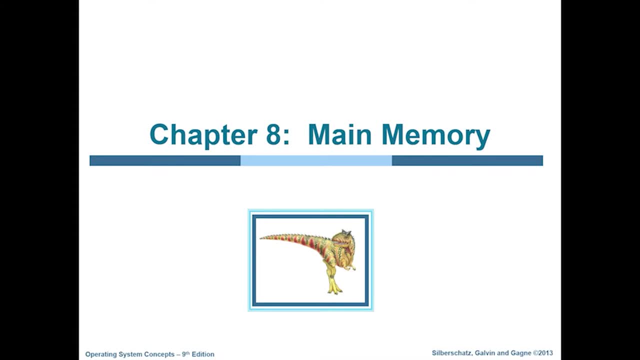 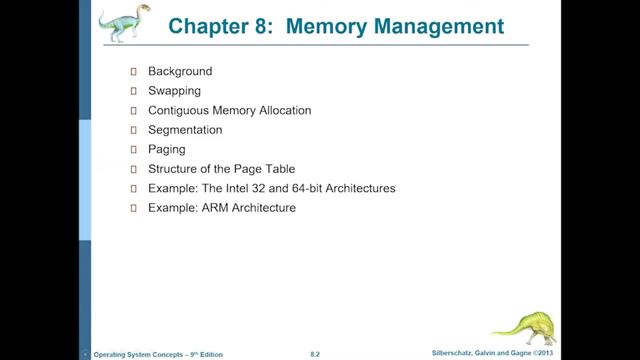 they are protected from each other and various things like contiguous elements, communication, performance and efficiency concerns are taken into account while allocating memory space to those processes. We will look at how these things can be handled in operating systems in this lecture. Let's proceed. So first we will look at some background and 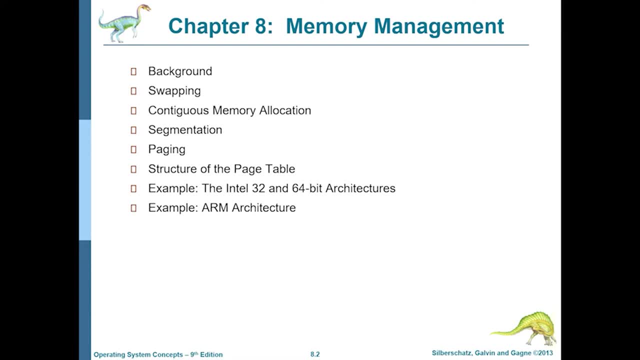 then we will look at what swapping is. Swapping happens when the system runs out of memory and you need to swap one process for another, because you cannot swap the other process. You cannot keep so many processes in memory at the same time. Then we will look at contiguous. 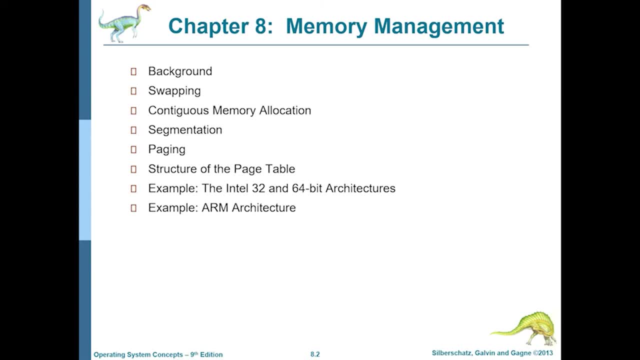 memory allocation, because if memory is not allocated contiguously, then programs will find it very difficult to run. So the operating system has to do special things, along with the help of hardware, to be able to allocate memory to processes contiguously. We will 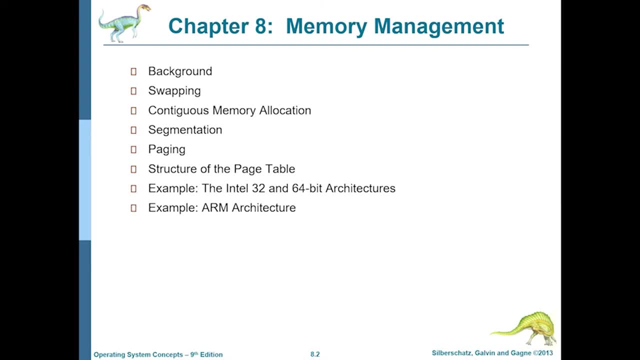 look at two famous mechanisms using which operating systems can run out of memory. One is called segmentation and paging. We will look at more details about how page tables are laid out. In the end, we will also talk about how the Intel 32 and 64-bit architectures. 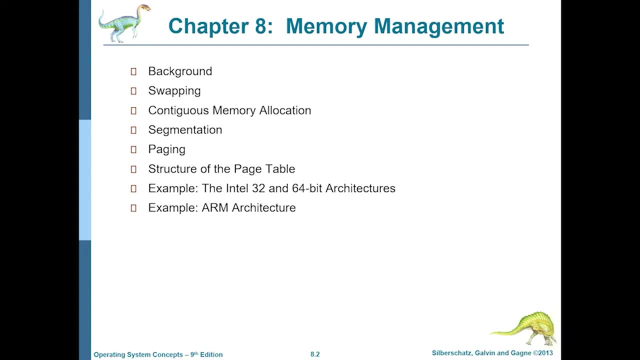 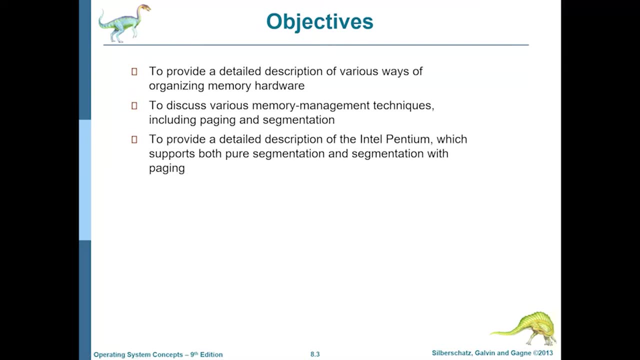 handle segmentation and paging. We will also take a brief look at the ARM architecture and how it does paging. The objectives of this chapter are to provide a detailed description of how memory hardware organizes memory. We will look at various memory management techniques, like paging. 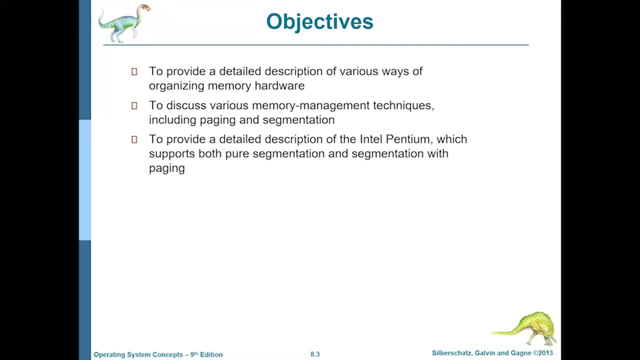 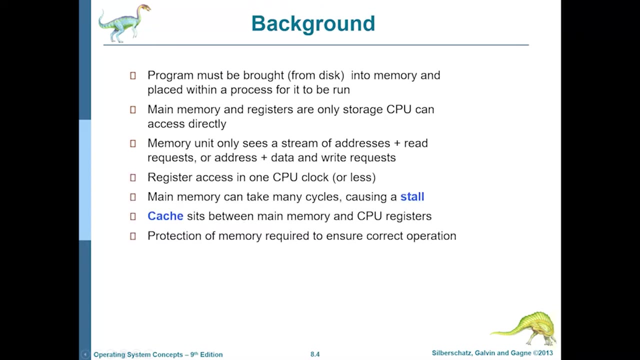 and segmentation. We will also look at a detailed description of the Intel Pentium way of doing segmentation and paging, And we will also look at how ARM does these things. briefly, Let's begin with some background. Programs must be brought from disk into memory, And 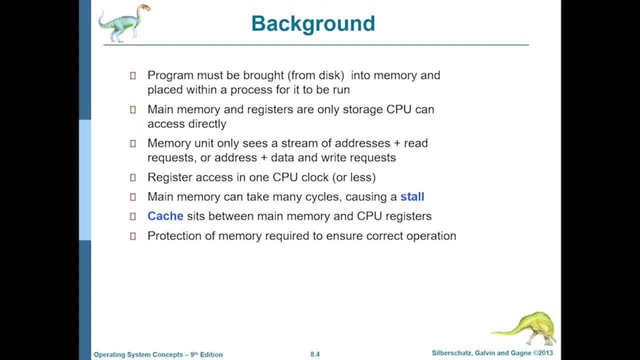 a process needs to be created from that memory, and then the process gets scheduled on CPUs and they run. So programs usually keep lying on hard disks or other storage media. They do not remain in memory from the beginning. It's only when you want to execute them will. 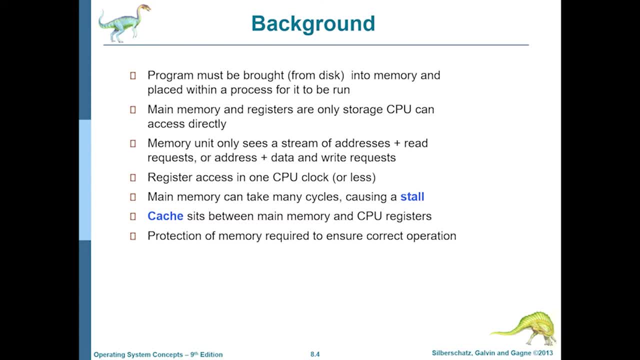 they be brought from the disk and put into memory And they will get scheduled as a process on a CPU and they will run. CPU can only access the main memory and its registers directly. It cannot access the hard disk directly. There is something called a memory unit which sits tightly between the CPU and the RAM, the main. 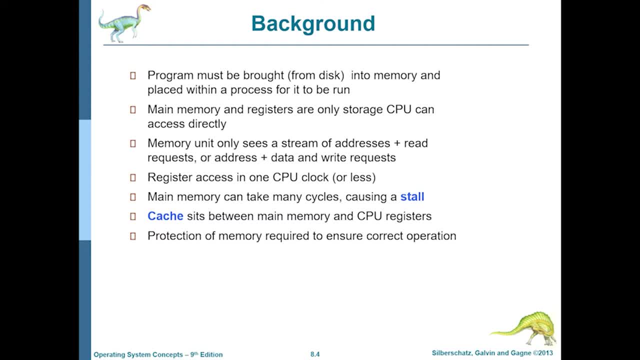 memory And its job is to take an address and whether if it is read or write, it reads data from that memory address or it writes data to the memory address. that's its only job. it does not worry about how the memory addresses are created if you have done architecture before. 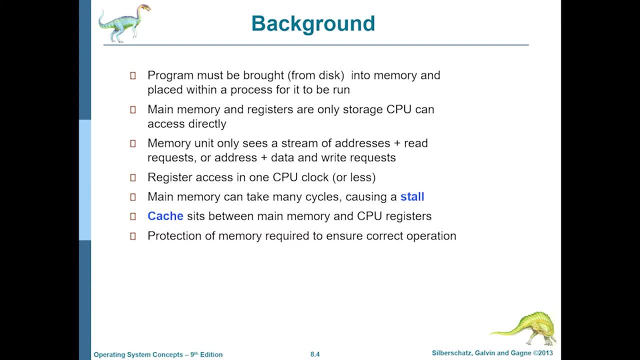 you will know that there are different ways of addressing. the memory address can come from a register. they can come indirectly from another memory location. they can be the sum of a base register and an index register. they can be literally given in the program. so there are various ways in which addressing can be done. it is none of the business of the memory unit. 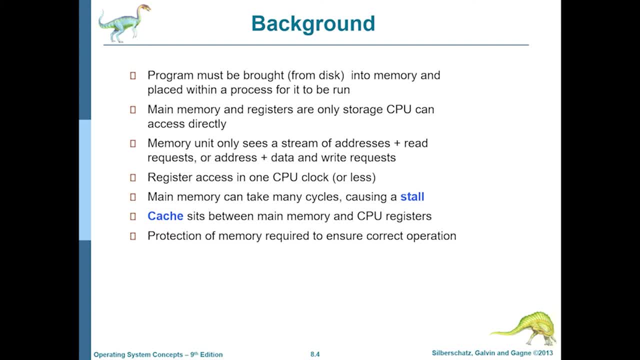 to know how the addresses have been generated. it only needs an address and whether to read or write from it, and that's its only job. when registers are accessed by the cpu, then that can be done in a very, very speedy manner. usually within the same clock cycle the cpu can access one or more registers and work on them. 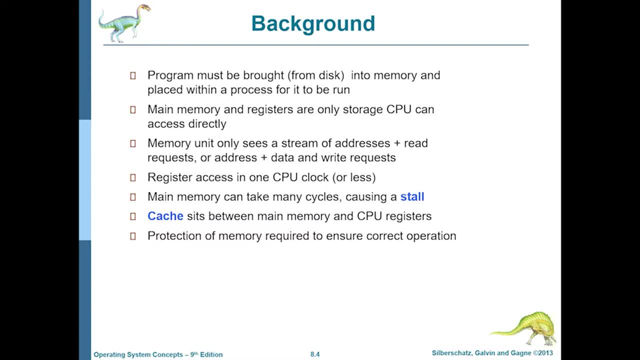 but when it needs something from the main memory, that cannot be done so fast because the address needs to go to the memory unit and the memory unit then gives it to ram the dynamic memory that you have and then that takes a very long time to retrieve or store the data and then give the 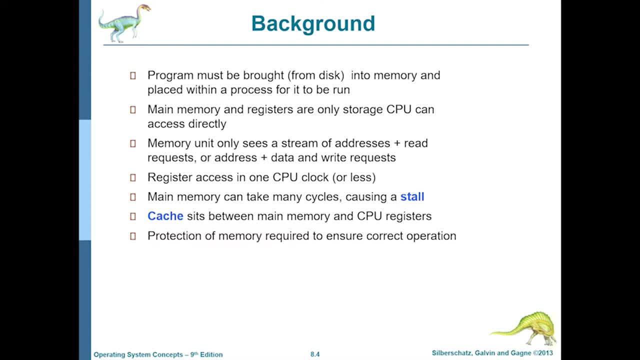 data back, or the confirmation that something has been stored, or here is the data that you want to be stored and read. that can take a lot of time in comparison with the speed with which cpus run. so the cpus usually stall. they don't do anything, they just keep waiting for the data to arrive, or the data. 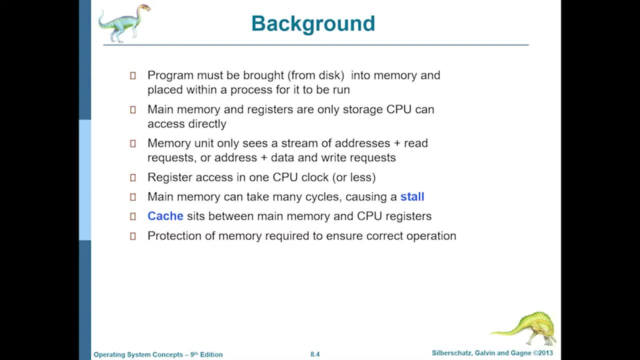 to be written. that is the reason we put a cache in between the cpu and memory, the main memory. the cache runs very fast. well, the cache does not run as fast as registers, but it runs pretty fast, way faster than ram can ever operate. and when the cpu needs something it first looks into the cache. if it finds it, then it's good. 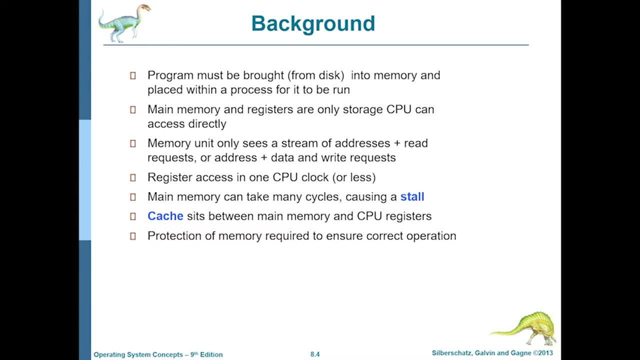 otherwise it has to go to the main memory, get the data, put it into the cache and then use the data next time. if it needs the same data, it will directly go to the cache and use it. if more than one processes are there in the system and they have their own memory areas, then we have to make. 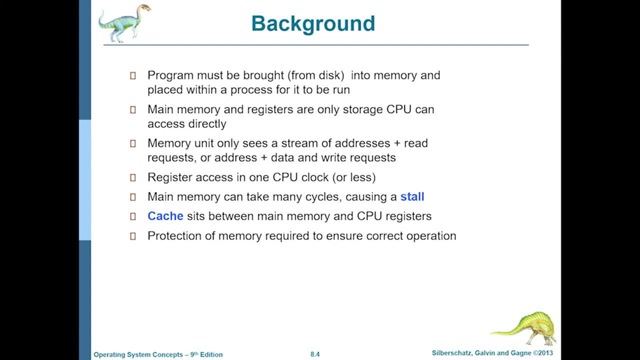 sure that they don't keep interfering in each other's business. if i am a process, then i should only deal within the boundaries of my memory. i should not try to access the memory areas of other processes. also, the operating system needs to protect its own memory area because if other processes can trample into the memory areas of the operating system, 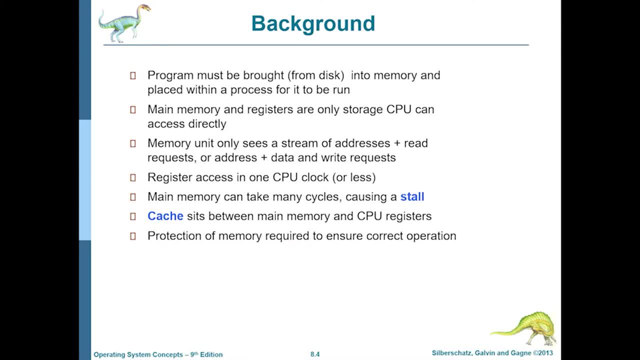 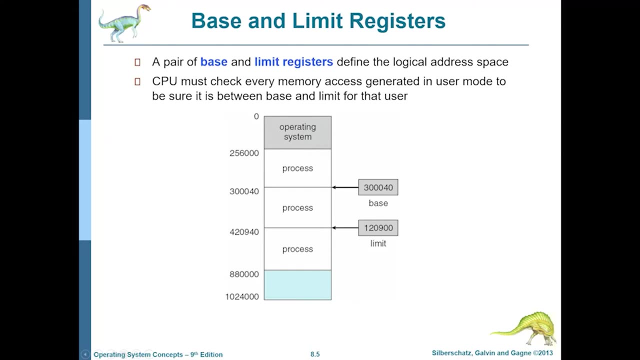 then they can corrupt that memory area, maliciously or otherwise, or viruses can get into that, and then the whole system is compromised and we cannot let that happen. so let's look at a very simple way in which that protection can be achieved. so that kind of protection can be achieved by using the concept of base and limit registers. 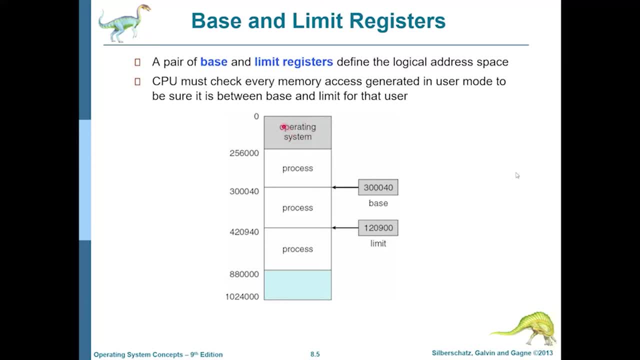 so here you can see, the operating system has its own area. it usually uses the lower memory addresses because zero is right here and the memory is increasing in this direction. the operating system is sitting and the memory is increasing in this direction. the operating system is sitting and the 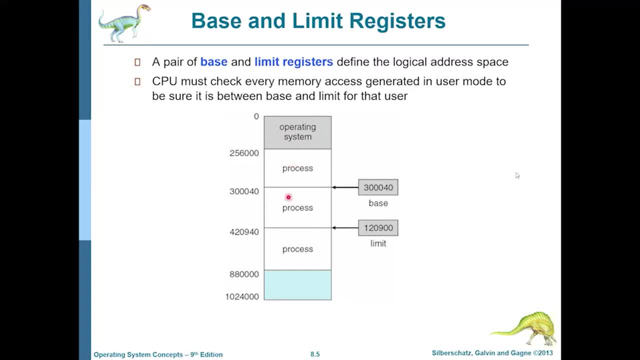 right here in its area. and then here is one process, here is another and here is yet another process. each process begins at a certain memory location and that is given by a base register, and there is a limit until which it can keep accessing, reading or writing memory in that area. 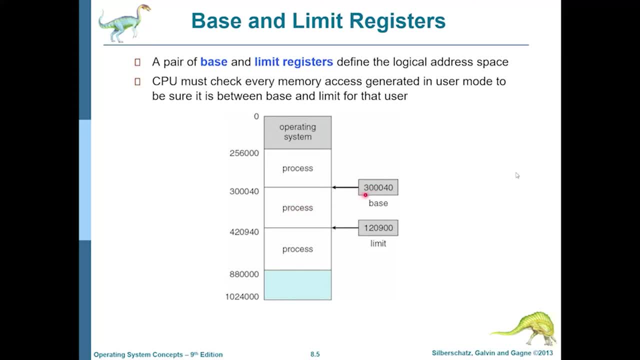 so here for this process as an example: the base is three zero zero, zero, four zero and the limit is one, two zero, nine zero zero. what does that mean? it can access this address: three zero, zero, zero, four zero. it can access all the memory addresses between this address and this address, plus the limit. 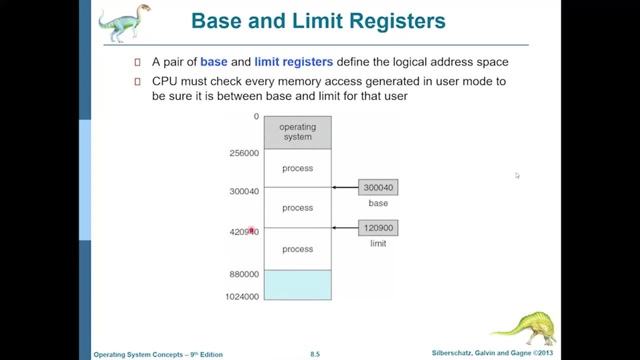 this address plus the limit is equal to four two zero nine four zero. well, this address belongs to the next process. so whatever you get by adding the base and the limit, that is exclusive. that is not included in this process. so all memory addresses, including the base but excluding the base plus the limit, this entire range, that is fair game. those are all. 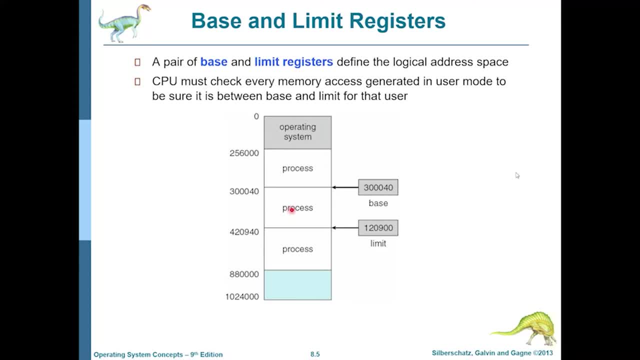 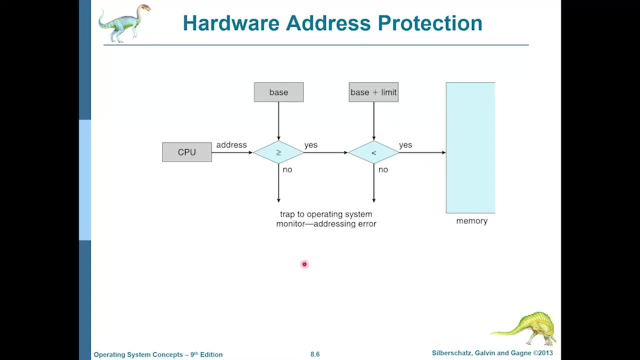 legal addresses for this process and it can only access memory read regions in that area. so this slide explains that process in a little bit more detail. so the cpu generates an address for a process. it is then checked against the base register if it is greater than or equal. 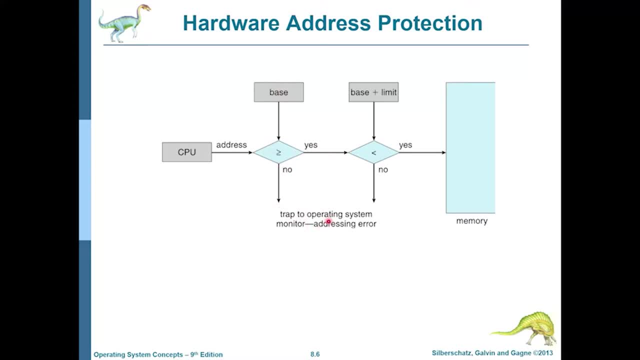 to the base, then you can proceed. otherwise a trap is generated and the operating system is asked to handle that trap. then the base plus limit is computed and if this address is less than that, as i said, the base plus limit is exclusive. that is not included in the memory region. 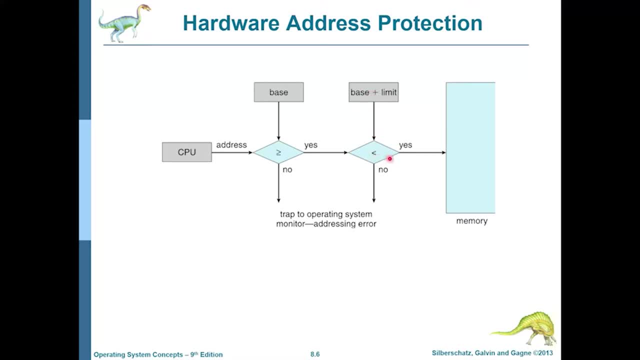 the process can access. so you have to be strictly less than that. if it is yes, then you can go ahead and access memory. otherwise, again, a trap is generated and, as i said, the base plus limit is is generated and the operating system has to handle that. This is a very rudimentary 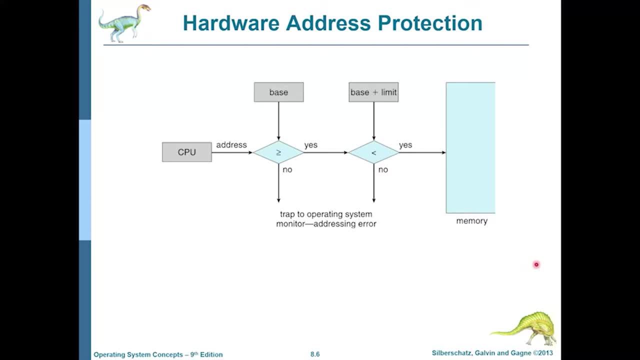 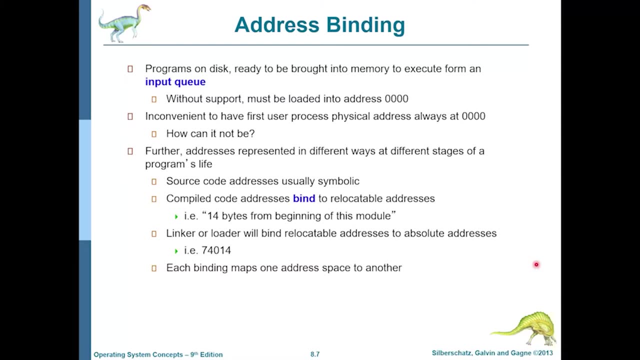 or a very basic way to handle protection. Now let's look at the concept of address binding. What is address binding? So, when you write a program, you have variables and functions, and those variables and functions need to have addresses, Otherwise how would the CPU? 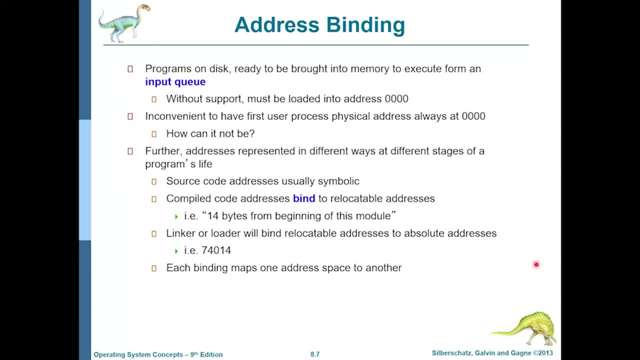 tell: go, get me the data for this variable or store this data into that variable. call this function. So addresses are very important for variables and functions and other things in a program. Now the program goes through various stages. It is first compiled and then 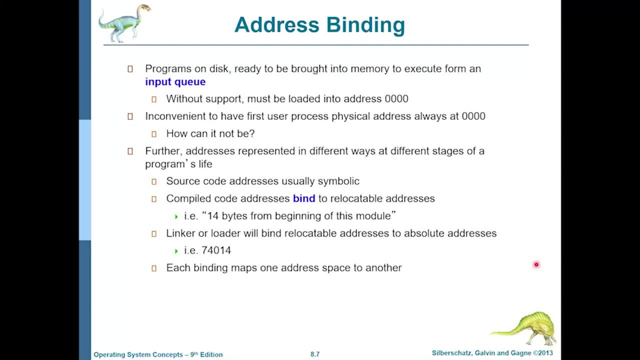 it is linked, then it is loaded into memory and then it is executed. These different stages bind different kinds of addresses to those variables and functions. So at compile time, okay, Usually relocatable addresses are bound to variables and functions. Now what is the meaning? 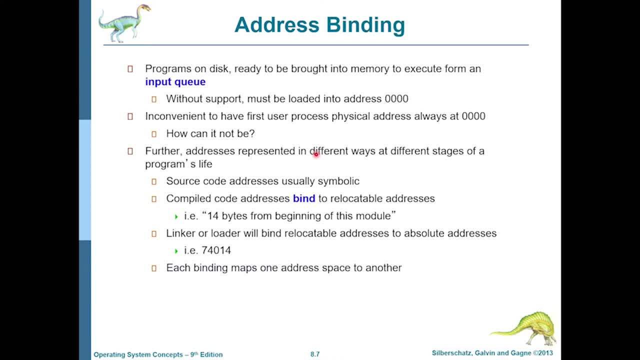 of relocatable. That means that it is not guaranteed where the program is going to end up in memory, where the program is going to begin, what is going to be the beginning address of the program, Since the compiler has no idea what that is going to be, it is going: 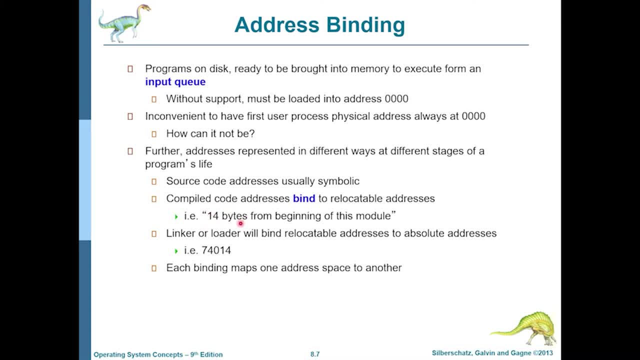 to give relative addresses. It would say: this variable is, for example, 14 bytes from the beginning of this module And at runtime, whatever the beginning of the module is going to be, this variable will get an address of 14 bytes after the beginning of that module. So it is clearly relocatable. You can relocate. 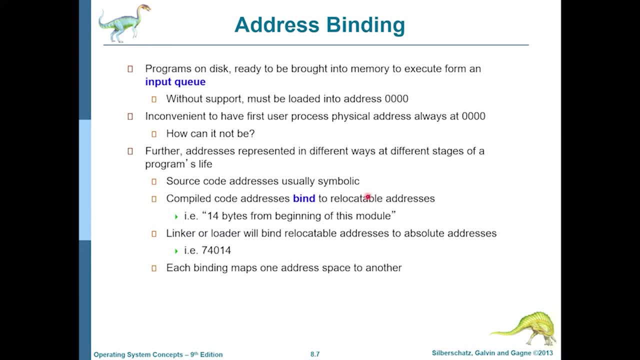 the program and all the variables and functions will get the correct addresses because the differences are given by the compiler. When you link or you load a program, then absolute addresses are given because the loader knows where it is going to load the program. what is going to be the beginning address when it is going to load the program? what is the? 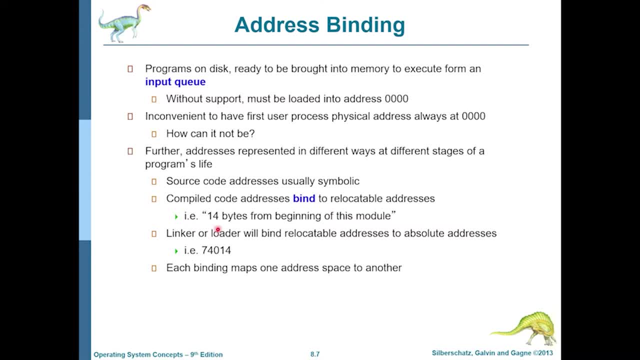 going to be the beginning of the module, So it can take these differences that the compiler has given that okay, 14 bytes from the beginning, and now the loader knows what the beginning is So it can give absolute addresses to those variables and functions. 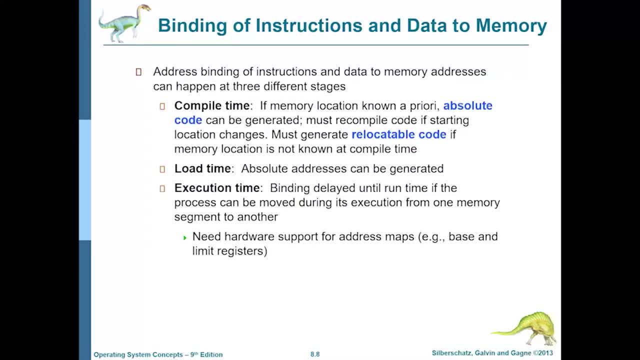 This slide talks about much of the same things that I was talking about in the slide before. At compile time, if you already know where your program is going to land in memory, then you can generate absolute code, But that is seldom the case, So the compiler must know. 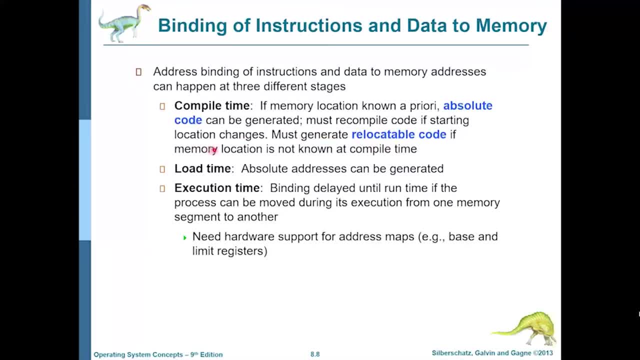 where the final location of the program is going to happen, and that the program must generate relocatable code At load time. you can generate absolute addresses, but only if you know where the program is going to land. again, just like the compiler usually does not know where the program is going to land, it must generate relocatable code if. 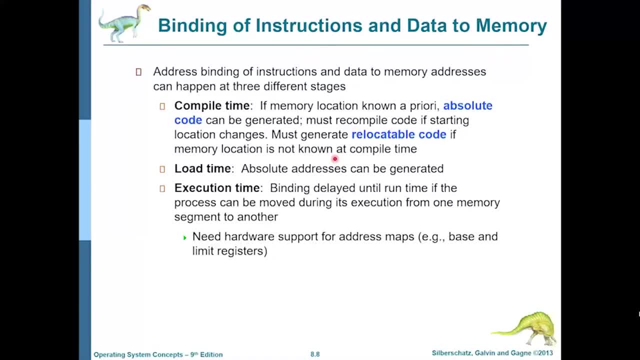 the loader also does not know what is going to happen at runtime, because the loader might put the program at one location, but she will have to find the address or not, because she does not know where the program is going to land. So this is what you are doing. You are. 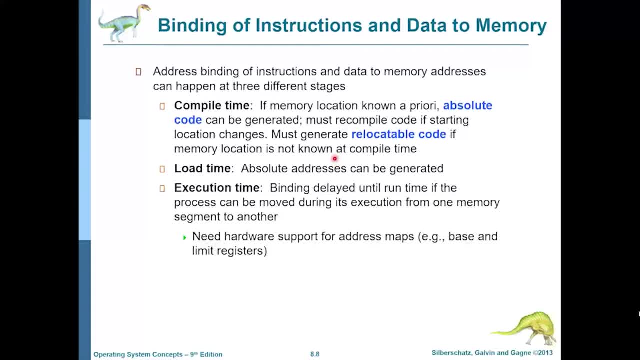 generating absolute code, operating system might try to move it around to different segments at runtime. then the final address binding job is given to execution time instead of loading time. but usually the loader knows where the final program is going to be, so the loader can generate absolute addresses. 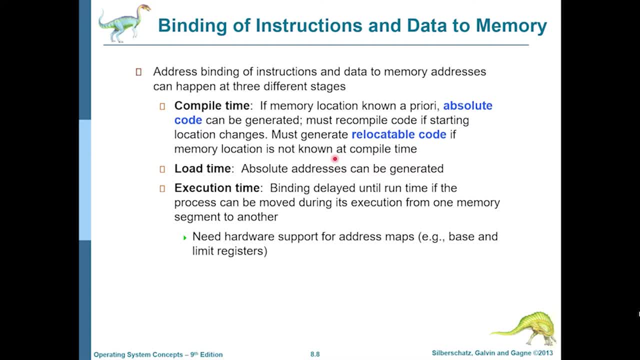 but if that is not the case, then at execution time the final addresses are generated and those are the addresses that the cpu generates and sends to the memory unit for reads and writes. once both are done, the final address binding job is shown to be free of cost. 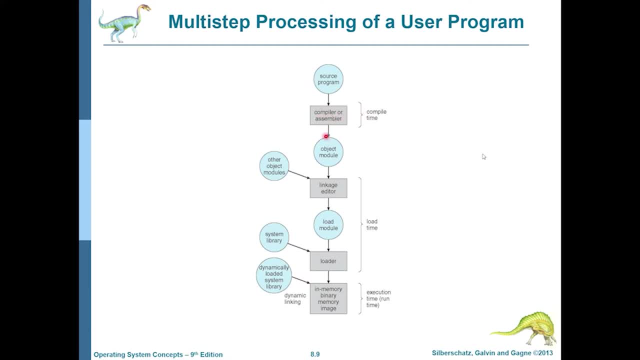 again. you can see the process very quickly. you have the source program. you use your compilers and assemblers at compile time to create object modules. then a bunch of object modules, as in your program, can be a setup, source files, assembly, source listings and whatnot. all of them will become single object modules and all of them can be. 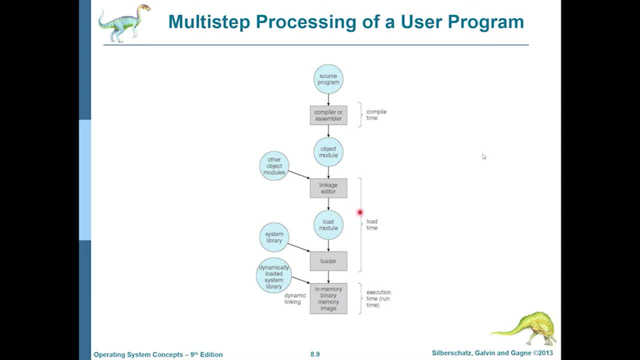 linked to create an object beings filed everywhere. so you can understand what I have just told you: executable and that executable is loaded into memory at load time and the loader when it does that, it also takes the help of system libraries, because system libraries are usually not linked. 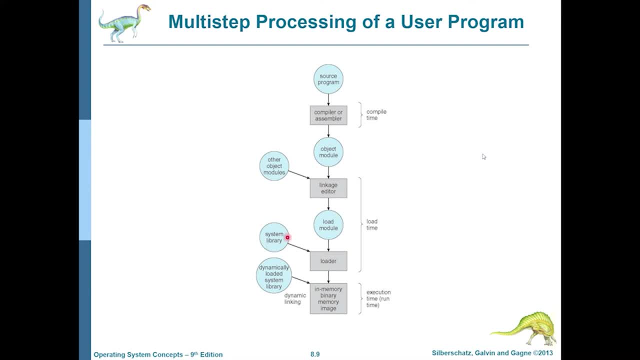 into the executable. so it is the job of the loader to also link in some functions and routines from the system library and the execution of the program begins. but there are certain functions and modules which are used so commonly and they are used by so many programs, that it does not 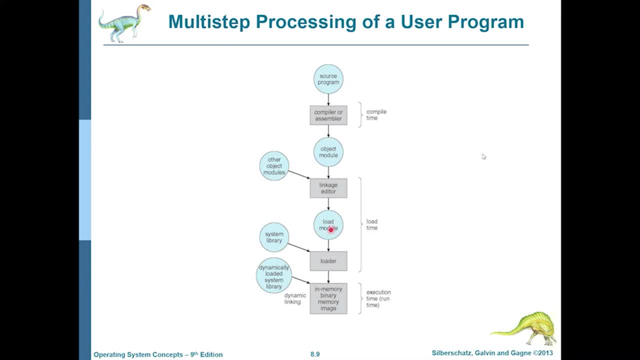 make sense to put one copy each into each of your executables. so when your executable is running in memory and if it encounters one such function, which is a common function- and the code for such functions is usually kept in dlls, dynamic loaded system libraries- then your operating system can go. 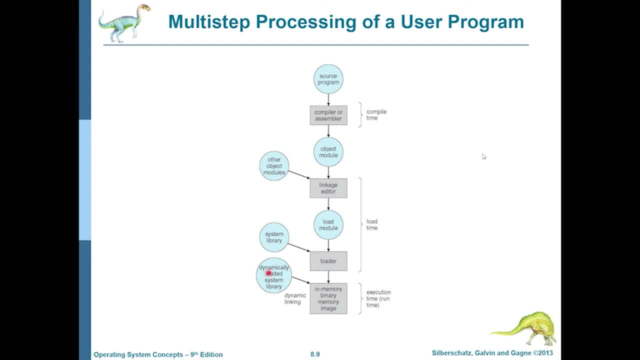 fetch the code of that function from the dll, put it in memory memory and then also patch that memory. tell your executable that, okay, you do not have the code for that function, but i have already retrieved that code from a dll and put it in memory. now you can go ahead and call that function, because its address is this: this: 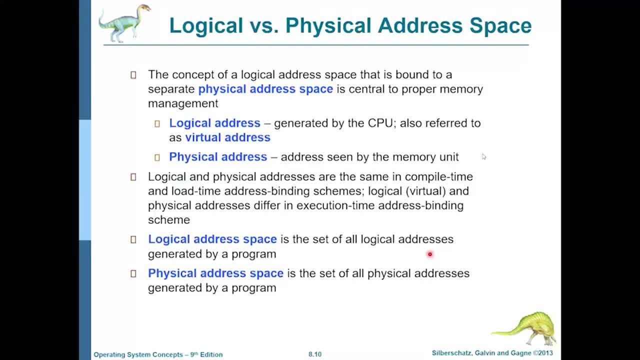 is where i have put it. now. there are two kinds of addresses: logical addresses and physical addresses. the addresses that are generated by your cpu, they are called logical or virtual addresses. the address that the memory unit sees, they are called physical addresses. there is a module in between. there is some functionality, there is some hardware that sits between the. 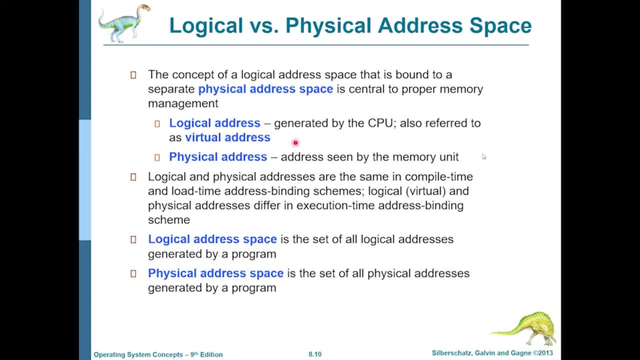 cpu and the memory unit that converts logical or virtual addresses to physical addresses. now when you are doing compilation or loading or linking, the program is not running yet and for those purposes logical and physical addresses mean the same thing. but when the program is running, the cpu is generating virtual or logical addresses, but those may not be the same addresses. that 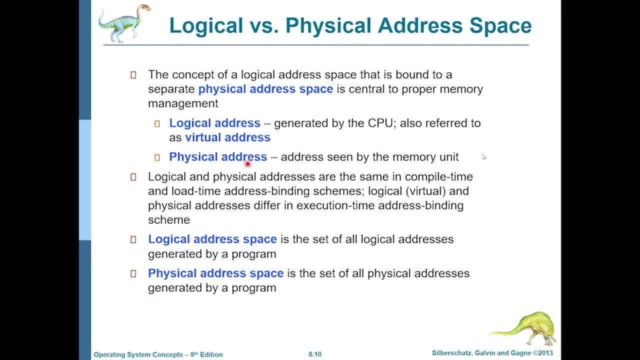 the memory unit is seeing when the program is running at runtime or execution time. the memory management unit that is sitting in between the cpu and the memory unit might be- because it does not always happen- might be converting these logical addresses to physical addresses and and, for the cases of running programs, there might be a difference between logical 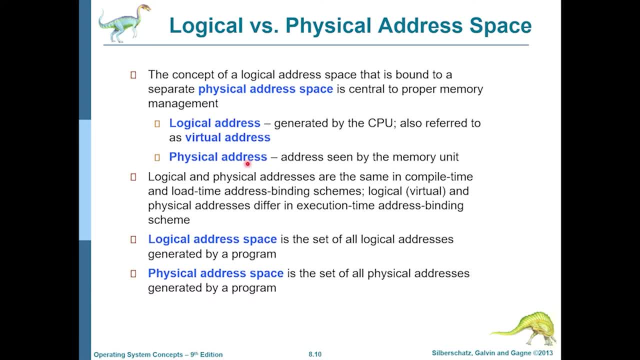 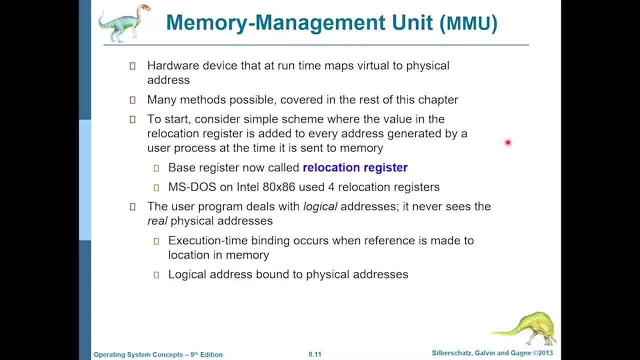 and physical addresses at the time of compilation or linking or loading, physical addresses and virtual or logical addresses mean the same thing. so i was talking about the memory management unit before and it is the unit that converts virtual addresses to physical addresses. but it is the unit that converts virtual, as in logical addresses that the cpu generates, and physical. 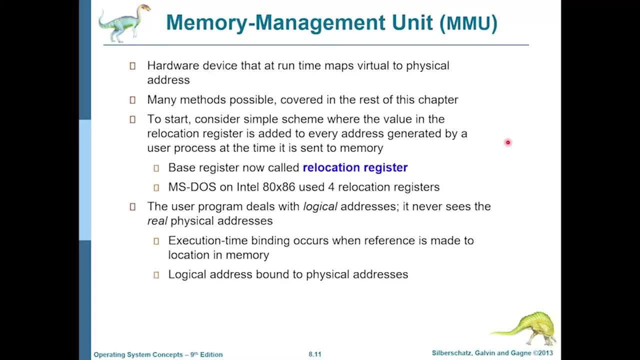 address, as in the addresses that the memory unit sees. back in the day when people used to use ms-dos on intel x86 processors, ms-dos used to make use of four relocation registers. now these relocation registers used to contain the base address of the code, the data, the stack. 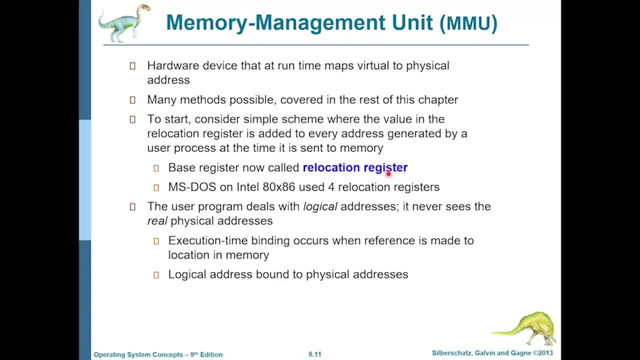 and an extra segment, right, so the code used to be in the code segment, the data for the program used to be in the data segment, the stack used to be in the stack segment and there used to be an extra segment for holding other things. and what would happen is that 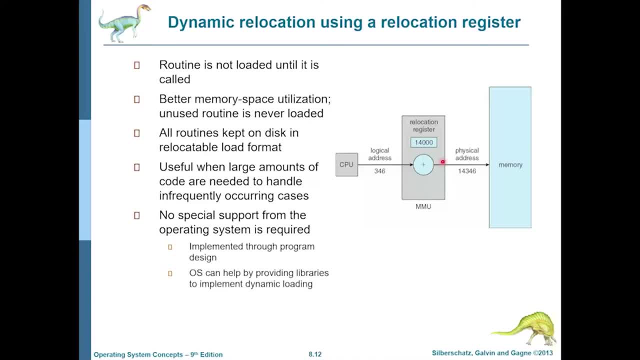 and let's look at that in the other slide- is that each of these relocation registers would have a base address and the cpu would generate a base address and the cpu would generate a logical address. the base address would get added to the logical address and a physical address would get created, and that was the job of the mmu, so the memory management. 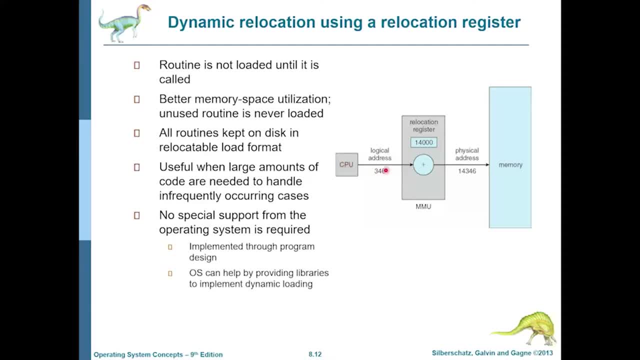 unit kind of knew that. okay, the cpu is generating a code address. i know the base address of my code segment: relocation register. i am going to take the logical address generated by the cpu. i am going to add this number and whatever number comes out, here is the physical address. 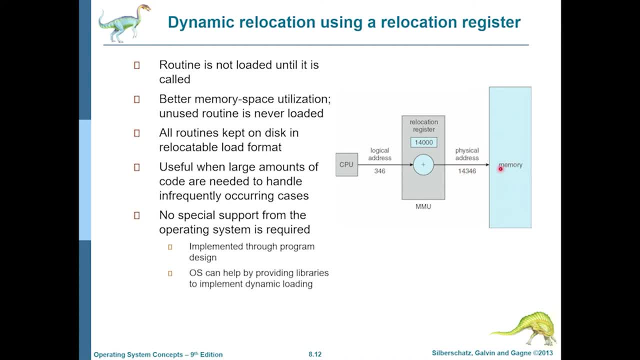 and this is what i'm going to send to the memory unit for reading or writing. so the os had very little to do with setting up the values in this registers. it was usually the programs which would do it themselves, and that is what kept these things very, very. 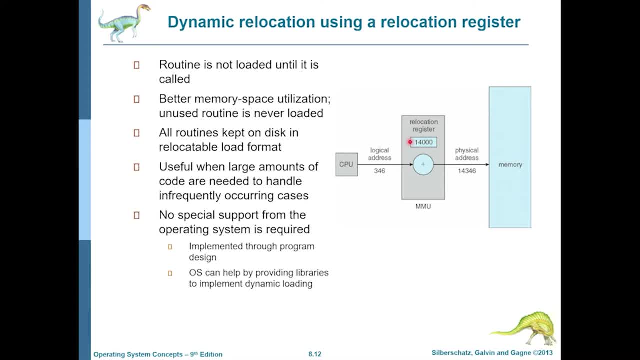 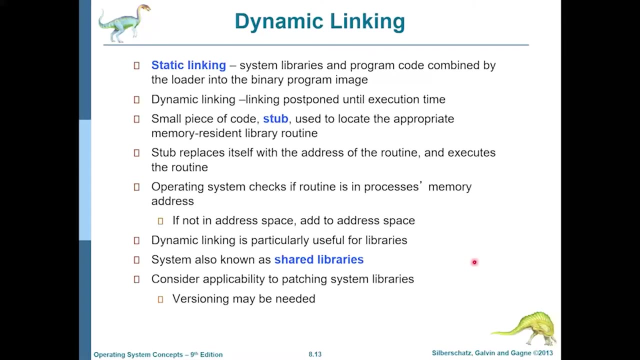 simple. but there was a problem. if the programs would not choose these values carefully, then they might be overriding memory areas of other processes. so ms-node provides very little memory protection. so we talked about dynamic libraries a little bit ago. this slide talks about much of the same thing. if all the code that your program will ever need is put into one executable. 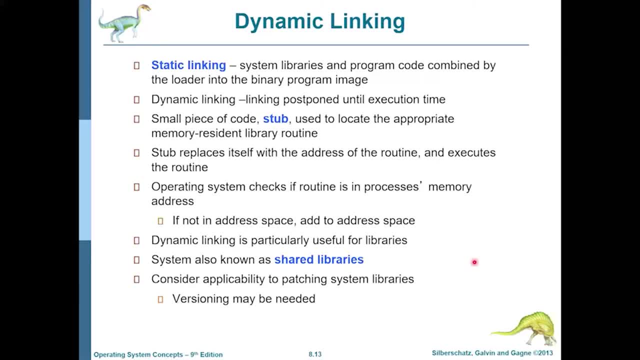 then that is called static linking. at run time your operating system does not have to handle any missing code because every function that you need in your program to get a successful result is right there in the executable that you compiled and linked. but that will usually result in big executables because there are some functionalities like 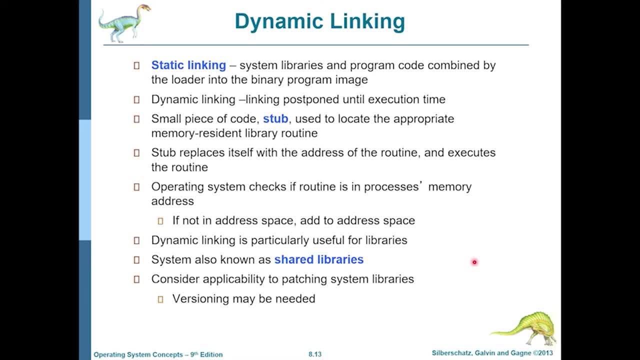 functions and modules which are so commonly used that it is better to keep them in one dll, a dynamic link library, and then at run time it is better to just get the code right there dynamically. so you're running a program which has got some functions whose code is. 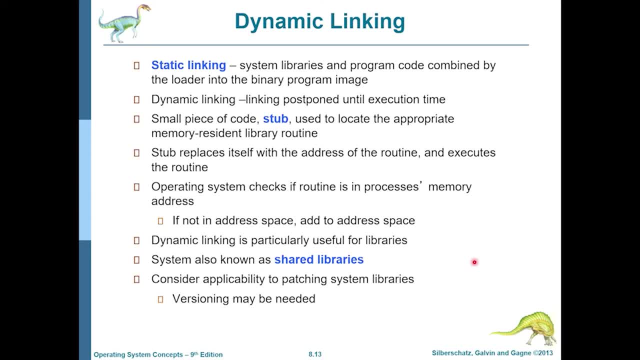 not there in the program, so your compilers and linkers will leave a stub at the end of the program and say, okay, here is the function, but i don't have the code for this. hey, os, whenever there is a need to call this function, you need to look at a dll, a dynamic link library. 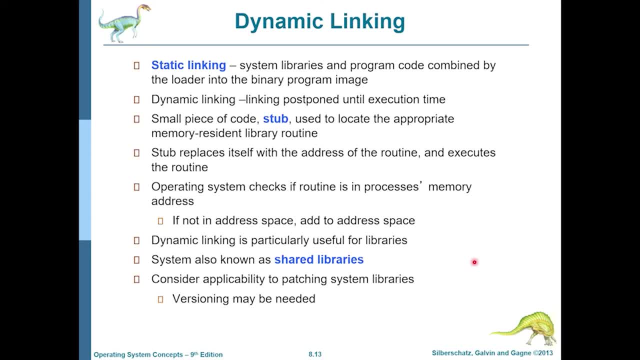 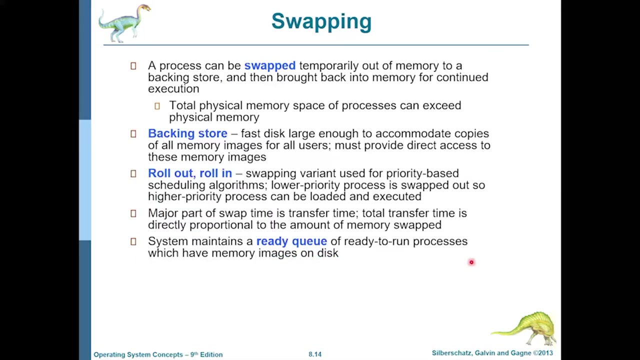 bring in the code, give the program the address and at runtime the program will dynamically jump to that function, do its job and come back. and this concept is called dynamic linking because the linking of functions to your executable happens dynamically at runtime. it is not done automatically at compilation or linking time. now let us take a look at the concept of 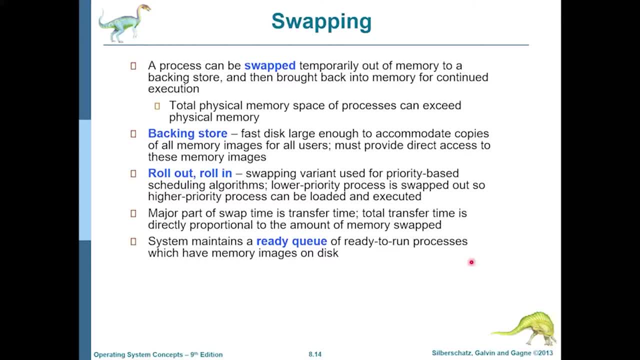 swapping now. as you probably already know, when you were little and you had smaller computers and we used to usually talk about things like: my computer is running out of memory because i don't have so much ram. my computer is running slow because i just have 8 mb of ram, if you. 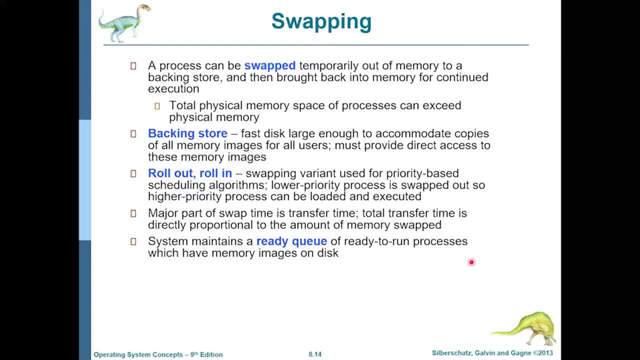 have 32 mb of ram, then maybe you can do it right now. if you have 32 mb of ram, then maybe you can run this game now. why that used to happen is usually the ram that we have is not enough to hold the memory images, the working copy of all the processes that are running. 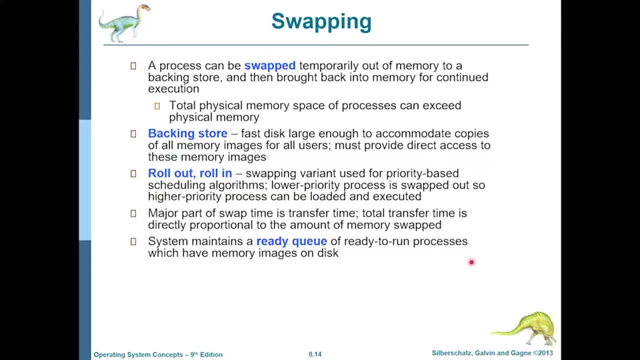 in the system. now, if you run out of memory, what the operating system can do is take a few low priority processes and swap them out to your hard disk or some other speedier media. speedier as in it cannot be a floppy drive, for example. a floppy drive is very difficult. 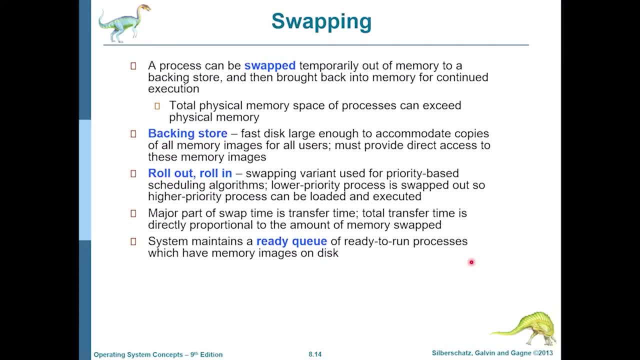 very, very slow, speedier in comparison to a very slow thing like a floppy drive, maybe your hard drive or your flash memory, your ssds and things like that. it can have a backing store in those kinds of media. it can take the memory contents of a process and it can. 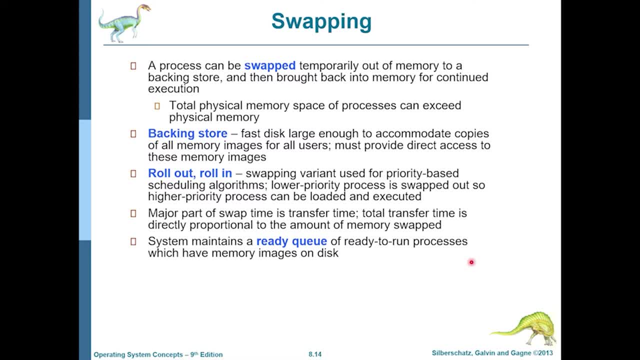 store it in the backing store and it can also maintain a ready queue of all the processes in the backing store and whenever there is a need for the process that is not in memory but it is ready to run but its contents are in the backing store, it can swap that process into memory. it can bring the contents from. 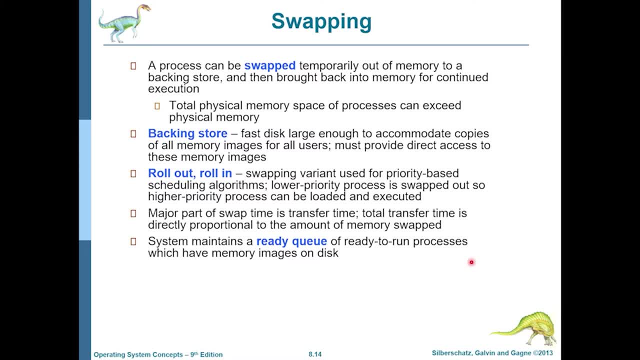 the backing store and put it in main memory and then it can start running the process. a process that is not in main memory will not be able to run, but if you are running out of main memory you can temporarily swap out some processes, their memory contents and 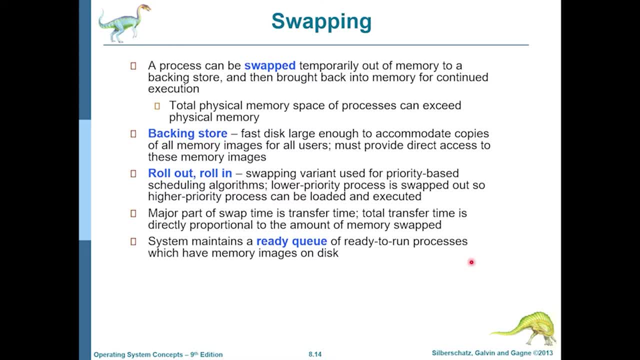 put it in a backing store and you can maintain a ready queue. if that process is Ready to run and the scheduler wants to schedule that, then you can bring that process from the backing store. that is your hard drive or your what we used to call the speedier memory, and they will bring it back from the backing store and put it into. 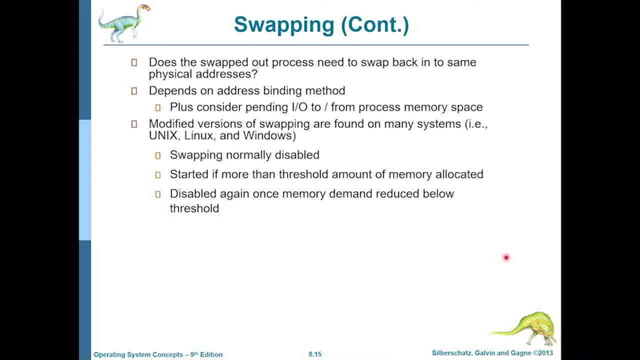 your main memory and then the process can start with swapping. does the swept out process need to swap back into the same physical address? let just say there was a process that was running at address number 500 and therefore there're lot of challenges associated with swapping. does the also become sloshed or there is a need to swap back into the same physical address? let just say that there was a process that was running at address no 500 and then there was a process of thats why an address negative or a 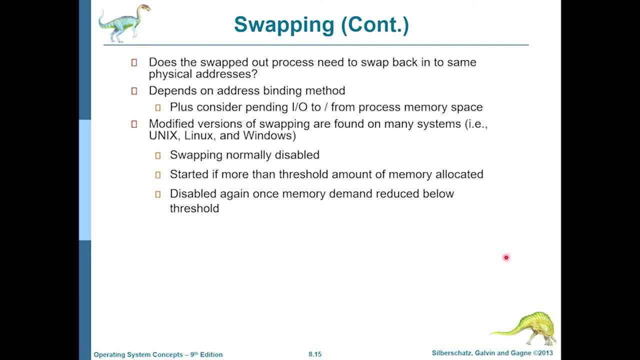 500 and then it had 1 MB of memory from that address. from 500 it used to use 1 MB of memory. now you swapped it out and you swapped in another process at 500 now the process that was swapped out. if you want to run that, you cannot just swap it in and put it at memory address 500 again. 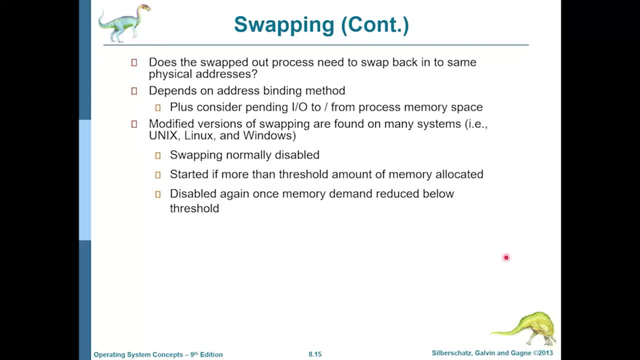 because there is another process that is running at the same physical memory. so that is one challenge of swapping. now, you can only swap out a process if you are sure that the process is idle with respect to input, output, for example, if the process had a buffer inside its memory range. 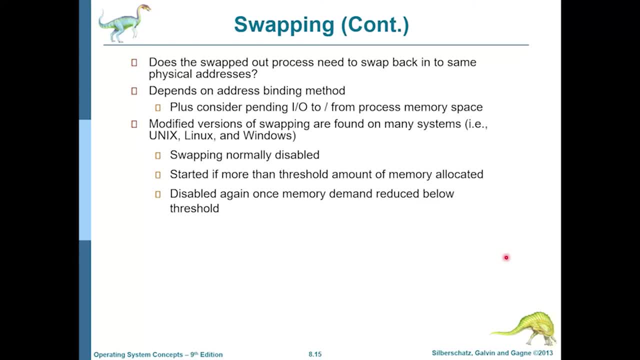 and it was trying to read something from the hard drive. now, before that thing could have been taken care of, the operating system swaps it out and puts a new process in the same memory location. now what might happen is that the contents of the hard drive can get written into the wrong memory. 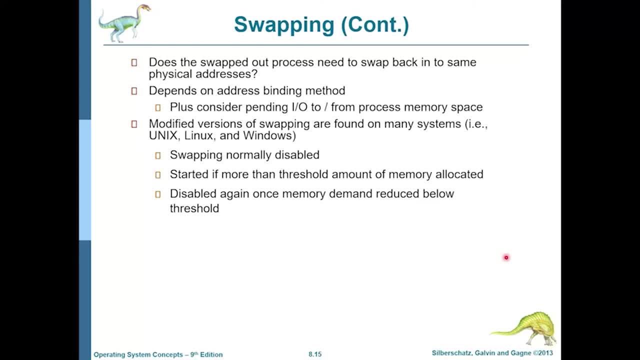 area, i mean the memory area, is the same, but the process has been swapped out and another process is running there, so that can be a problem. a solution to that is to always use the kernel, that is, the operating system, as an intermediary and say, okay, you create a buffer inside you, whatever the hard drive reads. 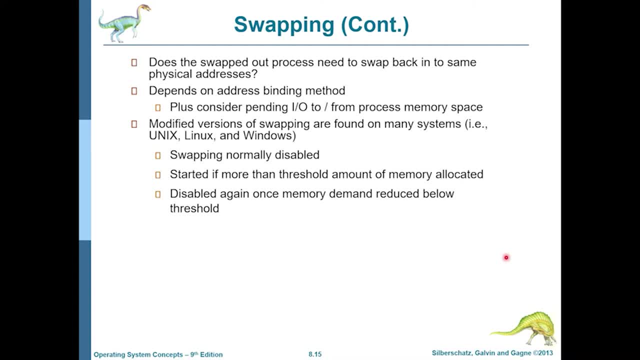 you put it inside your buffer and give it to me whenever i need it. but this can lead to a problem called double buffering, which is totally unnecessary and that can be one problem of future history, to where it looks like the system has already been disabled. but if the memory availability is running really, really low, then swapping can be enabled in systems. 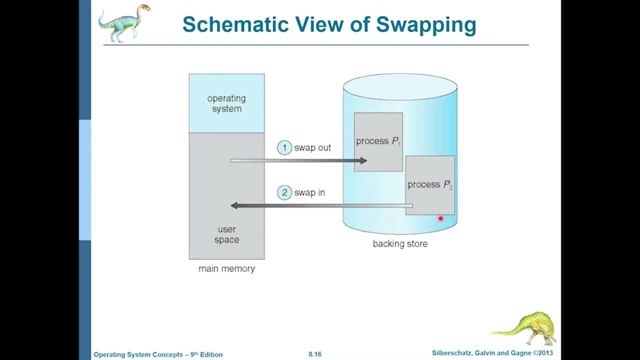 this is just a schematic view of swapping. so, as you can see, there was a process running here. it gets swapped out and it is stored in the backing store. another process, p2, gets scheduled and that runs for some time and maybe at one point of time the backing store is one of those speedier auxiliary memory devices that we have: hard drives. 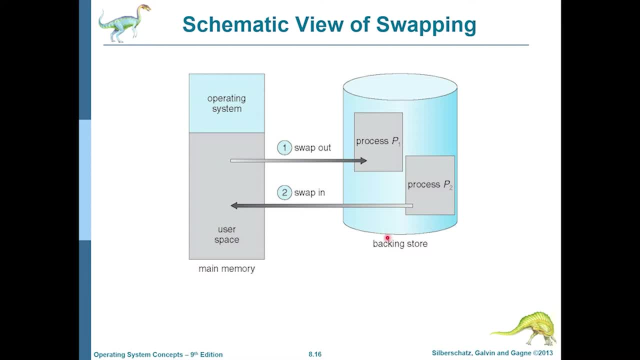 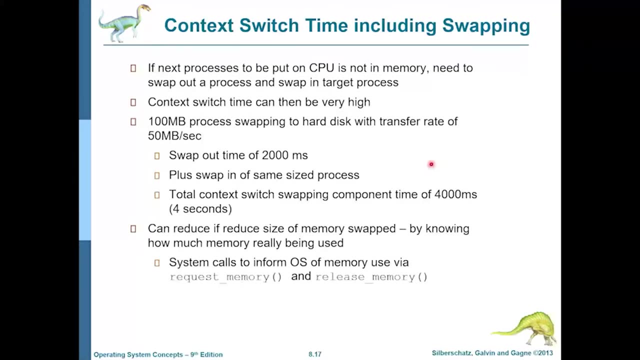 or ssds or splash memory and things like that, and main memory is your ram. now let's discuss the consequence of swapping with respect to context switching time. so what is a context switch when the cpu is running one process and then it has to go run another process because, well, 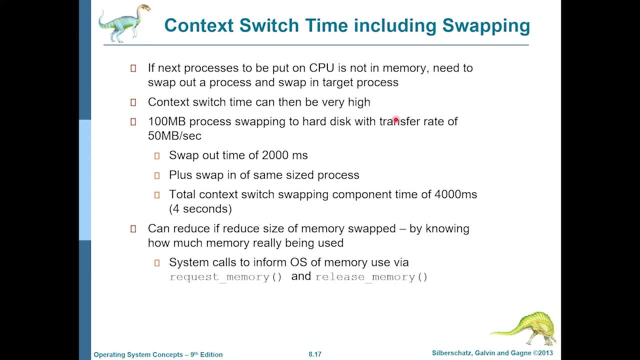 the cpu's time needs to be shared by different processes, then it needs to context switch it, it needs to remove one process from its execution and it needs to put it back in memory somewhere safe so that it can resume its execution at one point of time and then it brings in another process. 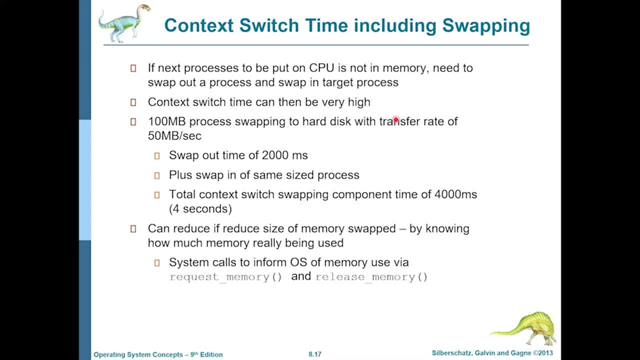 and starts executing that process. now, if the process that it wants to execute is not in memory but it is stored in the backing store, then what happens- so that process happens and then it starts executing that process, and then it starts executing that process- has been swapped out in the backing store. it has to be brought back into the main memory and only 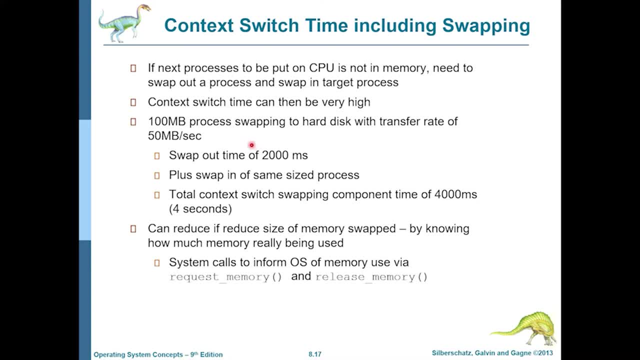 then its execution can start. now let's see: if the hard disk transfer rate is 50 mb per second and if the process size is 100 mb, then swapping one process out can take this much time and swapping another process of a similar size in can take another 2000 milliseconds. here we are assuming. 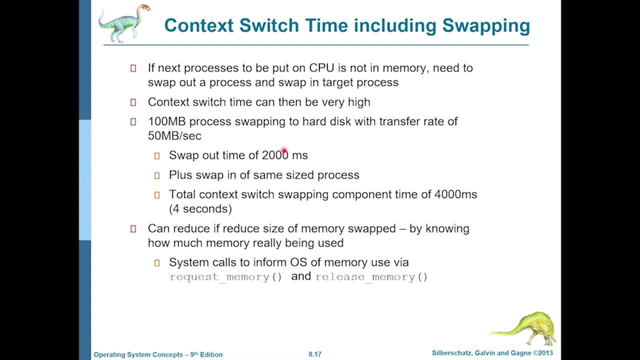 that before one process can be swapped in for execution, another process has to be swapped out. because we're assuming, because swapping is going on, memory should be almost full. so for one process to come in for execution from the backing store, another process has to be swapped out. so this combined. 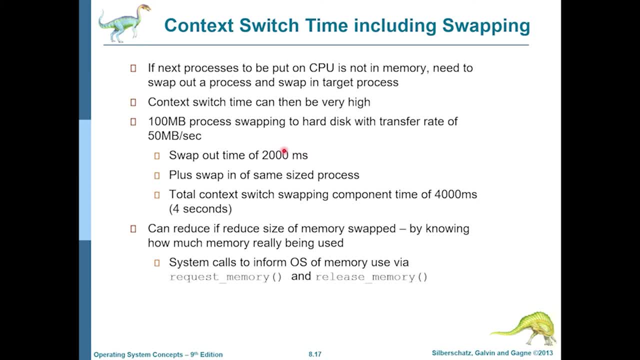 process of swapping out one process and then swapping in another process can be two into 2000 milliseconds, that is about four seconds- and then swapping out one process can be two into 2000 milliseconds and then swapping out one process can be two into two and then two meters across. 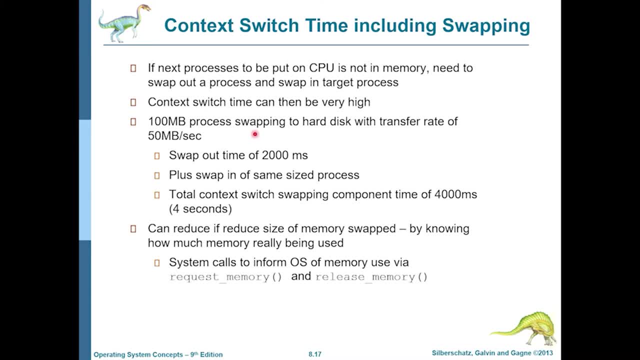 and then two meters across knee of goddess and then two meters across is an enormous amount of time compared to normal context switching, in which it's just a matter of microseconds, maybe to swap one process for another. this swapping time can reduce if the amount of memory that is used by processors is is less and also it is very 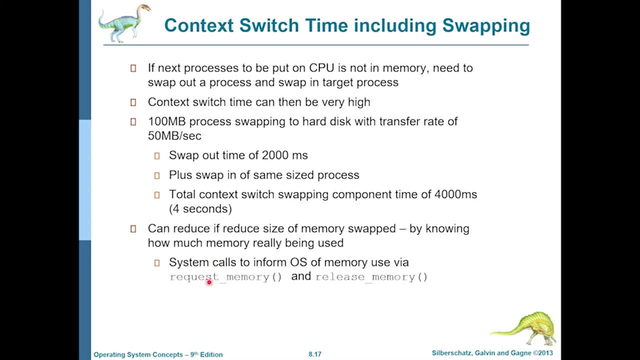 very well known to the operating system. so if processors can make use of system calls like request memory and release memory, so the operating system can do a very good job at bookkeeping of how much memory can be used to execute what we can have in the process to execute one process. 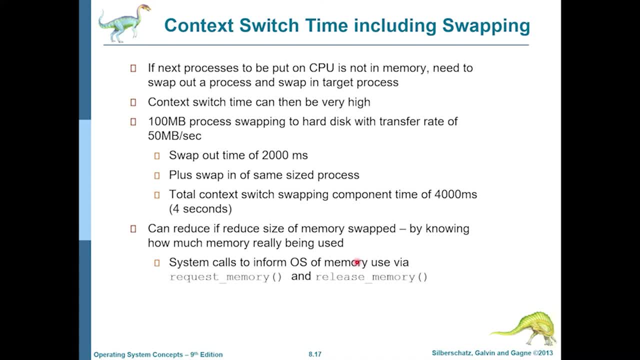 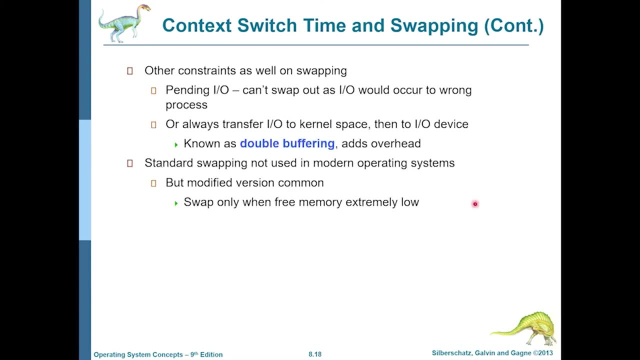 memory a process is using and that can make this process of swapping out and swapping in a little bit more efficient. We have already talked about the contents of this slide. I mean, I was talking about pending input output buffers that are there in a process that might. 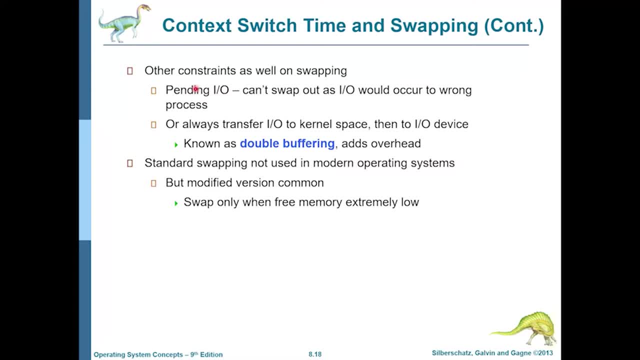 be there in a process. So the process was going through some input output and then it also had some buffers for filling in the input output data. And if the process was swapped out before it could even get the data, then what can happen is that the wrong process might get that data or the data could override some essential 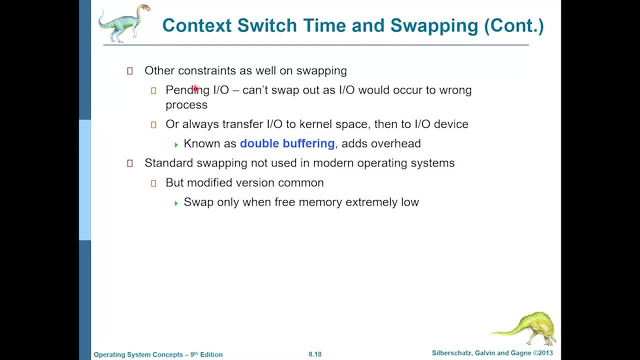 memory contents of another process, The process that has taken the place of the old process which got swapped out. Now processes might want to use the kernel space for buffering of their input output data, but that can result in double buffering, because the kernel will buffer it once and 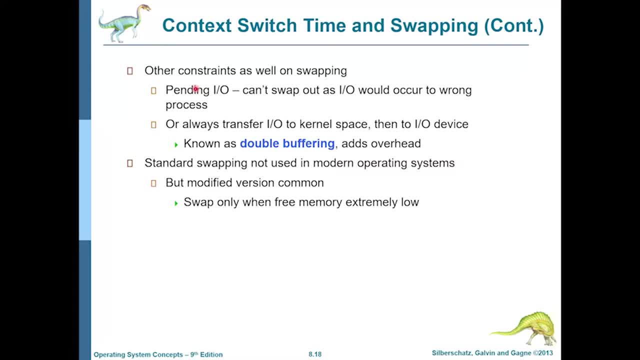 then it will transfer it to the buffer of the process And that is not very, very efficient because swapping is a very, very time consuming process so far as context switching and input, output and these things are concerned. So swapping is kind of disabled in modern operating systems and swapping is only enabled. 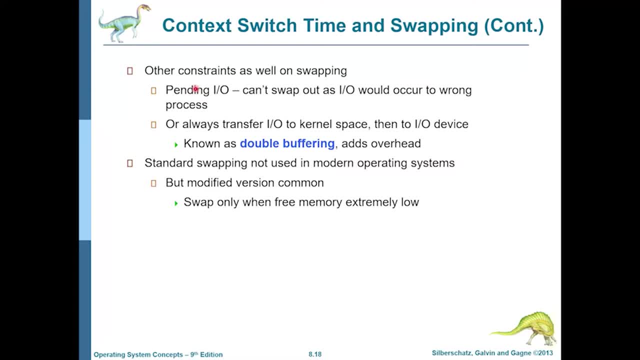 if the memory is running really really low. Memory availability is running really really low. But modified versions of swapping do exist in which you don't swap out entire processes. You choose to only swap out parts of the process. So that is not very, very efficient because swapping is a very, very time consuming process. 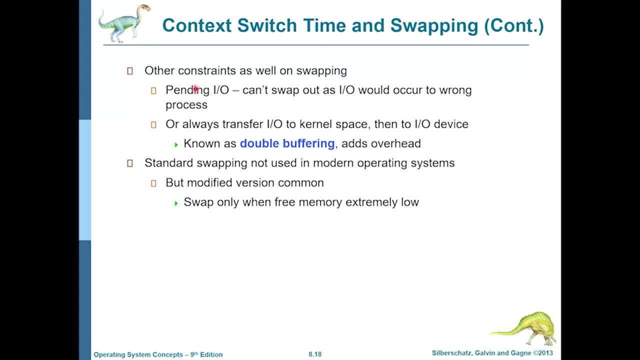 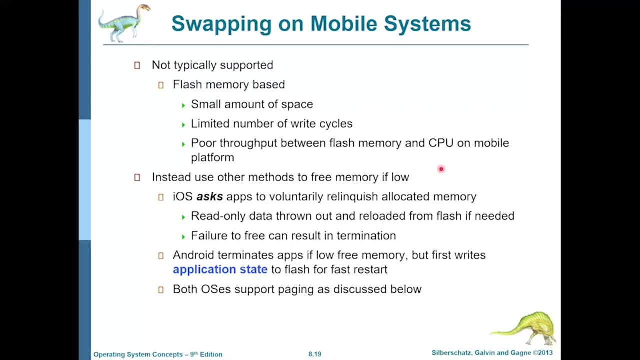 And we can see how this is done in the context of paging, in which we can swap out parts of a process and then bring them back as and when the process needs, those so called pages. In mobile operating systems, swapping is not allowed: Android and iOS, both of them don't do it. 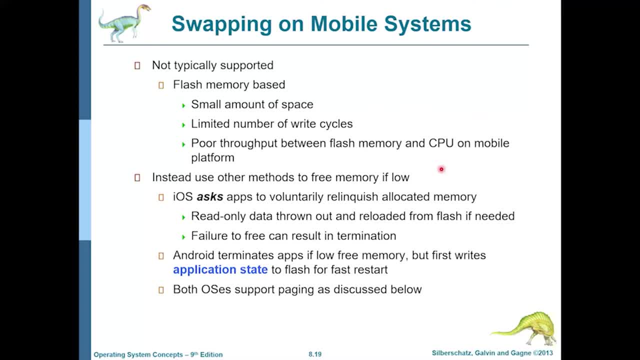 What they do is something very, very novel. when memory is running low, they ask the apps. we call it applications as apps. As you all know, the operating system asks the apps to terminate execution but also save their important state information somewhere, the state bundle somewhere. So if there is an calculator app, then the calculator app might want to store its entire. 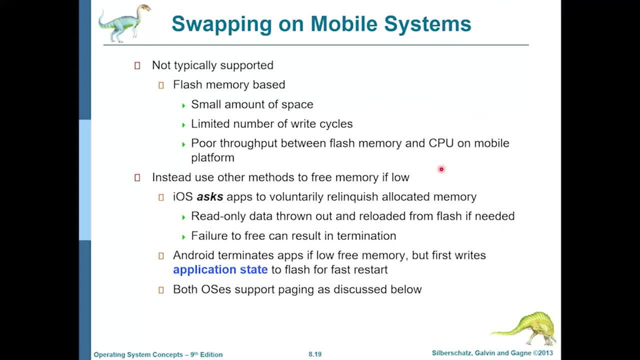 stack of what all operations the user had already done and what was the current answer on the screen, and all of those information That can be saved into a bundle and thrown into the hard drive or the SD card or some persistent storage like that. And if the operating system wants to bring the calculator app back to life, then it can. 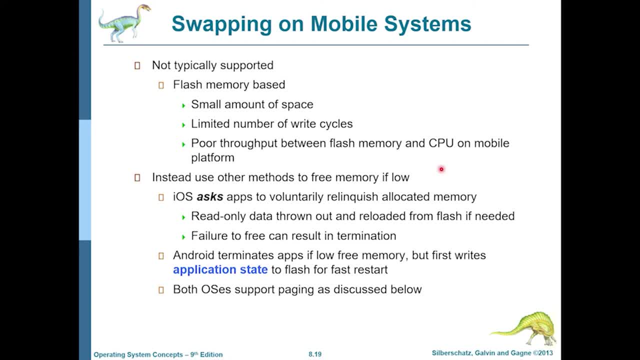 draw the UI, because it can always draw the UI, because that information is right there in the executable. But the state in which the calculator app was there can be restored from the bundle and to the user it will look as if nothing has happened. But in the meantime, when the operating system was running low on memory, it terminated the 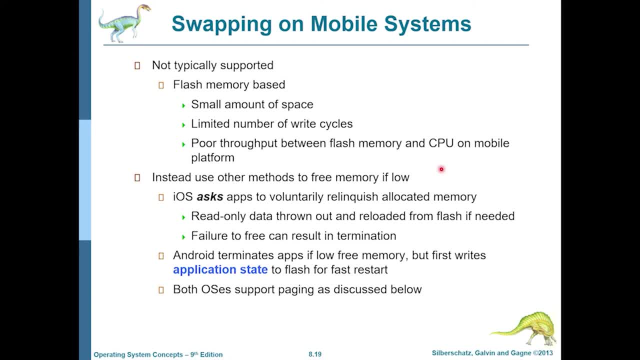 calculator application After saving its important state information And then use the freed up memory to run something else, and after some time, when the user wanted to go back to the calculator application, it looked as if nothing of that sort had happened, And both iOS and Android do something similar like that. 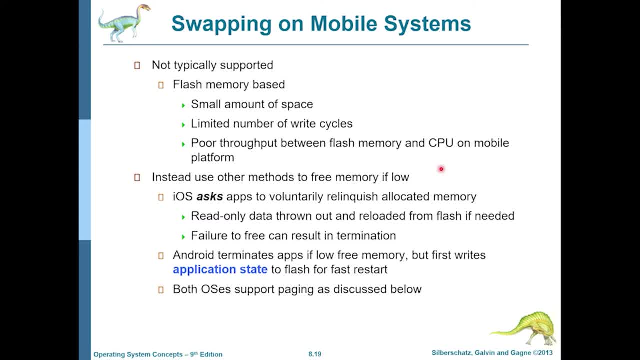 Both the OS's- Android and iOS- support paging, though, and because of that, parts of applications can be swapped out, Some pages of an application, But the entire application, as in the traditional swap out, does not happen. Parts of applications can be swapped out and swap in, and we will see that further in this. 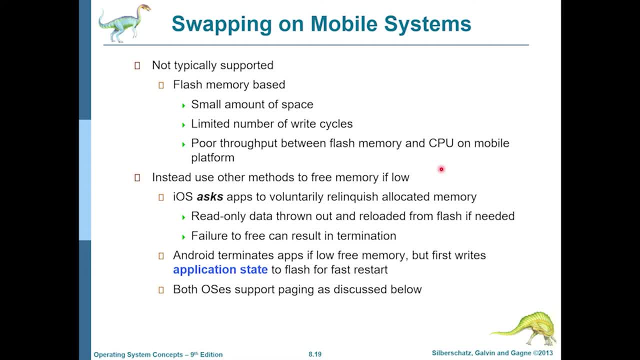 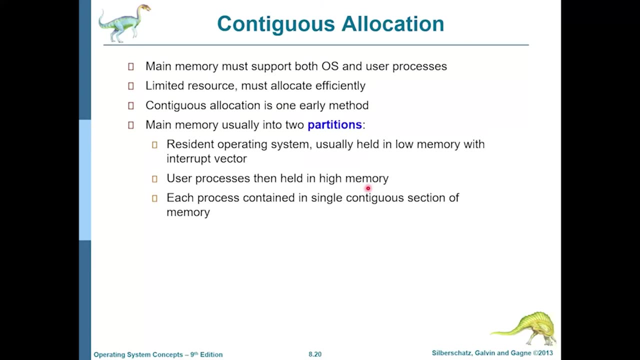 chapter and in the next chapter as we go. But this traditional swapping out and swapping in of throwing out entire processes to a backing store and bringing them back when required even does not happen in Android and iOS. Let's discuss a mechanism through which memory was allocated to processes and the operating. 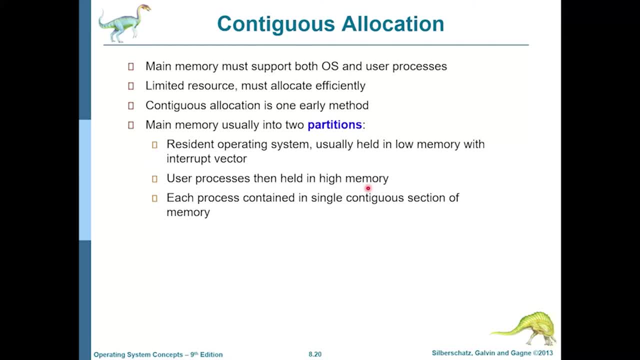 system. What are operating systems? Usually, the lower memory addresses used to be given to the operating system and the higher memory addresses used to be given to processes, and each process used to be contained in a single contiguous section of memory, As in. there would be no interruptions in the range of memory that is allocated to a process. 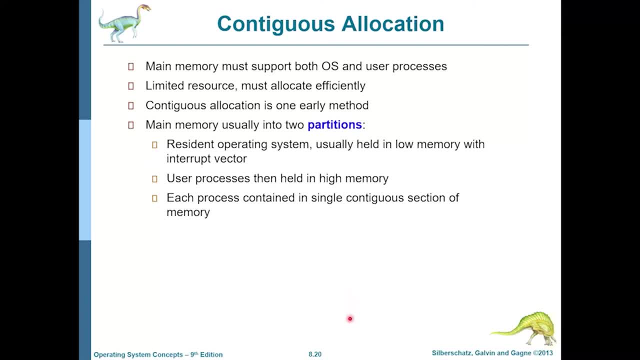 The process begins at one place, then it will just continue contiguously till it ends and then maybe another process can begin From where the first processes. memory addresses stop And the operating system is given the lower set of addresses and the upper set of addresses. 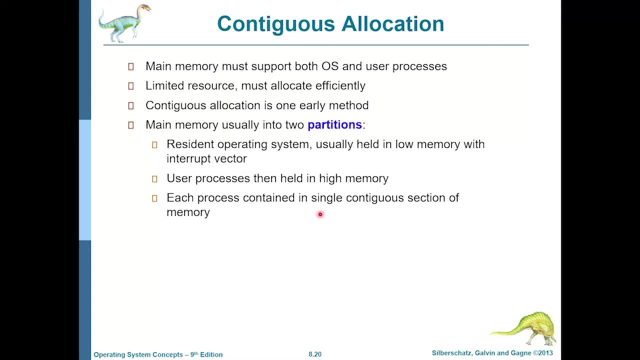 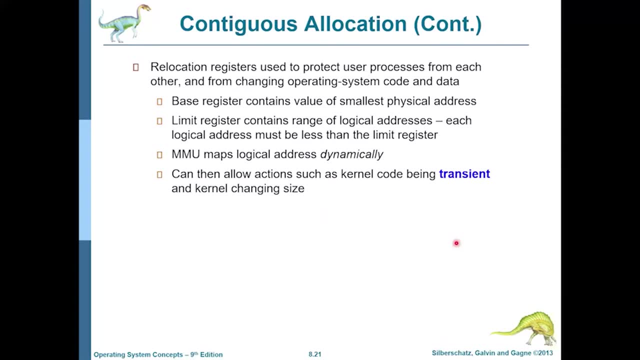 go to processes And the memory for the operating system and the processes are allocated contiguously- And we have also studied this before- and protection can be achieved if memory is allocated contiguously using relocation registers, And it is a job of the MMU to map logical addresses. 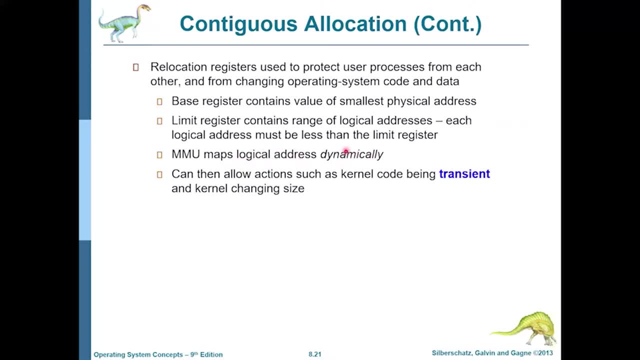 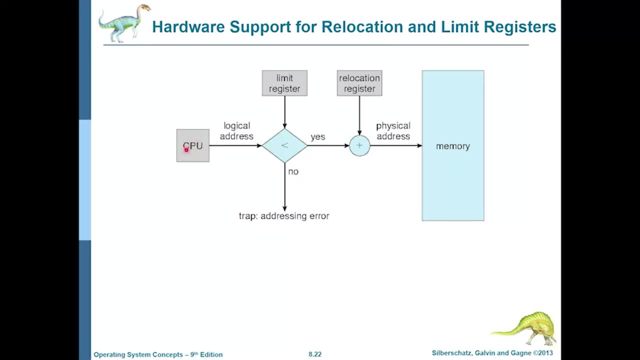 So if the memory is allocated contiguously, then it is a job of the MMU to map logical addresses. It is a job of the MMU to map logical addresses dynamically, as you can see right here. So there is a CPU and that generates logical addresses. 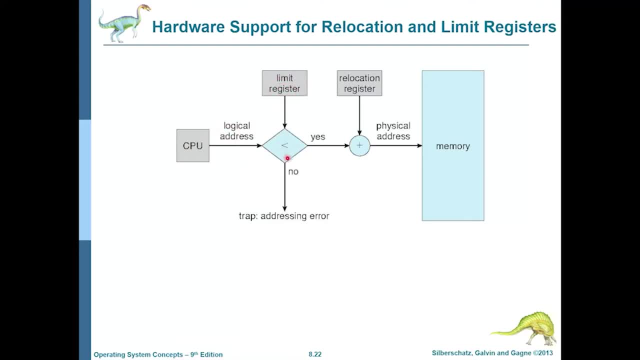 So there is a limit register which says, okay, are you within the limit? If not, we will trap. If yes, then I'm going to add the contents of a relocation register to you and then a physical address is created. So this is the job of the MMU, right here. 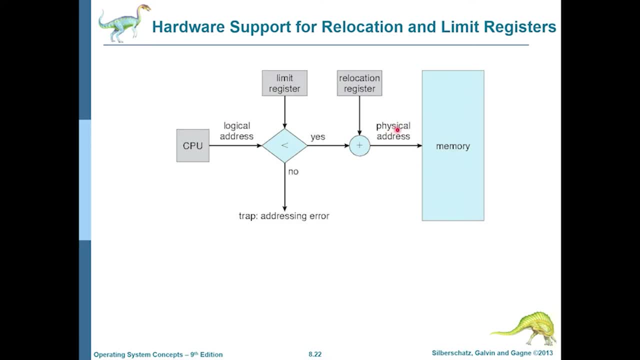 right here that takes a logical address and converts that to a physical address. it does a check, then it adds a base to give you a physical memory, and this is how processes used to run in older operating systems. so for the process it does not really matter where it is running, as long as 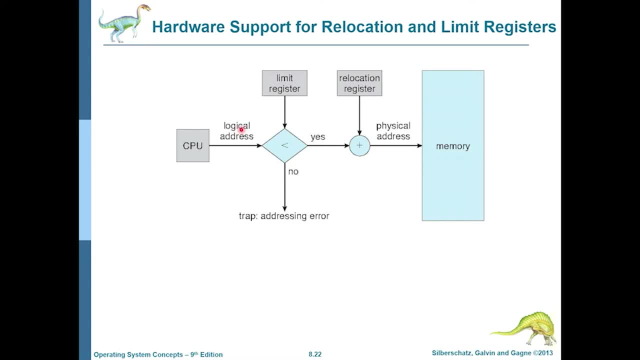 its logical addresses follow a continuous pattern, so there are no gaps in the logical addresses that it generates right and the operating system can also guarantee that those logical addresses are also contiguous over here, because the mmu cannot introduce any jumps. all it is doing is checking for a limit to make sure that this process is not trying to access addresses outside the range that. 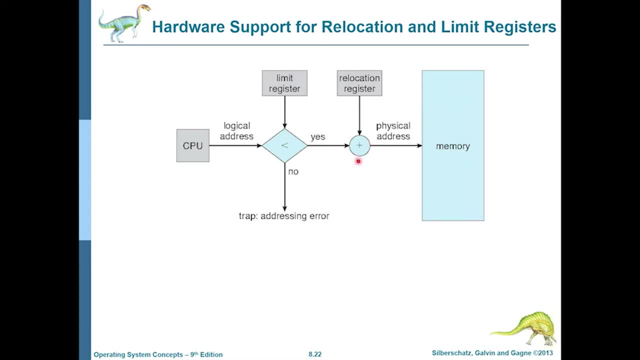 it is supposed to access within and, and that wherever it is placed by the operating system, its base is stored in a relocation register. you might be somewhere over here, so the process might be present somewhere here the second time. if it is running, then the operating system might allocate the process somewhere over here, and so the 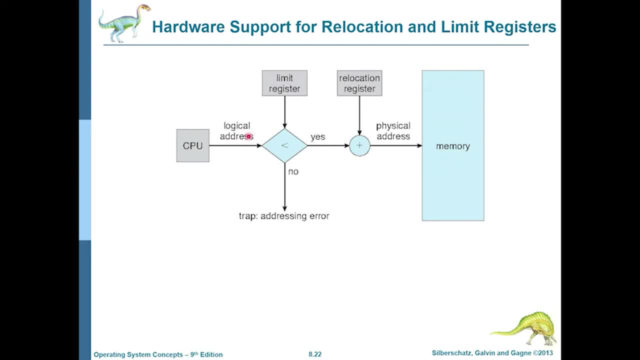 relocation register might be somewhere over here. so for the process it does not matter where it is placed. for the os it it matters that the c that the cpu- whatever addresses the cpu is generating- is within the range. and it also matters to the operating system that, wherever it has placed the 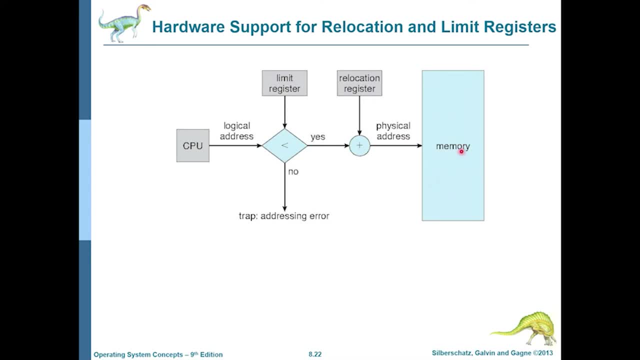 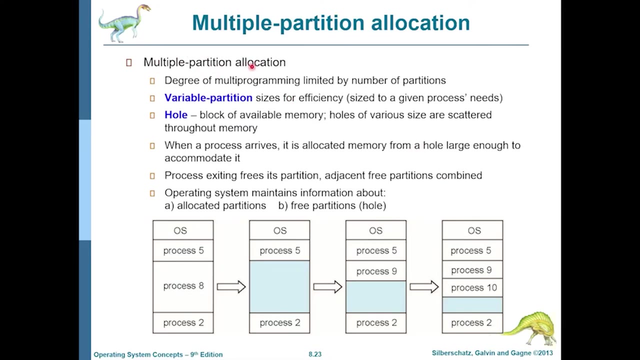 process. the physical addresses are actually getting generated in that region because the relocation register has been set to the base of that region. in the context of contiguous allocation, there is something called a multiple partition allocation, in which each process can be of varying sizes. here, as you can see, process 5 is small. as you can see, process 2 is small. as you can see, process 3 is small. 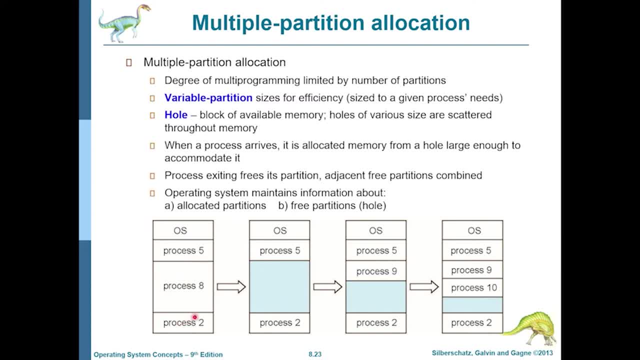 process 8 is really really big. process 2 is again small and the entire memory is not partitioned into any fixed size partitions, so the partitions can be of varying sizes and so just imagine this situation over here. so the operating system is always there and after the os has been given. 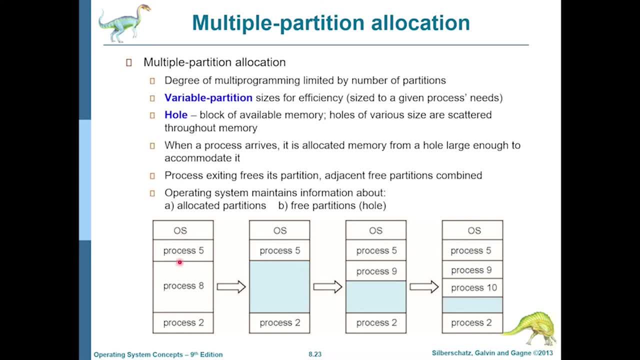 its area. here you can see the rest of the processes that are present in the system at this point of time. now, process 2 has definitely come before processes 5 and 8, but when process 2 arrived, then this was probably the best place to keep it, and when process 5 arrived, then this was the best place. 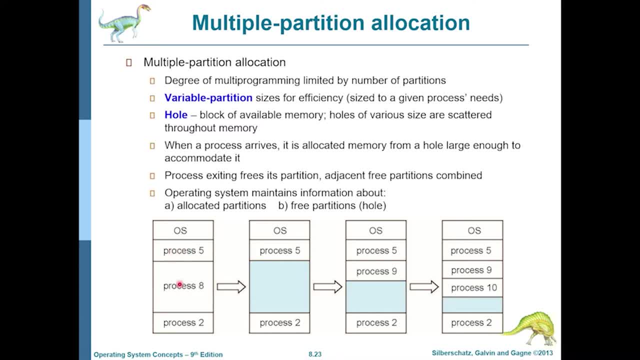 to keep that and process 8 was able to just fit into the gap between 5 and 2. they arrived in different orders, but at this point of time this is the state in which the processes are arranged. so if process 8 exits then a whole system is not there, because the losses are always available and 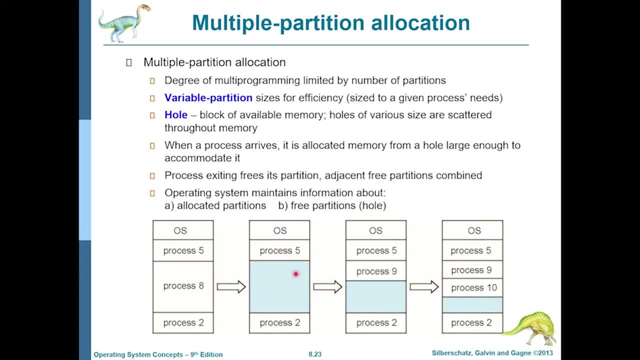 the processes where the losses are always. there will be differences between them, however. when you a hole is created, so that is called a free partition or a hole, whereas process five and process two are called allocated partitions because they still exist now when process eight exits. then there is this huge hole that gets created now when process nine comes in. 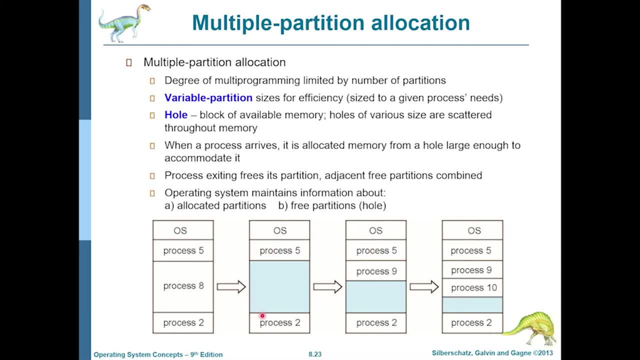 then the operating system will use some algorithms to figure out a an appropriate hole for the process. now that can be the first fit, best fit or the worst fit, as we will see in the next slide. but depending on whatever fit it wants to go for, it will figure out a hole. 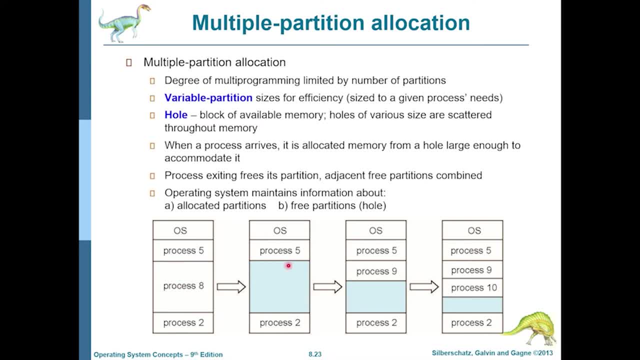 and then it will allocate some area of that hole to this process so that the process can sit there and start executing. now if another process- process 10- comes in, then process 10 can go in this hole right here, because this hole is big enough to fit process 10, and then 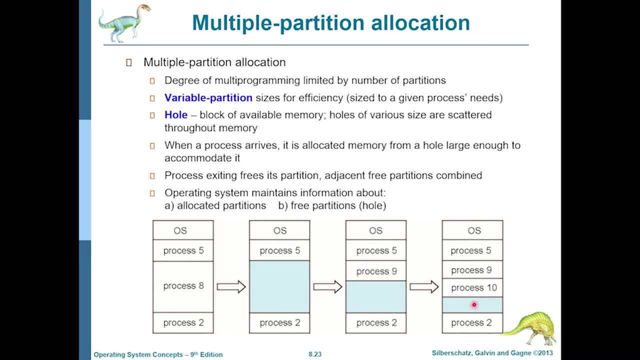 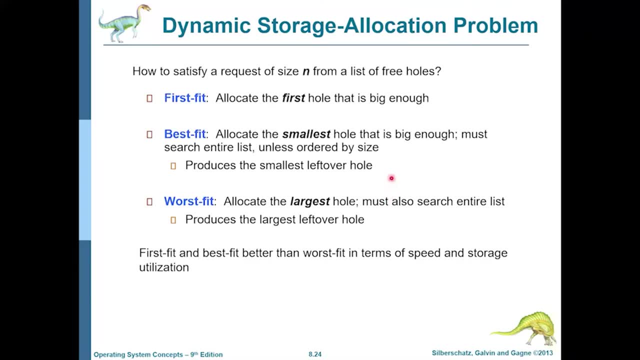 thread it and then process 10 can have a hole all the way down further away. so now this hole is complete and there is still another small hole over here which the os might use later. so there are three ways in which the operating system finds a hole large enough. 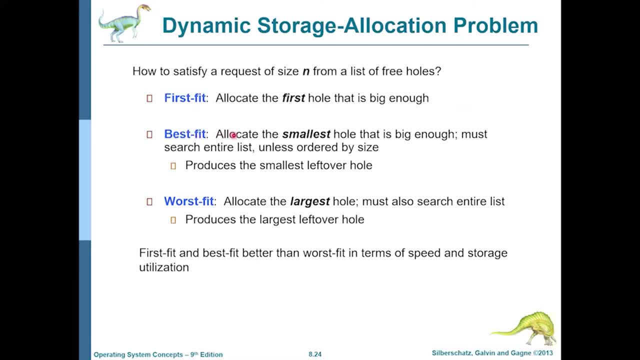 for a process to fit, it can do first fit. so it goes through the list of all the holes and the first hole that is large enough to hold a process is chosen. then there is a best for a huge hole and then take a small chunk of it. it will go through all the holes in the system. 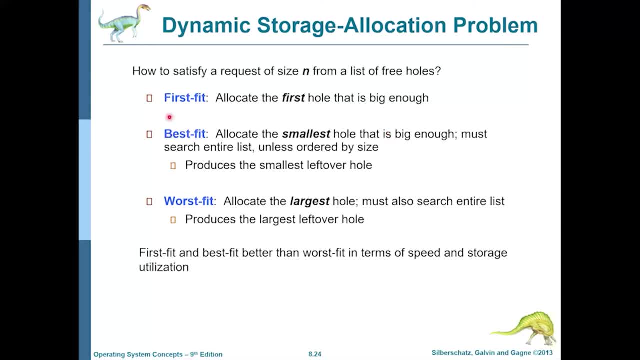 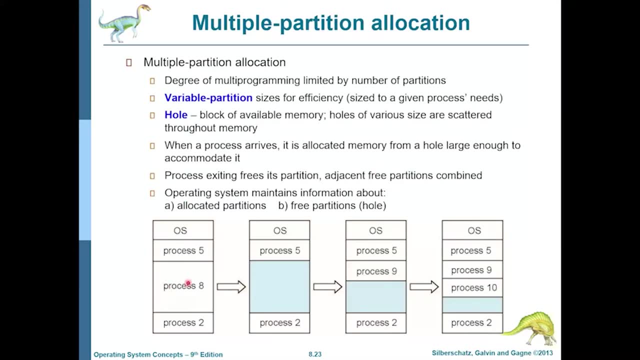 and figure out which hole is just big enough for this process to fit in, and this produces the smallest leftover hole. leftover hole as in when process 8 exited over here and process 9 came here. so this is the leftover hole. so, but process 9 was really small, it did not need such a big hole. 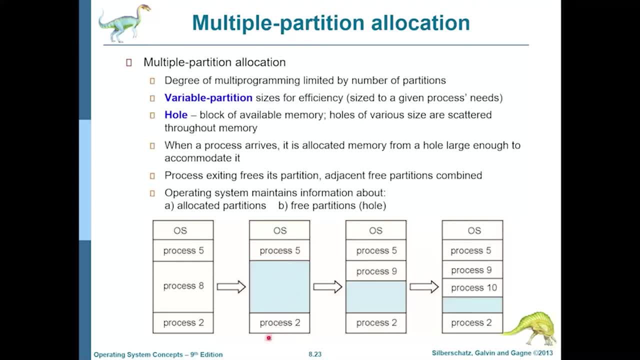 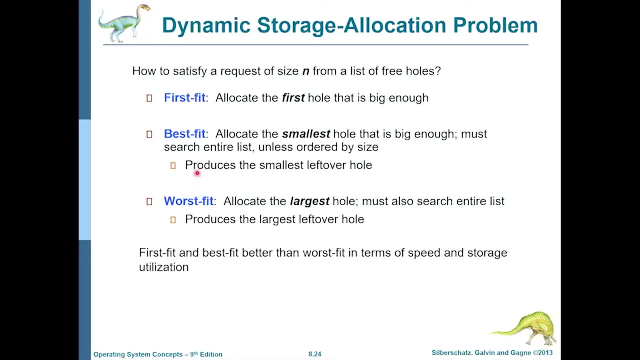 so if the operating system could have gone below process 2 in the entire memory area and found a hole which was just a little bit bigger than process 9, then the leftover hole would not have been this big as we see over here. then there is a worst fit. i don't know why would anyone want? 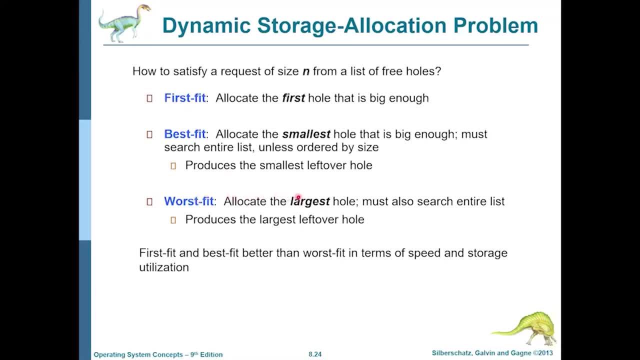 to do that. but in this strategy you allocate the largest hole and you must also search the entire list and figure out the largest hole and then give that largest hole to this process and this produces the largest leftover hole. so first fit and best fit work better than worst fit in terms of speed and storage utilization. 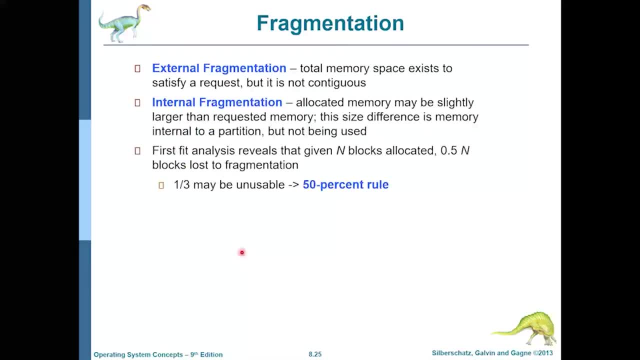 two kinds of fragmentations can happen if memory is allocated the way we were talking about. external fragmentation can happen when the total memory space exists to satisfy a request, but it is not contiguous. so, as you saw in the previous video, you can see that the memory space is. 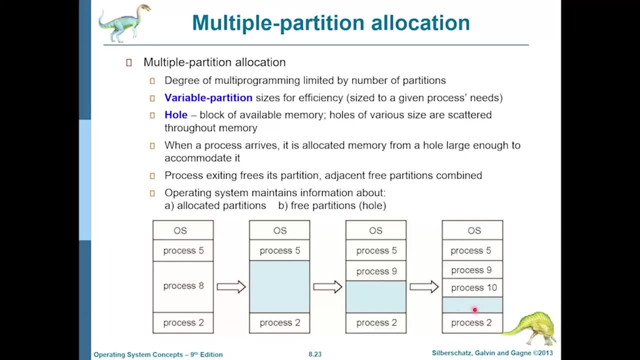 this already opened. so if say, we want to draw a 3d model, which might be small, well, let us take an example right here. so let the model looks like this: we have the space system in place, so it is here like this, and what this means is that we take the length from the. 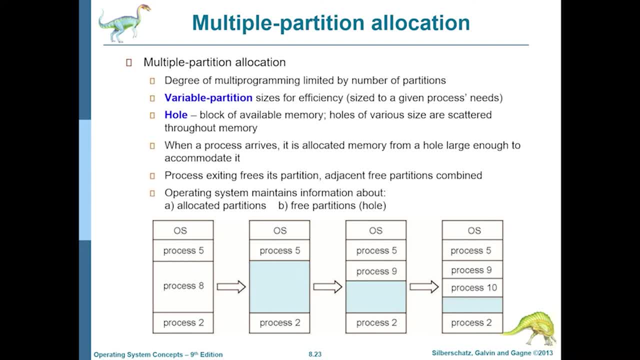 terminal. now, when dot comes down it is under theLET Restaurant. the lighter� shows that dot is still under the compile. then dot comes down again. so all of the centimeters from the terminal which is being collected, depending upon the unit we are talking about, is still. 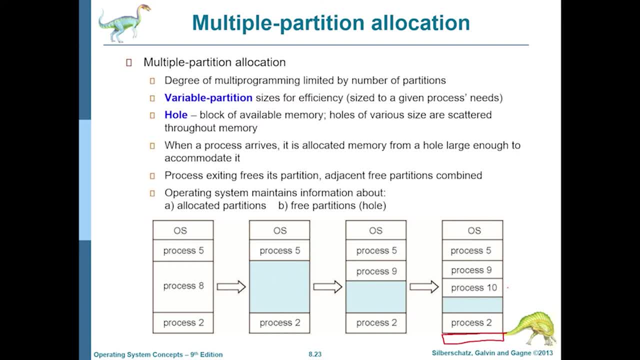 a0 after dot bar sounds like the one before we have the locals term� with dotmail argue. so at this point, this study does not includeенные containers, facebook as well. for the point w, then to theWhat else що I want to say? that, in two-dimensional order, the idea is that, as a 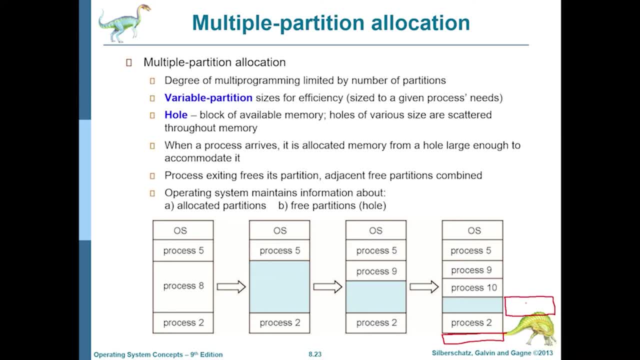 things can be solved: this one as a fight, that as a function. qli thought better to terror or a yourselves. now, this process cannot fit into this hole. it cannot fit into this hole, but it could have easily fit into the combination of the size of this hole and this hole. but since we really want, 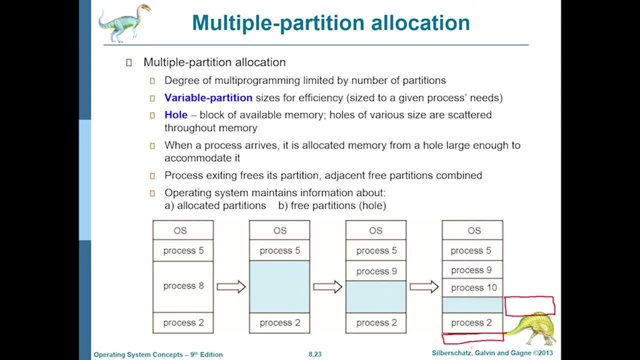 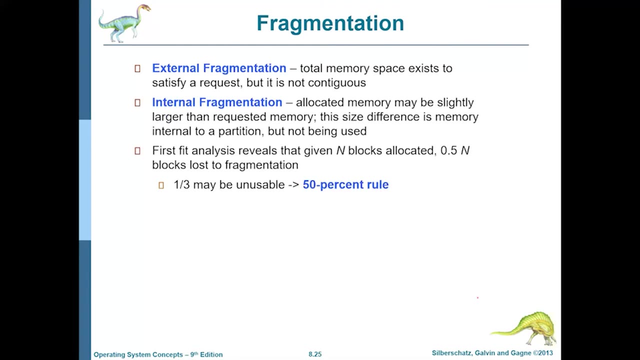 to do contiguous memory allocation. these two holes are of no use for holding this process. so these two holes that are kind of far away because process two was sitting in the middle, these are the result of external fragmentation. internal fragmentation can also happen. now, when we were talking about contiguous allocation, 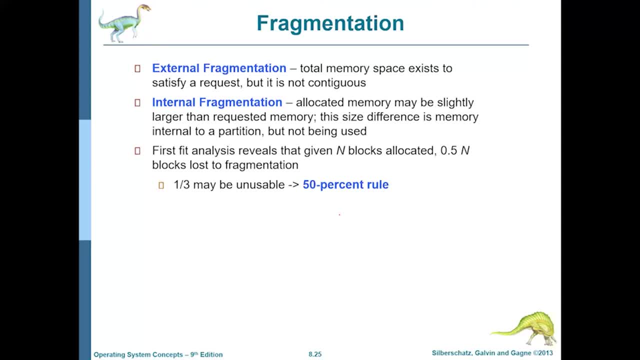 we decided that we will not be using any fixed size partitions. all the processes could have varying amounts of memory sizes and we will figure out a hole and put them over there, using the best fit, first fit or the worst fit strategy. but imagine if our memory, you have a hole in the middle of this hole and you have a hole in the middle of this hole. 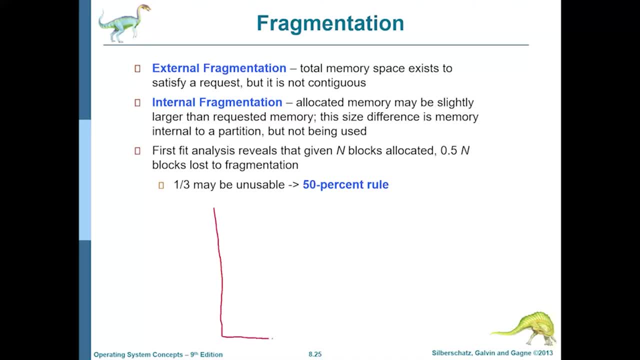 and you have a hole in the middle of this hole, and you have a hole in the middle of this hole had fixed size partitions. so let me draw some kind of memory over here and i will draw fixed size partitions. so we have one, two, three, four, so we have four partitions each of similar size. well, almost. 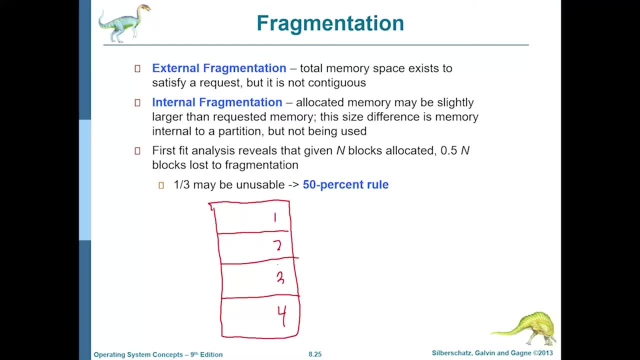 similar size. pardon my drawing, but just assume that all of these partitions are of the same size. if a process comes that takes this partition, this partition and only little bit of this partition, so this area cannot go to another process because the rule here is that one partition can only go. 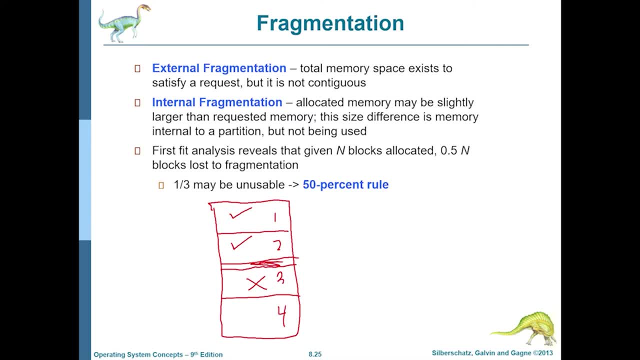 to one process. so whatever it uses here is used by that process, but the the rest of the partition- number three- is not used by that process. so that is called internal fragmentation. so if you have fixed size partitions and you allocate certain partitions to a process continuously, what can happen is that if the size of the process is not exactly divisible by the size, 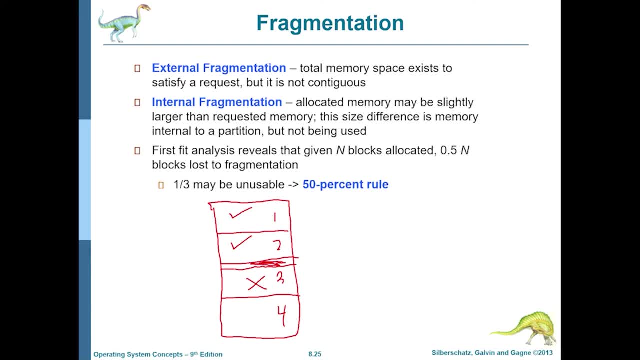 of the partitions. it can not cover the last partition completely and whatever size is left over in that last partition goes towards internal fragmentation. now there is a 50 percent rule which says that if you use first fit for allocating your memory and you have fixed size and given, given that there are n blocks, then 50 percent of those n blocks, that is, 0.5, n number of. 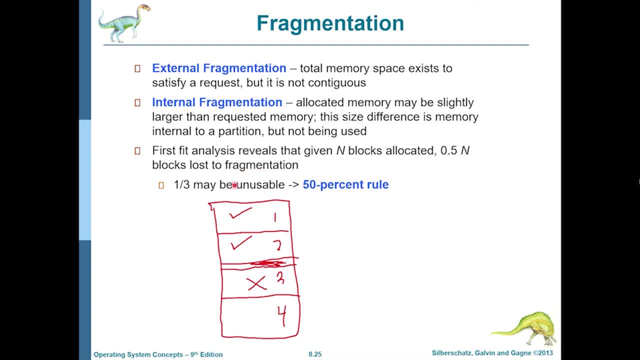 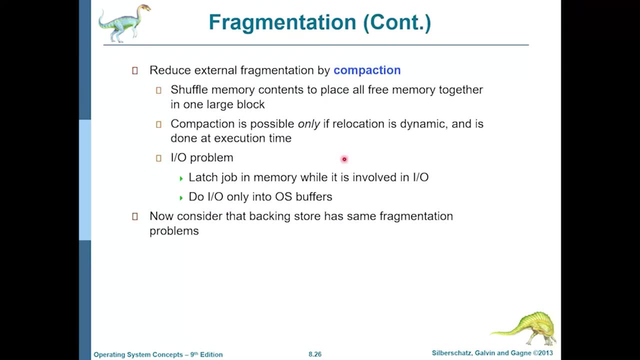 blocks will be lost due to fragmentation, that is, one third of the blocks may be unusable, and this is also called as the 50 rule. one of the ways to handle fragmentation is compaction, so what you can do is, if there are holes all over the place, what you can do is move the processes around so that 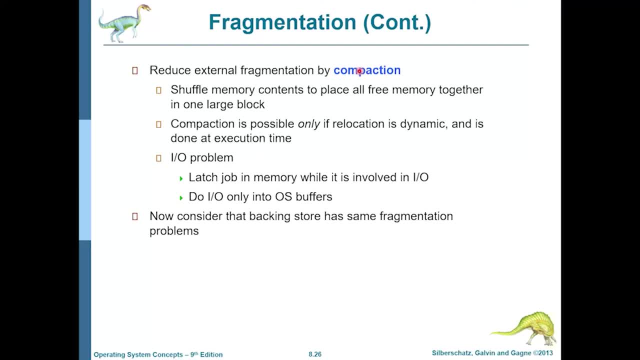 the holes can coalesce to make a bigger hole. so, for example, let me draw it again. so this is the memory area and here let's just say there is process number one, here there is a hole, here there is process number two and here there is another hole. 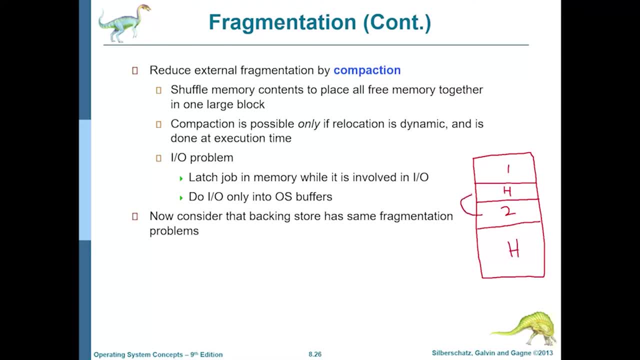 so what if we move process number two over here and then it looks like this: we have process number one and we have process number two, and these two holes can combine to become a bigger hole. now there is no fragmentation, because now this is a contiguous chunk of memory. 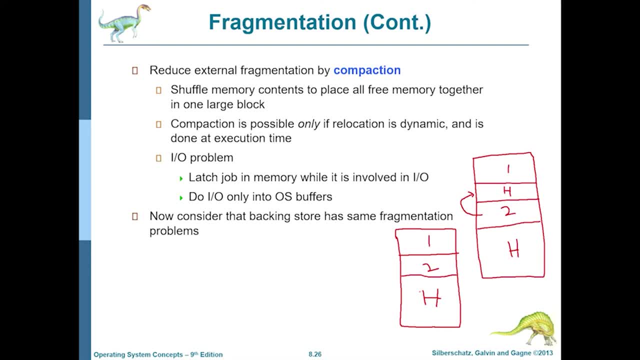 that can be assigned to any process that is equal to or just smaller than this hole. now the problem with that kind of compaction is, if the process number one and process number two are combined to become a bigger hole, then execution cannot handle the addresses that are generated by process number two. so process number two has been coded to run at this memory location. now if it moves here, the operating system execution needs to be able to rebind the addresses of two so that it can run properly at its new location. so if relocation is dynamic, if the operating system can dynamically rebind the addresses of two so that it can run properly at its new location. so if relocation is dynamic, if the operating system can dynamically rebind the addresses of two so that it can run properly at its new location. so if relocation is dynamic, if the operating system can dynamically rebind the addresses of two so that it can run properly at its new location. so if relocation is dynamic, if the operating system can dynamically rebind the addresses of two so that it can run properly at its new location. so if relocation is dynamic, if the operating system can dynamically rebind the addresses of two so that it can run properly at its new location. so if relocation is dynamic, if the operating system can dynamically rebind the addresses of two so that it can run properly at its 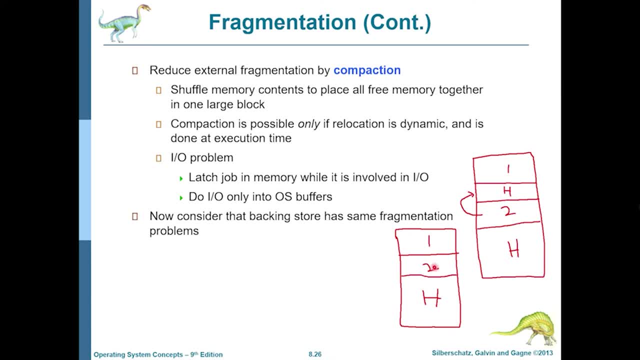 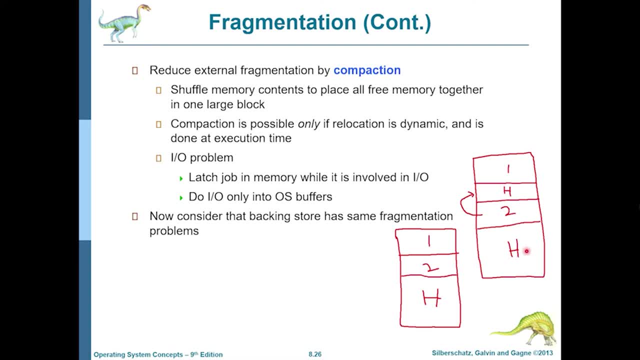 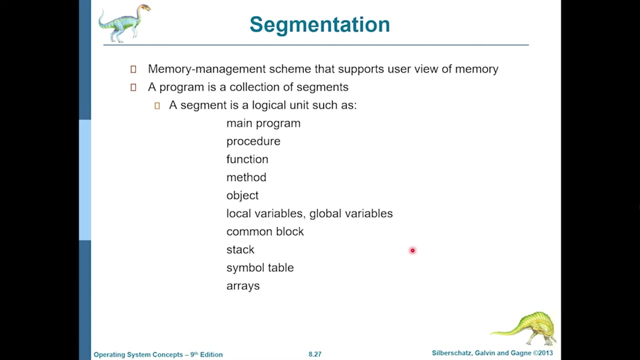 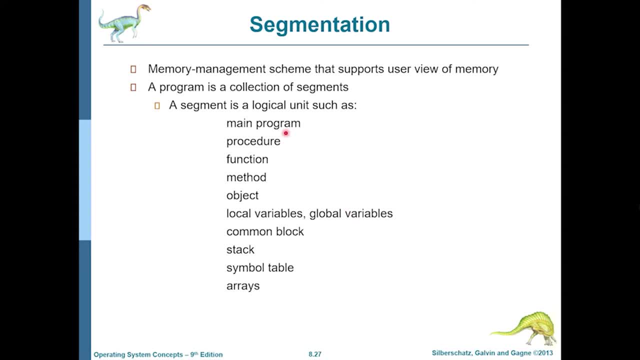 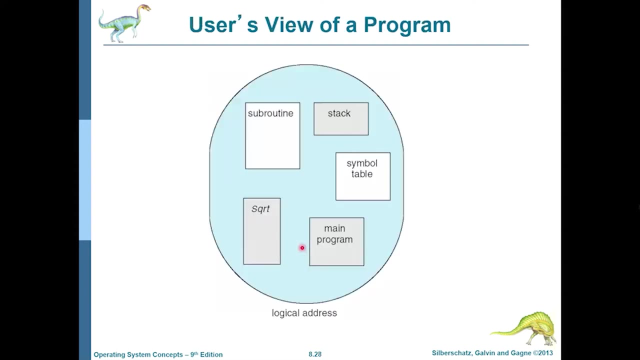 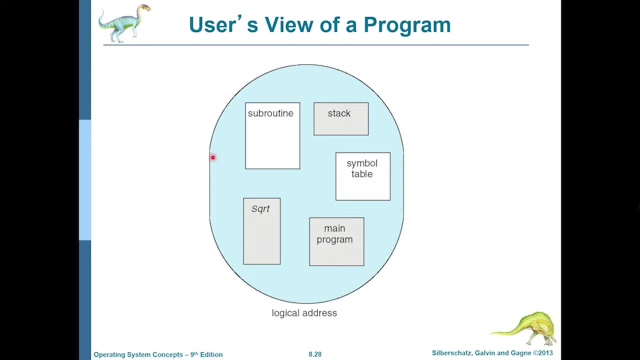 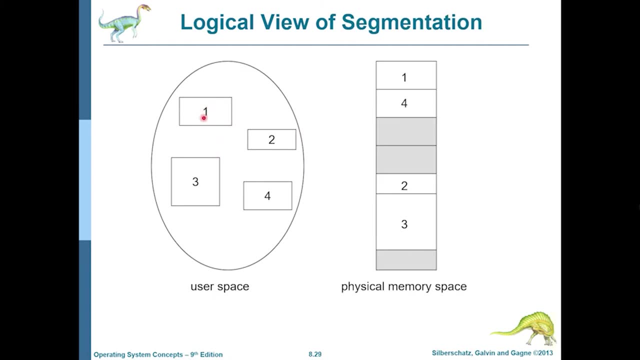 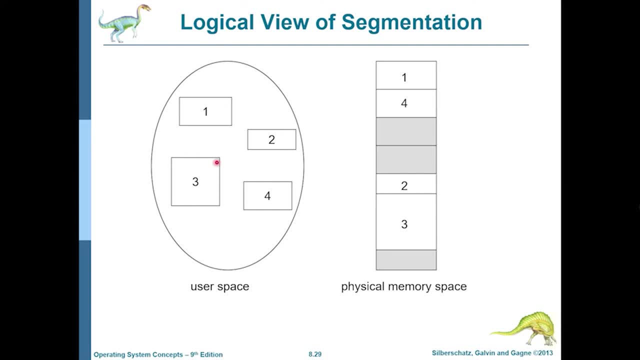 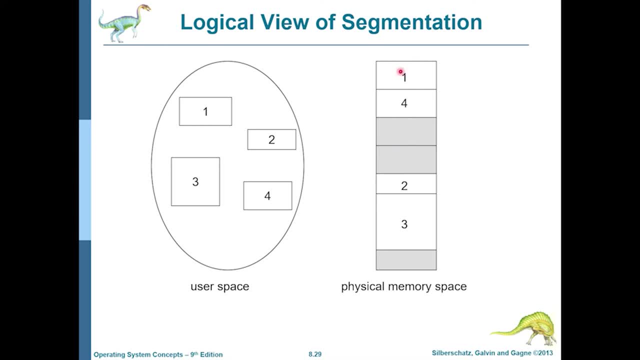 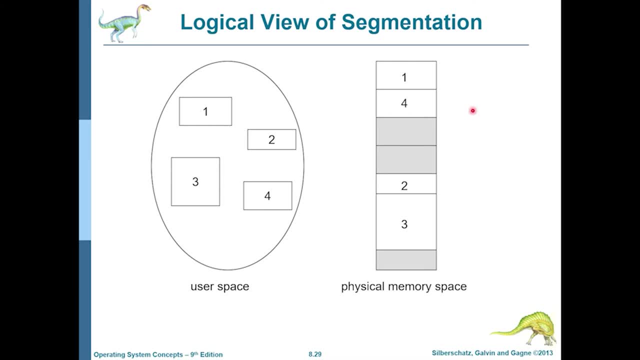 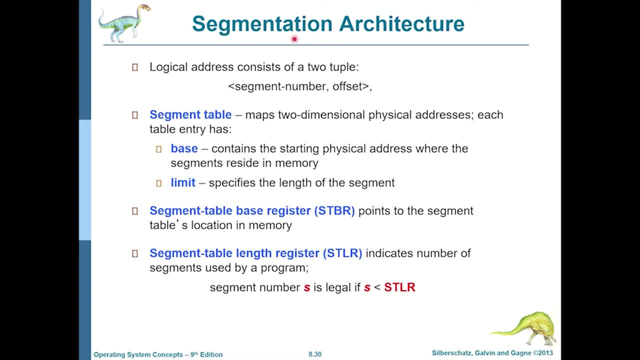 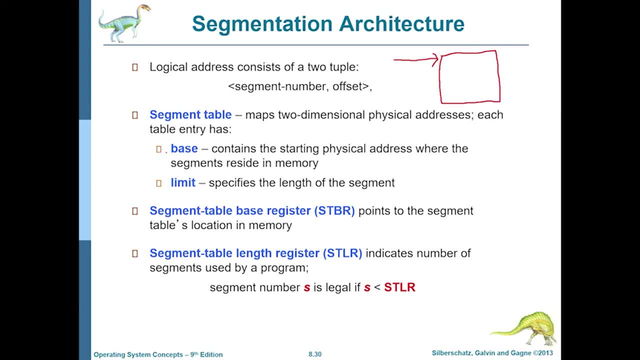 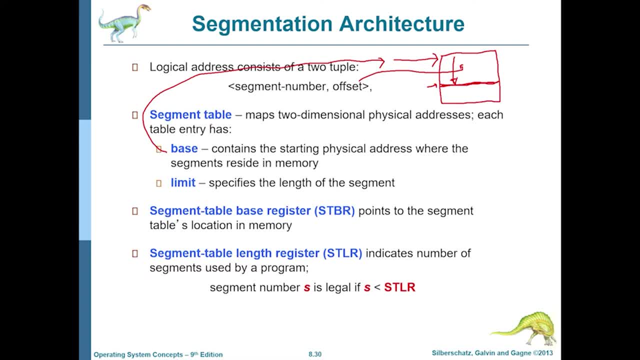 relocation is dynamic, if the operating system can dynamically reb the addresses of two so that it can run properly at its new location. so if relocation is dynamic, if memory address is, and that is how we can convert a logical address to a physical address. so, as already mentioned, so the segment number can be used to look into a segment table. now. 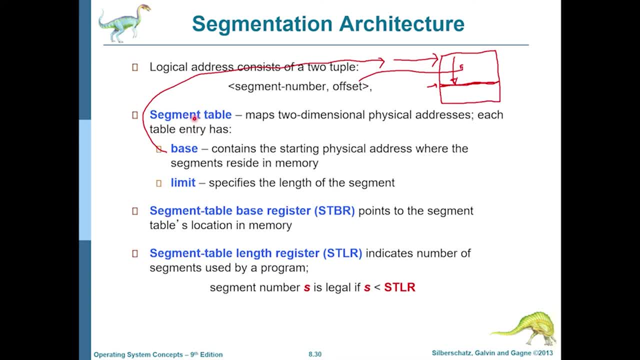 the operating system maintains a segment table somewhere and the operating system knows where the segment table is because that is stored in the segment table base register. so the segment table base register will give you the location of the segment table. you will use the segment number to look into this table to figure out this segment's base and its limit. you need to know the limit of. 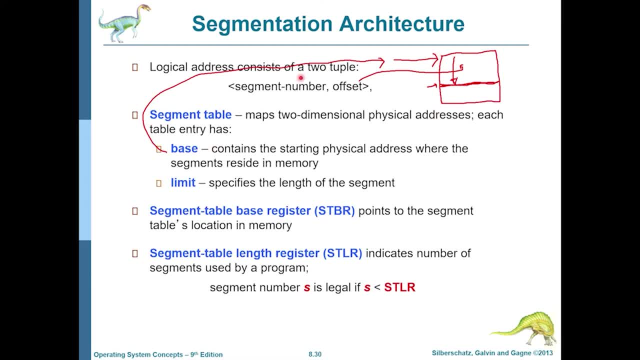 the segment, the maximum size of this segment. then, once you have figured out the base, you can then take this offset and then look into the segment to find out where, in physical memory, your logical address is. and that's how you can convert a logical address to a physical address and that's how you 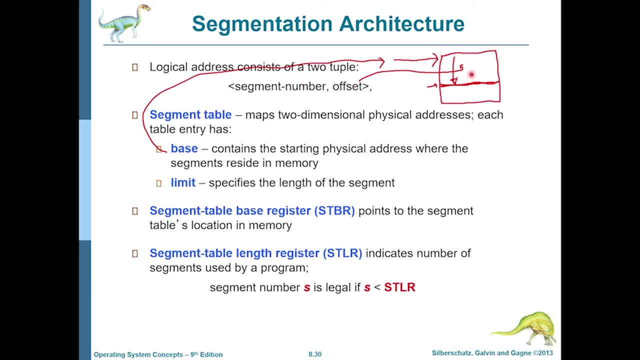 can take a logical address to a physical address. so this is how we can take a logical address and convert it into a physical address. there is also a segment table length register, stlr, which is basically used for protection purposes. again. now i might say process number two. 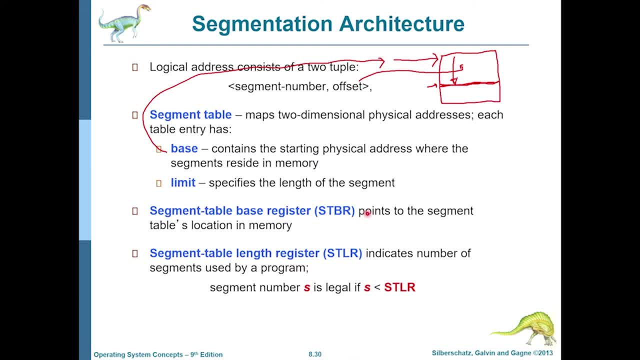 can only use three segments: segment number zero, one and two. so if it generates a logical address, which which is an address in segment number five, then stlr might say no. the maximum number of segments that you are allowed is three. so you cannot go to segment number five because 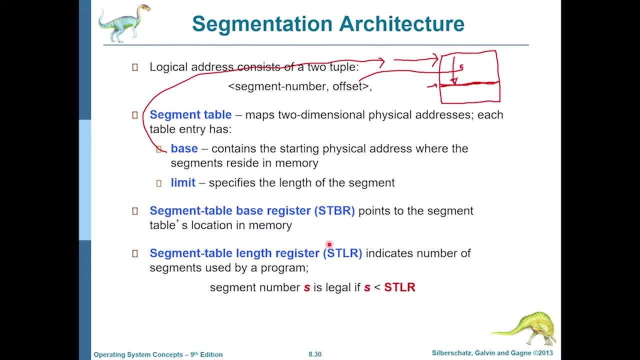 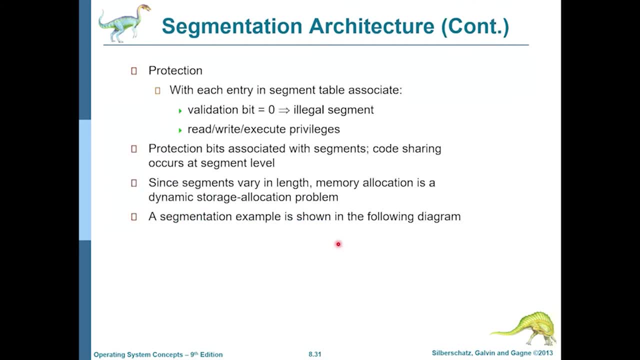 that is outside your reach and that can be used to generate traps, and it is for extra protection. now, protection is not only guaranteed by the segment table length register. as we saw here, we also have validation bits in segments. if the validation bit for a segment is set to zero in the 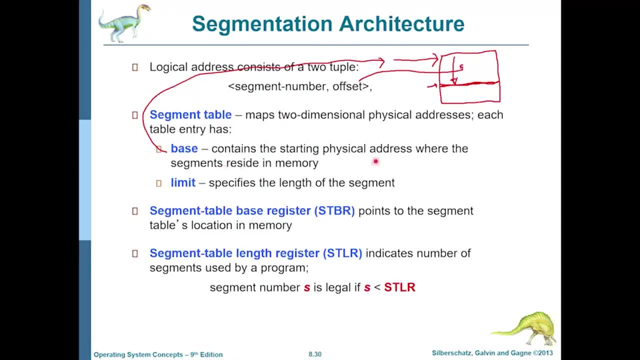 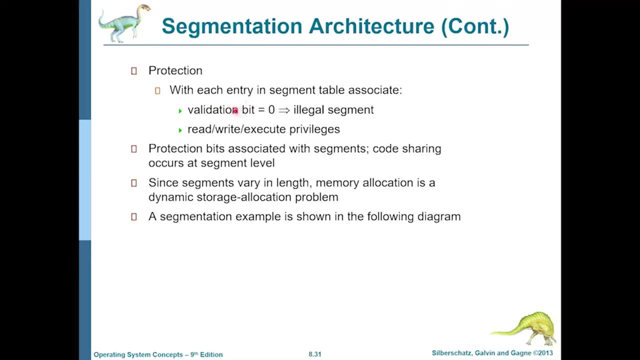 segment table. so in the segment table you will have one entry for each segment and those entries can have different bits on them. one of the bits is the validation bit, which if it is zero, it is an illegal segment and this process cannot access that segment if it is trying to access that segment. 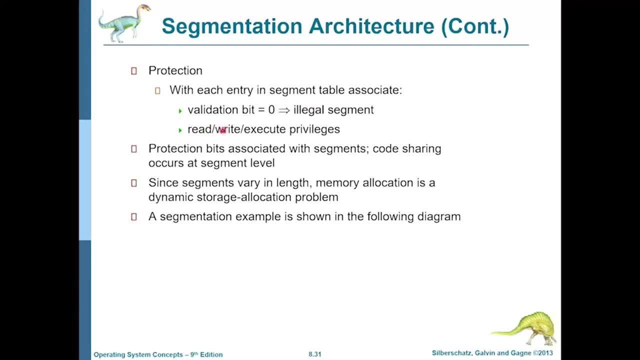 you will get a trap. now the segments can also have read, write and execute privileges. if the program is trying to read from a segment in which the read bit is set, then it is allowed, but if the write bit is not set and if it is trying to write data into that segment, then 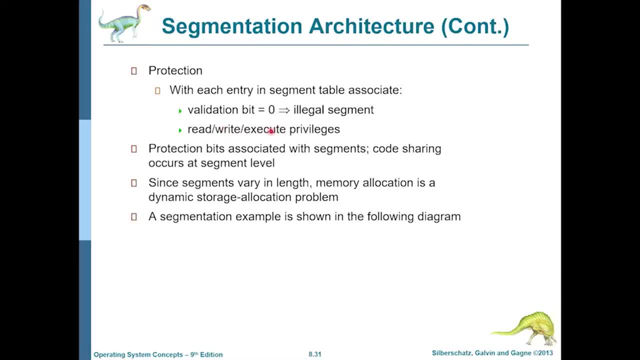 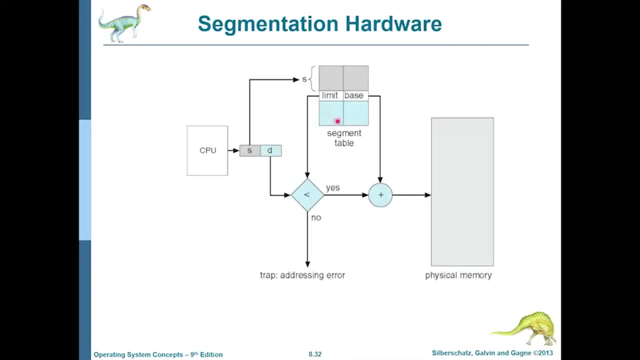 a trap will be generated if it is trying to execute code that is stored in that segment and the execute bit on that segment is not set, then a trap will also be erased. so we will go to the next slide to figure out, uh, how segmentation works in the segmentation. 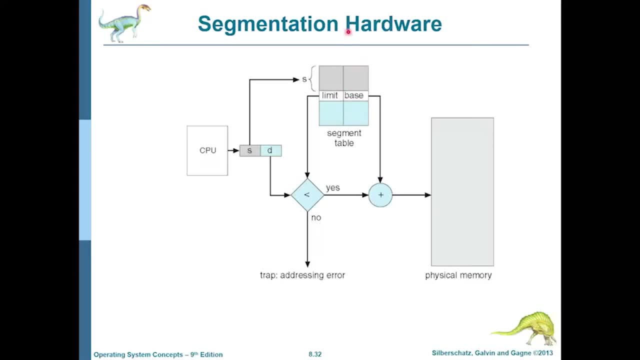 hardware, and i have already talked about most of these things. the cpu generates logical addresses, so the left parts, the most significant parts, will be used to look into a segment table. so the segment table is like this: and since the segment number is s, so we start at the beginning, we go s number. 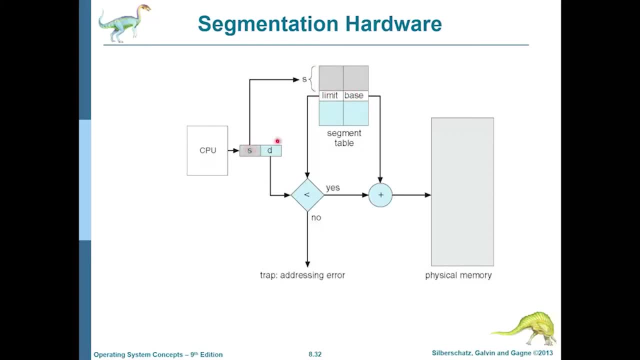 of entries into the segment table because it is segment number s. so this gap is s and we figure out the limit and the base for that segment. and once we know the limit and base, we take the offset address, now the least significant bits on the right side of the logical address. they form the. 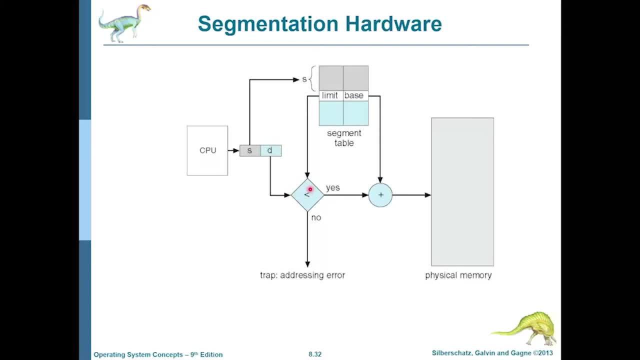 offset. now, if the offset is more than or equal to the limit, then a trap will be generated because you are trying to go outside the segment that way. so the offset has to be strictly less than the limit, and if it is so, then the base of the segment is taken and this offset is added to that and you 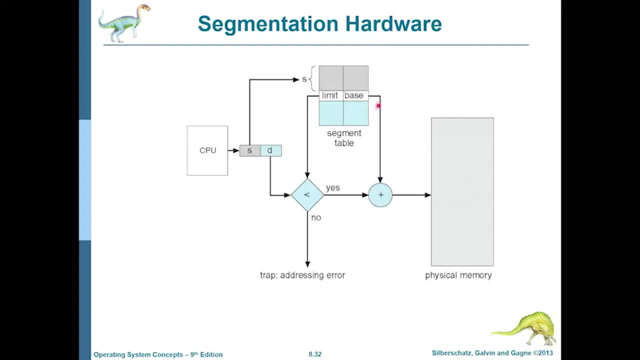 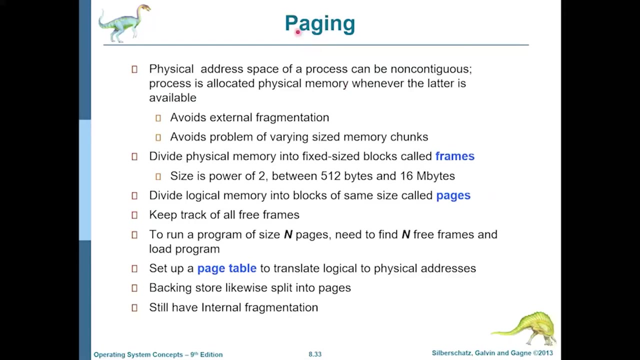 can get your physical memory address that way. so this is the process that we use to convert a logical or a virtual address to a physical address when segmentation is being used. we looked at segmentation. now let's look at the other famous mechanism in which memory can be ordered, and 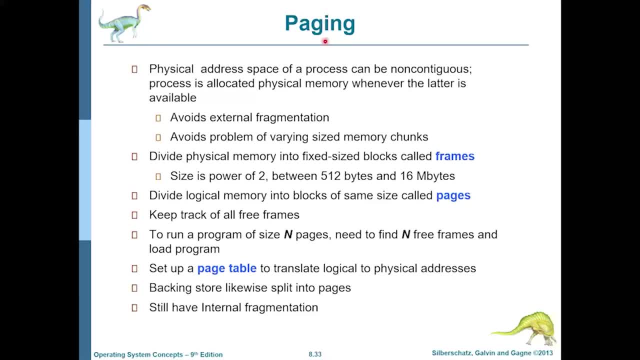 managed. it's called paging. it is very similar to segmentation. in segmentation we could go for non-contiguous physical memory allocation for processes, but each of those segments could be a varying length, so you could still have external fragmentation and all the problems that come with varying sized memory. 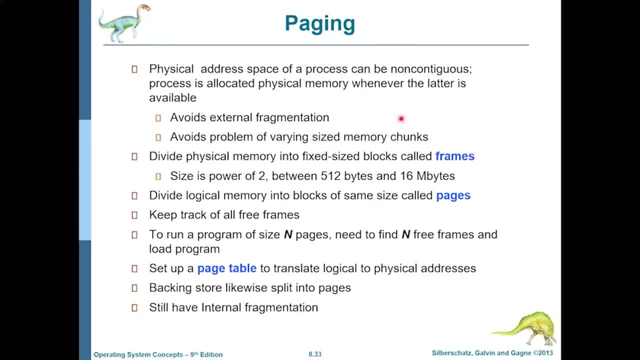 chunks. they all were there in segmentation. but what if we could divide physical memory into fixed sized blocks, called frames, and also divide the logical memory range into blocks of the same size, called pages, and then have a page table in the memory management unit that will map a page in the logical space two frames in the 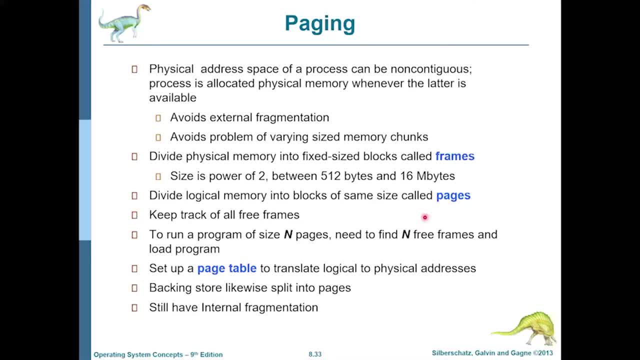 physical space. then we could have allocations where a certain process will not have a contiguous or in order allocation in the physical space but its logical addresses can be contiguous and they can be whatever they want, but there is a page table conversion. if we want to go deeper into the practical applications, we would have to go to the 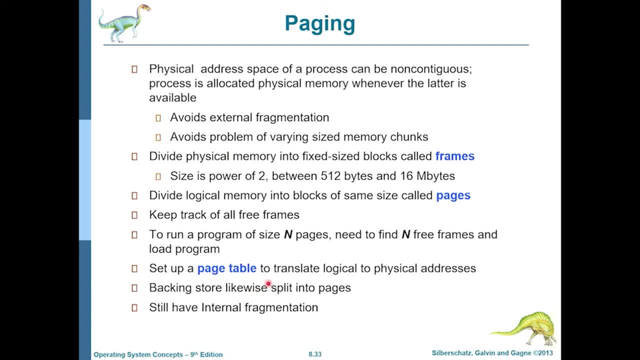 search engine, and what this would do is it will scène automatically and provide us with a map that shows, in the data, Successful programming in the internal fragmentation that can happen in the memory management unit. that will take a page number and it will figure out the frame number and then it can generate physical addresses from logical addresses. now let's look at how that works in the next slide. but before moving on you have to still keep in mind that internal fragmentation can still happen in paging. now, what is internal fragmentation? we remember that if memory is divided into fixed size partitions, then we can have internal fragmentation within the 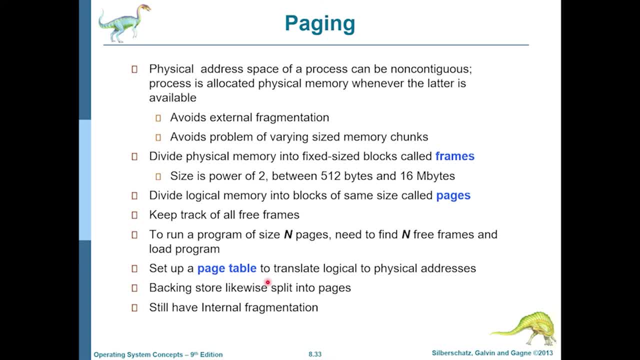 it is not always necessary that the amount of memory you need for a process will be an exact multiple of the block size. so if the process takes, for example, in in paging three pages and there is a little bit of leftover, then it will need four complete pages, even if the fourth 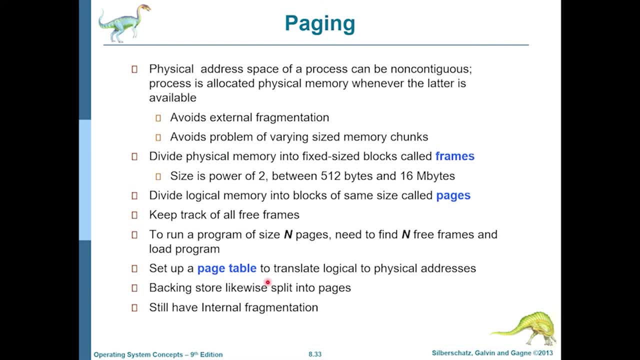 page is not completely full, it will still be allocated to that process and we still have internal fragmentation. it is also important to keep in mind that the frame size is always equal to the page size, that is, the fixed sized blocks into which we divide the physical memory and each. 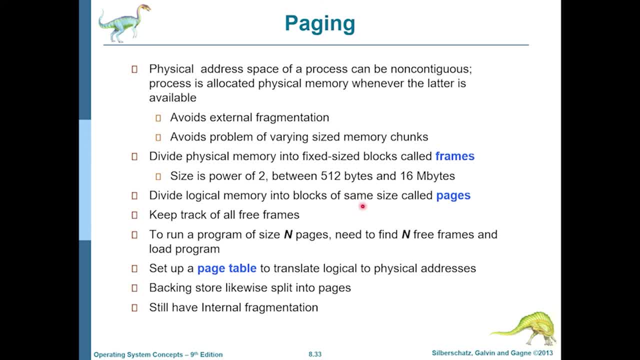 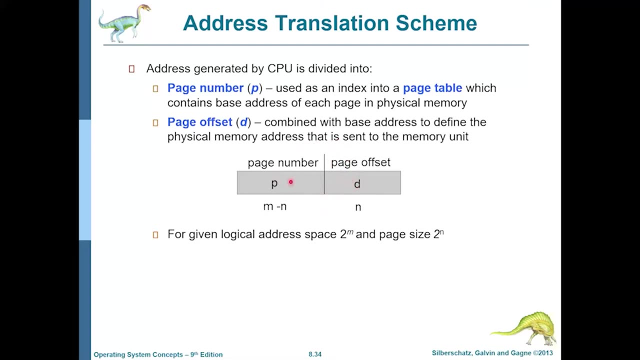 of those blocks is called a frame. then we also divide the logical memory space into pages and the size of each page is equal to the size of each frame. just like in segmentation, in paging also you can divide a logical address into two parts, the most significant bits, that is p denoted over here. 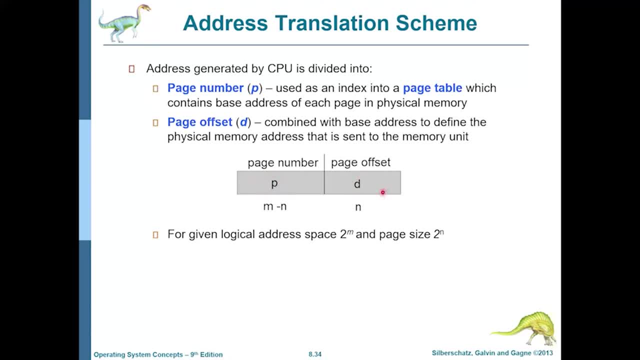 that can be the page number and the least significant bits can be the page offset. we have n number of bits to signify the page offset and m minus n number of bit to signify the page number. the total number of bits is obviously m, and m bits are enough to specify all addresses in the 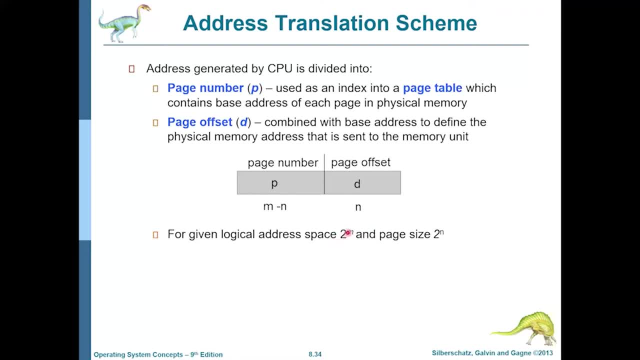 logical address space. so we have two to the power m as the size of the logical address space. and since n bits are enough to specify page, all page offsets, then the size of a single page would be two to the power n. so once we decide on a page number, then we try to find where inside the page the 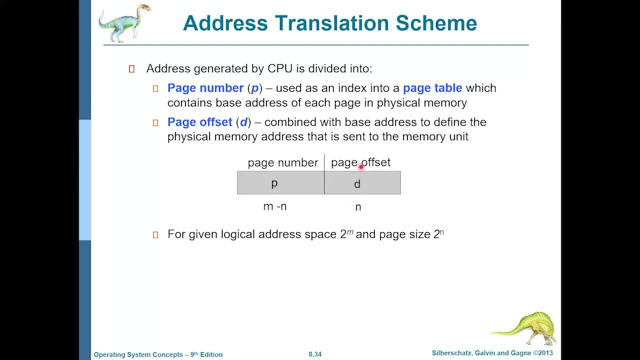 memory location edge. and then if we have n bits to specify the page offset, then obviously the size of a page is two to the power n. the page number of bits is also n. the size of a page is also m. so if we have an image of a page, 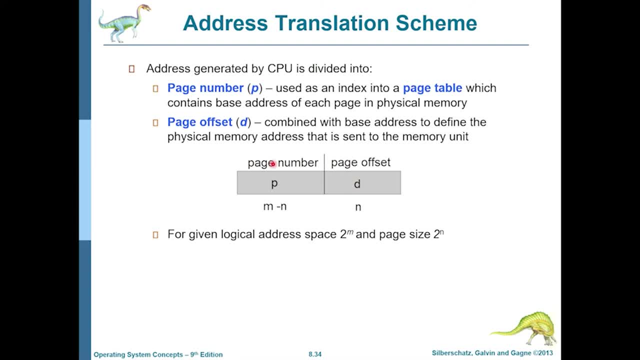 then we have m minus n bits as the size of the page. so actually what we have is a table and we have m minus n bits for the page number. so if we have a table where there are page table entries which specify information about a page, then how many entries will that page table have? it will. 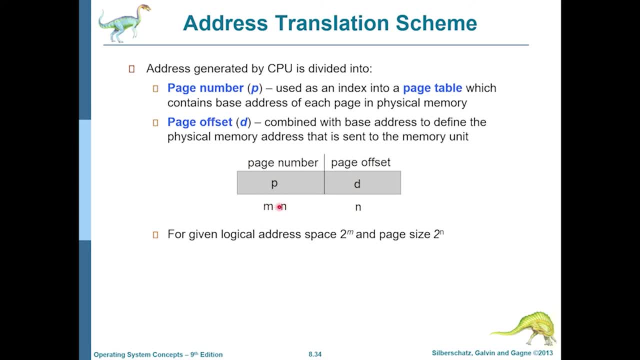 have 2 to the power, m minus n at the top, because m minus n bits are used to signify page numbers. so pages, as in where the page begins, whether the page is valid, whether we can read, write, execute- different things that we saw for segmentation, different things that were there in the 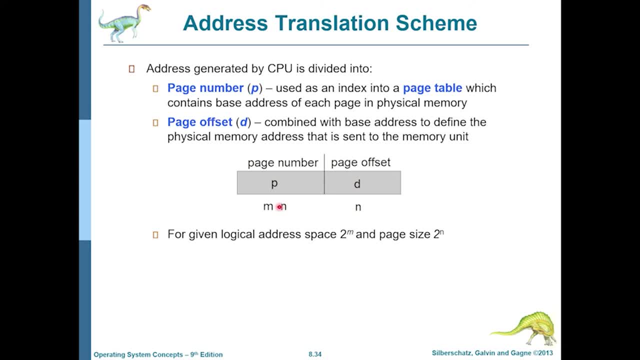 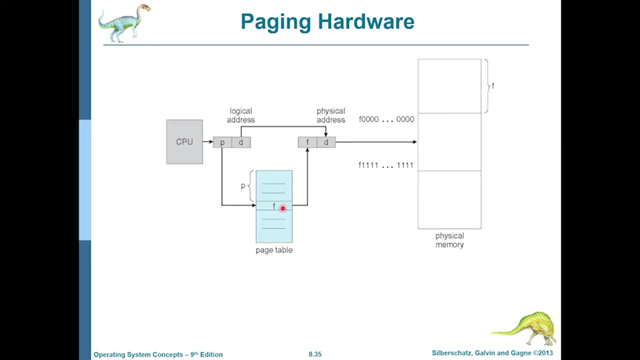 segment table entries. similar things can be there in page table entries, and page table entries go into page tables, and if m minus n bits are used to signify page numbers, there can be two to the m minus n entries in a page table. so here you can look at the entire process very, very clearly. 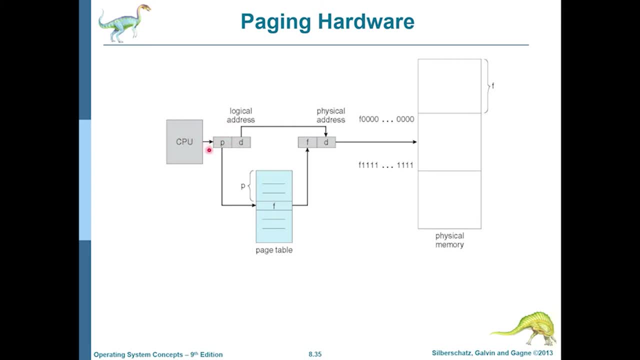 so the cpu generates a logical address and the logical address is split into two parts, where this is the page offset and this is the page number. the page number is used to look at page information inside a page table. since we are looking at the p number page entry, so we get into. 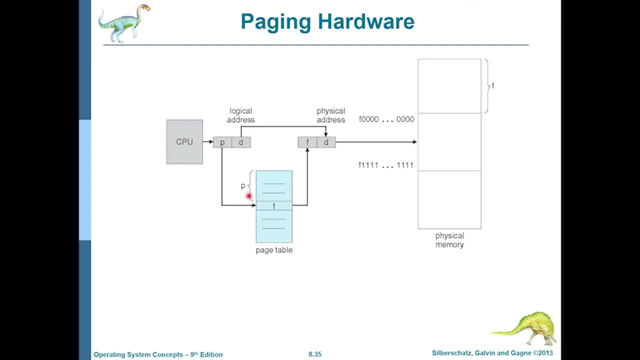 p entries into the page table. so this distance is p. so once we have found the pth page table entry, we figure out the frame number as in: in which frame of physical memory is this page mapped to? as we know, we can have pages in logical address space and we can have frames in the physical 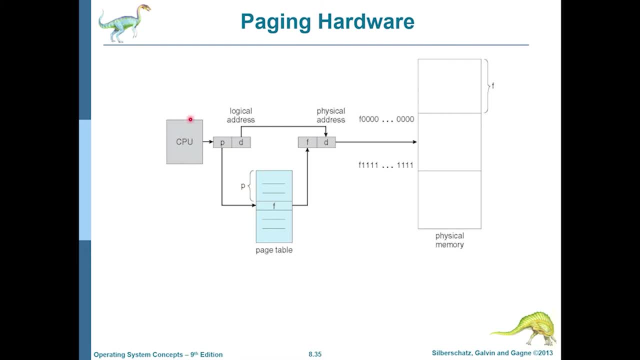 address space and it is the job of the page table to map a page to a frame. so basically we find the page number from the logical address. we look into a page table, we look at the correct page table entry and that is given by p, the page table number, and from the entry we figure out the. 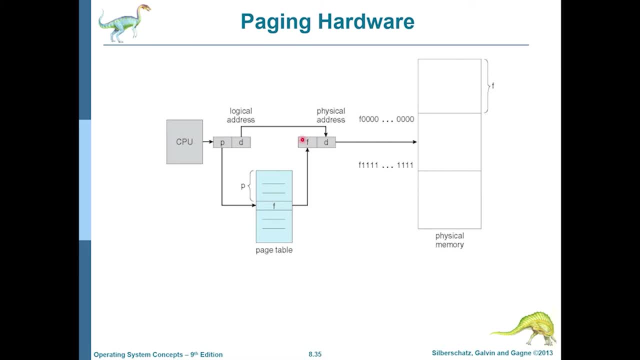 frame number to which this particular page has been mapped by the operating system. then we replace p by f and this is the frame number and the offset just remains the same, because the size of a page is equal to the size of a frame. so whatever this distance or whatever offset into a page, this logical address is in physical address space. it would be the same. 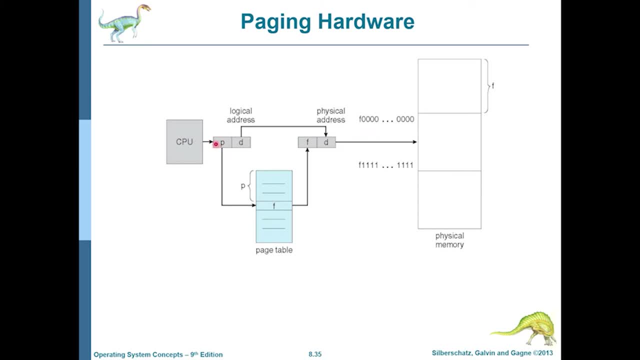 offset inside a frame. so we just replace p with f and the information about f is given by the page table inside a page table entry. so we look at the page number, we go to the correct page table entry, we figure out the frame number and we replace p by f and the offset remains the same. now this logical address has. 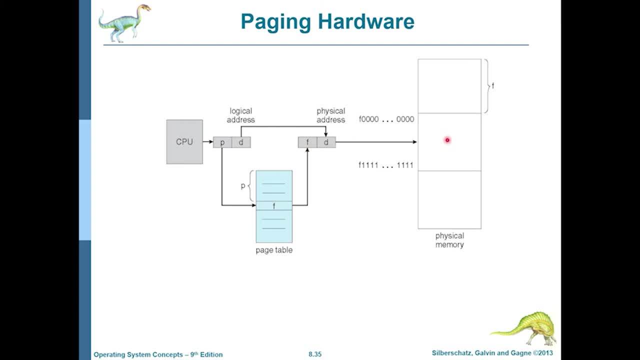 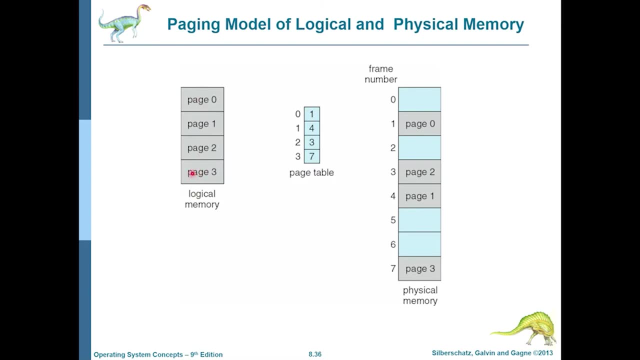 been converted into a physical address. now we can go read and write in our physical memory. here is an example. so our logical memory has been divided into four pages: page 0, page 1, page 2 and page 3, and here is a page table. so we 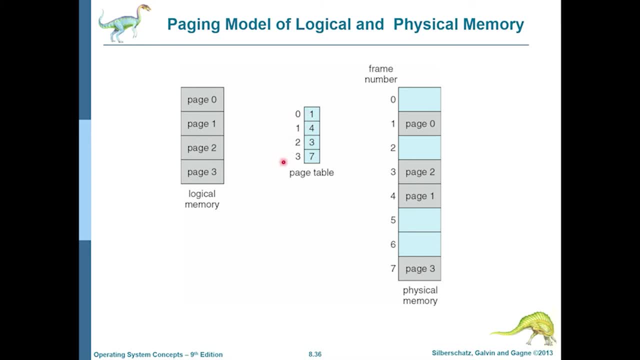 have page table entries for page 0, page 1, page 2, page 3 and these are the frame numbers that are mapped in the page table. so for page number 0 we look at entry number 0 and the frame number is 1. so we go to frame number 1 and we see in physical memory page number 0 is present right here for 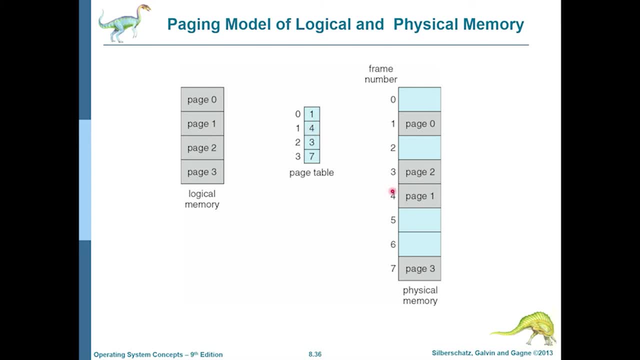 page number 1 the frame number is 4. so we go to frame number 4 and we see page number 1 is mapped right there. similarly, for page number 2, the mapping is at frame number 3 and page number 2 is right there. for page number 3, the mapping is at frame number 7 and page number 3 is right there. 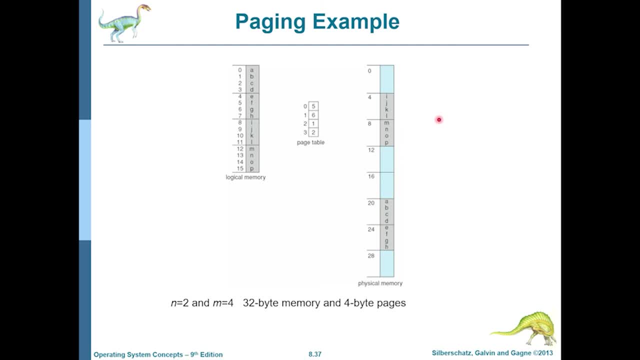 in frame number 7 in physical memory. this is another, more involved example of a page table. here we have n equal to 2. now what does that mean? that means that the page size is 2 to the power 2, which is 4, so, as you can see, each page has. 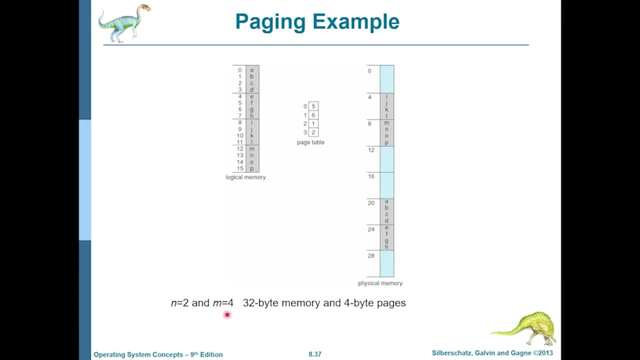 4 bytes in it and m equal to 4. what does that mean? that means that the logical memory space, its size, is 2 to the power 4, which is 16, and, as you can see, it has 16 entries over here. so how many pages are there? so we have to do m minus n, which is 2, and 2 to the power 2 is. 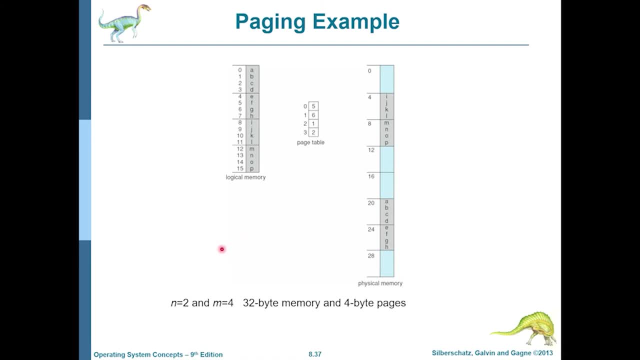 basically 2 to the power m minus n is 4 and we have 4 pages and, as you can see, the page table has 4 entries for 4 pages right here. and let's look at the mapping. so this is page number 0 and page. 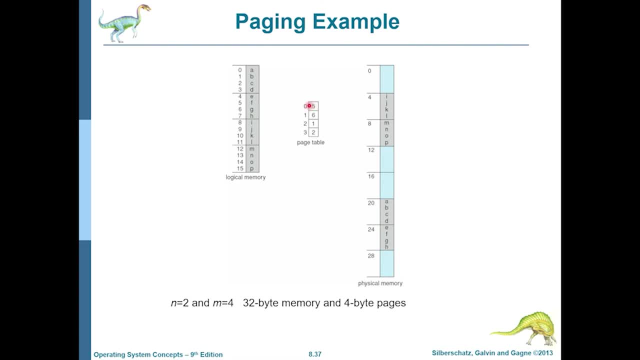 number 0 has a frame number of 5, so let's go to frame number 5. this is frame number 0: 1, 2, 3, 4 and 3 4- 5 and, as you can see, page 0 had a b c d and frame number 5 also has a b c d. and how can you? 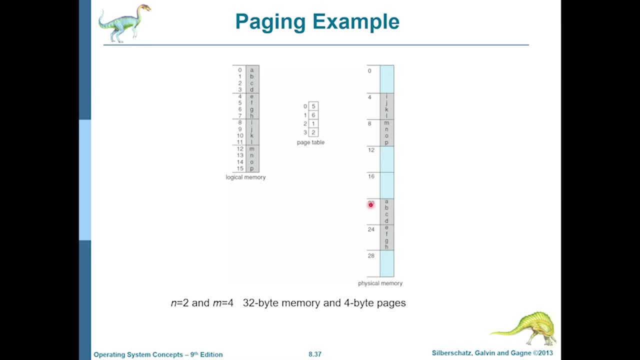 easily know that this is frame number 20. well, what you do is you basically get the frame number and multiply it with the size of a page, since the size of a page is also equal to the size of a frame, and that is 4. you multiply 5 with 4 and you get 20, which is the physical memory address of the base. 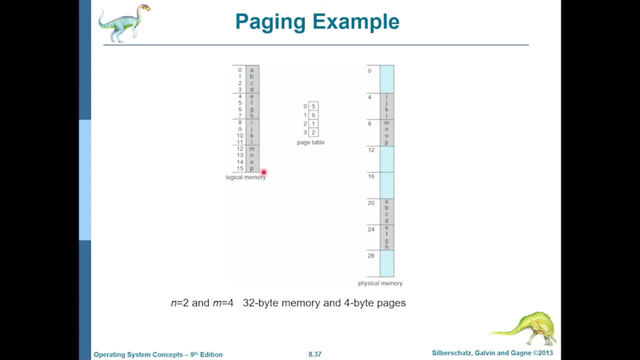 of that frame. let's just do one more. page number 3's frame number is 2. we multiply 2 with 4 and we get 8, and, as you can see, the contents of page number 3, which is m n o p, is present right here in frame. 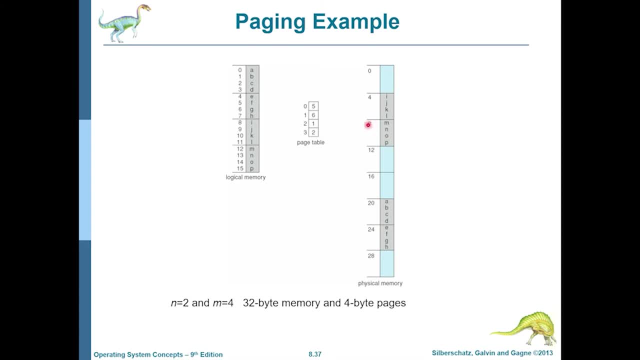 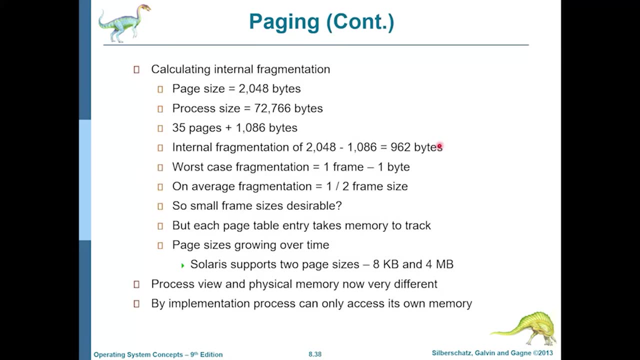 number 2, which begins at address 8, because 8 is equal to 2- into 4 m n o p is right there. i said that internal fragmentation is still possible in paging and let's see how that is possible. so the page size is 2048 bytes and the process size 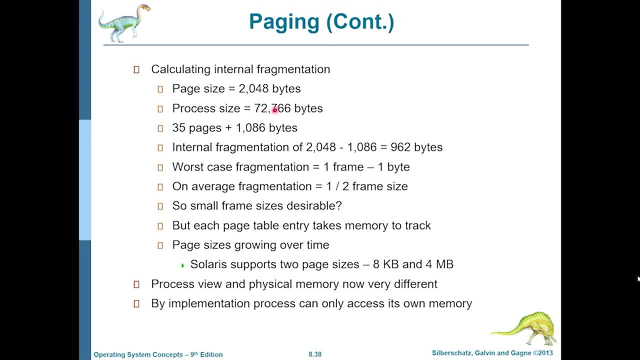 is 72766 bytes, so this is exactly equal to 35 pages, 35 into 2048, plus these 1086 bytes extra. so how many pages do you need? you need 36 pages. even if the last page is not going to be completely occupied, you still need it. and what is the internal fragmentation? the last page had space for. 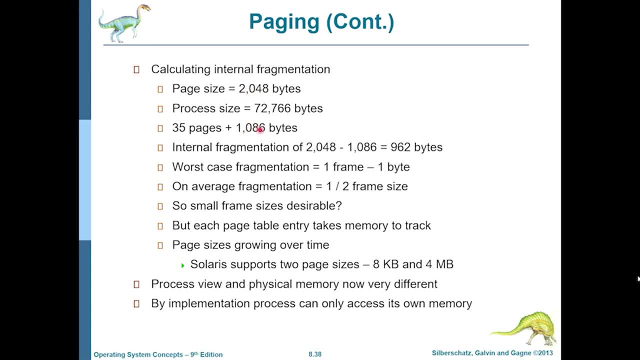 2048 bytes. you are only using 1086 bytes, so we have a wastage of 962 bytes. the worst case fragmentation can be. just imagine if this process had 35 pages and just one byte left over here. for that one byte we would have to take an entire frame of memory, an entire page of memory. that would be. 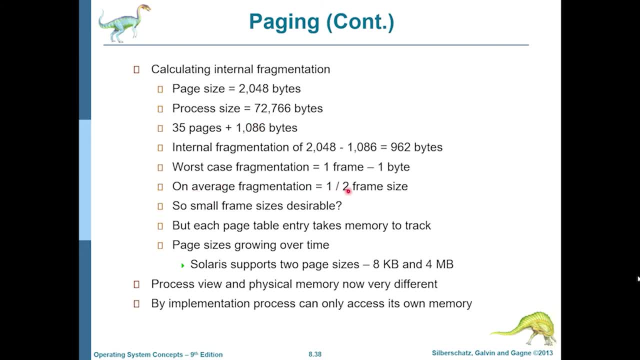 the worst case. on an average, usually half a frame worth of page is usually lost due to internal fragmentation. so should we just make small frame sizes, because if the here, if the frame size or the page size, because page sizes are equal to frame sizes here, if we have made the page size to, let's just say: 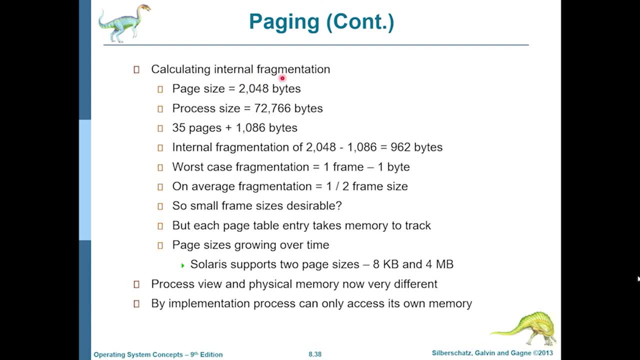 512 bytes, then the fragmentation would have been very, very less, because out of this 1086 bytes, even two pages, 1024 bytes could have gone to two complete pages and only a few bytes would have been left. and and agreed that that would have taken another. 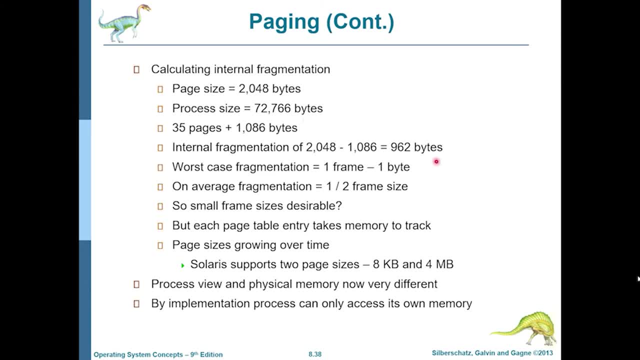 512 bytes of a page, but the loss would not have been as high as 962. but the problems with very small frame sizes is that we need a lot of page table entries. so if you make the page size very, very small. so, as you remember, we had n bits for the page offset and m minus n bits for the page. 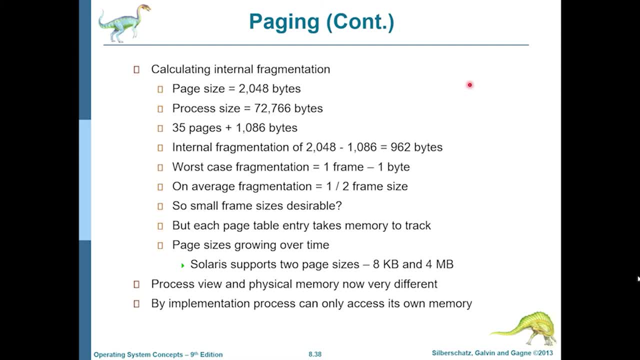 number. so if you make the pages very, very small, then the offset is very, very small. so you don't need those n bits for the offset. so if you make the pages very, very small, then the offset is very. n is small, and let me draw it for you right here. so your logical address is kind of like this: 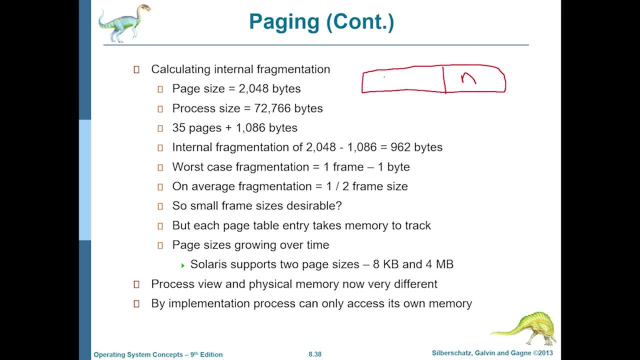 and you have n bits for offset and m minus n bits for the page number, right now, if you have small pages, then this is small, right, so your logical address is still the same size, but your frames are small, so you don't need such a large offset. and this is again m minus n. so what happens here? 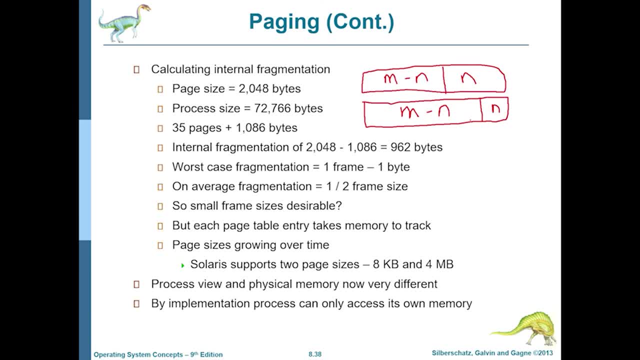 m minus n is bigger. so now you have more page numbers. and when you have more page numbers you need more page table entries in a page table and the page tables can become very, very big. in fact, modern operating systems and modern hardware prefer to use bigger pages because fragmentation 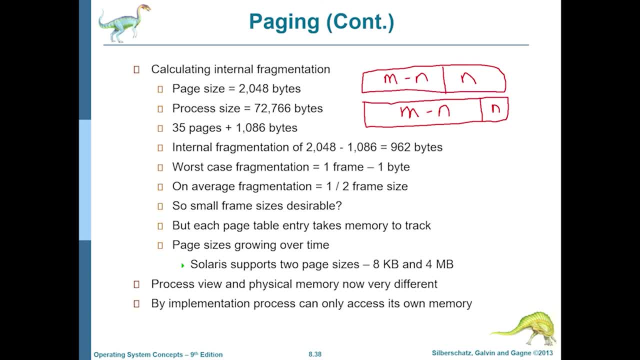 is there, but these days you don't need such a large offset, and this is again m minus n. so what happens here? m minus n. ram is very, very cheap, so to avoid the maintenance cost of so many page table entries. operating systems are usually okay with loss of memory due to internal fragmentation, but they try. 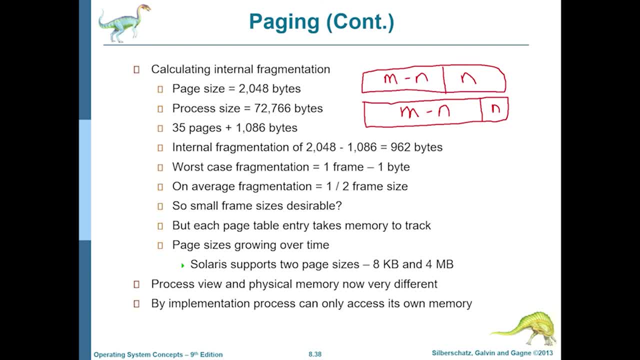 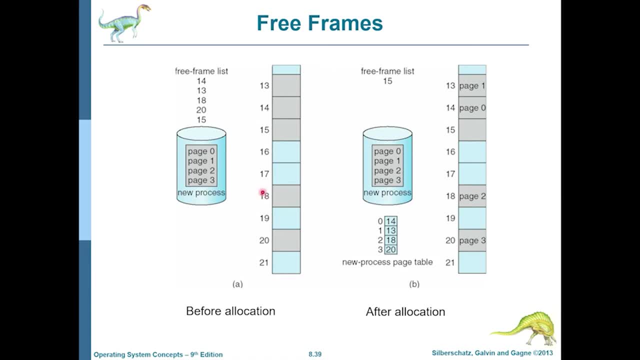 to get as much as possible out of the efficiency gains in having less number of page table entries. now let's look at the concept of free frames. so the operating system has to maintain a list of free frames in physical memory. it is only then that it would be able to allocate those frames. 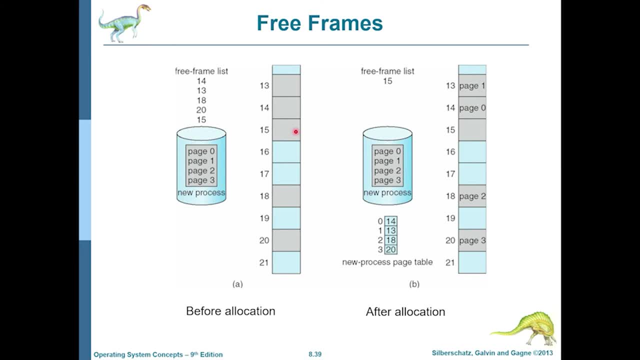 to pages for a new process and then map them in a page table. so before allocation, the operating system had all these frames free and a new process comes in which needs four frames. now, before allocation, physical memory used to look like this. after allocation, the process is there. 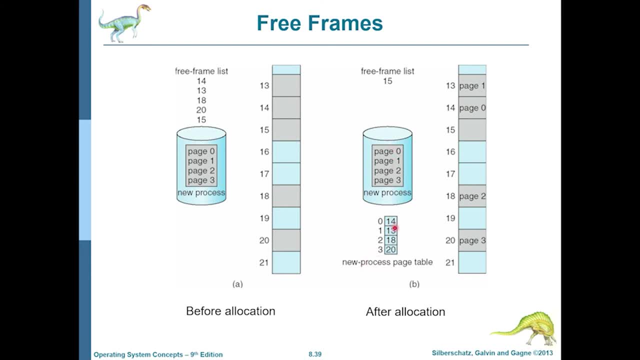 in memory right now and we have a new process page table. page number zero has gone to frame number 14 in physical memory. page number one has gone to frame number 13, page number two has gone to frame number 18 and page number three has gone to frame number 20. as you can see those. 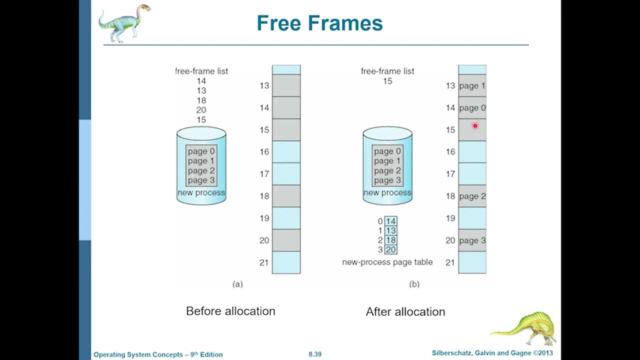 allocations have been done here. they are not contiguous, they are not in order, and that is basically what paging is and what paging lets you do. and now the free frame list is shorter because four frames are gone and only one frame, that is frame number 15, is free at this point of. 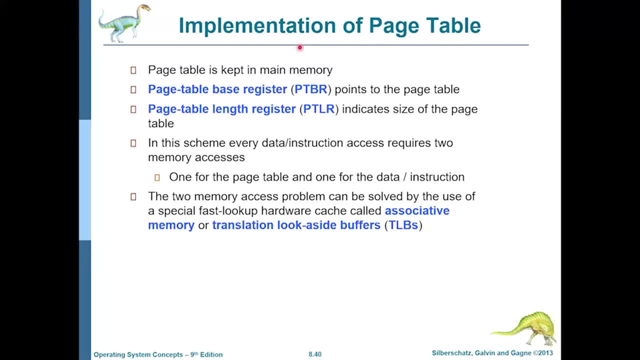 time. just like in segmentation, like the segment table used to be kept in memory somewhere, page tables are also kept in main memory and the location of the page table is usually given by something called a page table base register. and there is also something called a page table length register which can be used for extra protection. so if the logical address says: 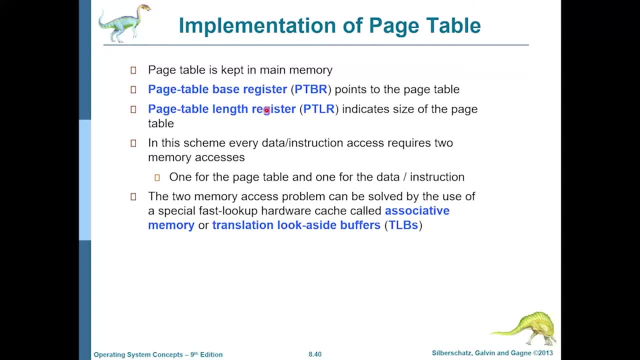 that i need a very high page number which is not allocated to the process, then the operating system can raise a trap. we saw similar concepts in segmentation also. so every memory access by the page table needs to go through two accesses. one is the access into the page table, so that it knows. 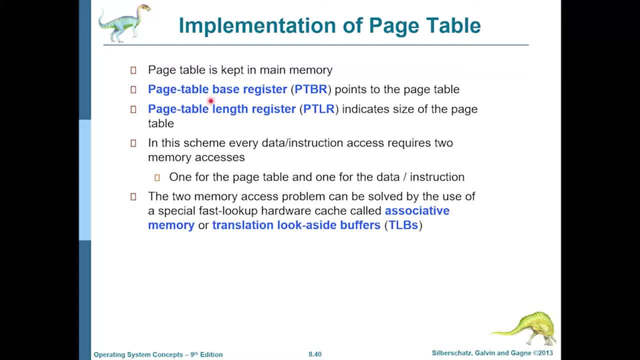 which frame to go to in physical memory. and then, once it knows the physical address, then the actual access into ram or physical memory has to happen. then it has to come back to the process now. how do we avoid two accesses? well, just like in cpus, we used caches right. so we used to first go to the 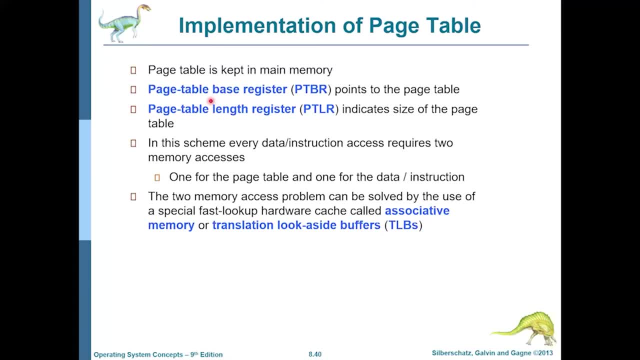 cache to see if something is present. if it is not present, only then we would go to main memory. just like that, we could use something called associative memory or translation. look aside buffers- they are called tlbs, and this is a very important concept in operating systems. so what the system can do is first go and look inside translation. look aside. 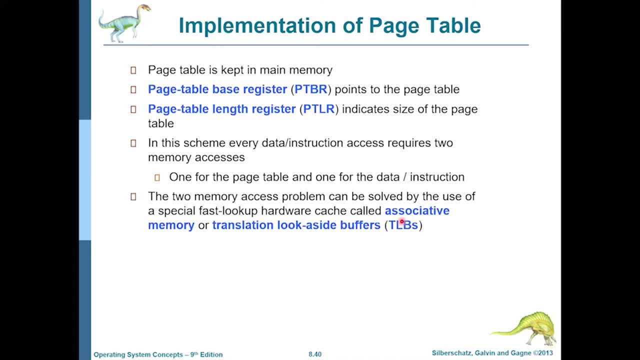 buffers to see if a certain page table mapping is present in those tlbs. if it is present, then it will find the frame number from that tlb and directly go to physical memory and get its data or store the data. if it is not present in the tlb, 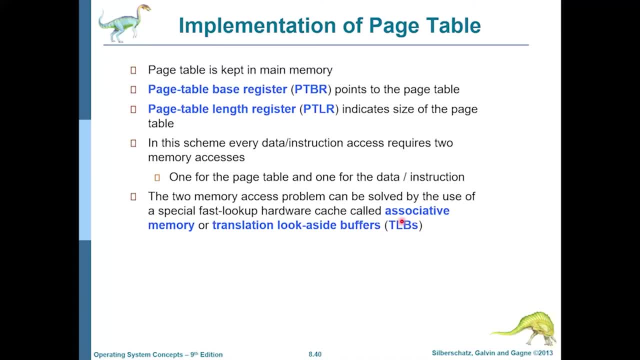 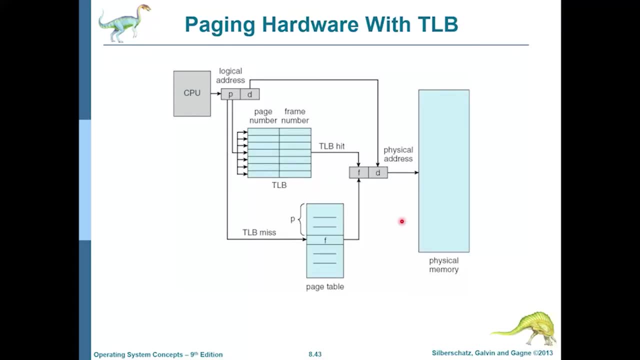 then the page table and memory will be consulted and then it will go on from there. so in the next slide we will see, using a diagram, how this works. so this is an example of a tlb, a translation, look aside- buffer. so when a cpu generates a logical address, the address is split into two parts as 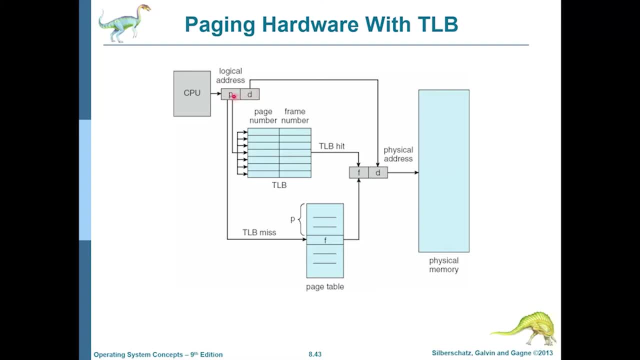 we know there is a page number and there is an offset. now the page number is first sent into a tlb and these comparisons happen parallelly. we don't go one by one, we don't go linearly, because that would be very, very wasteful and it might take a lot of. 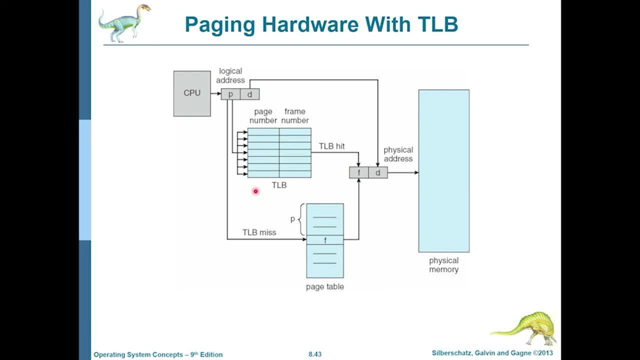 time. memory accesses have to be done extremely fast. you cannot afford to take so long to do a single memory access. that is why these kinds of memories are called associative memories, as in the access into the different cells of these memories can be done simultaneously, that is, parallelly. so all the entries here are search to see if this page, number p, is present. 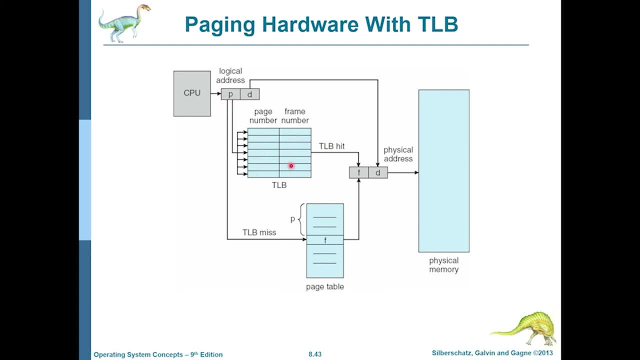 if it is present, then it is called a tlb hit. we immediately get the frame number. now we know f, so we have removed p and we put f into the logical address. the offset remains the same and we go to physical memory. if there is a tlb miss, if this page number is not present in this tlb, then as 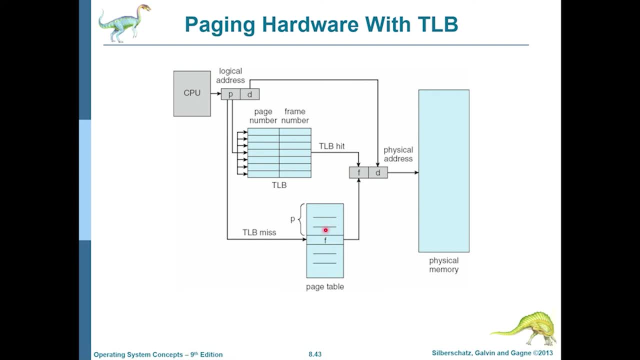 usual, we look into the page table, which is again in main memory somewhere. we figure out the frame number. this is slower but we still have to do it because it was not present in the tlb now. we figure out the frame number and we go to the physical address space to get the data or store. 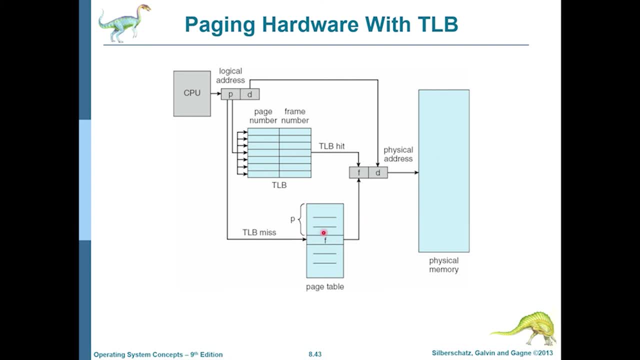 the data and we also try to put the value of f into the tlb because it is very likely that the next access is also going to happen inside the same page. so if there is one tlb miss, next time around that same tlb miss should not happen. 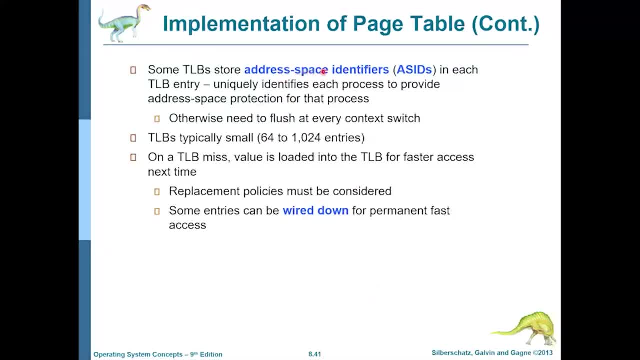 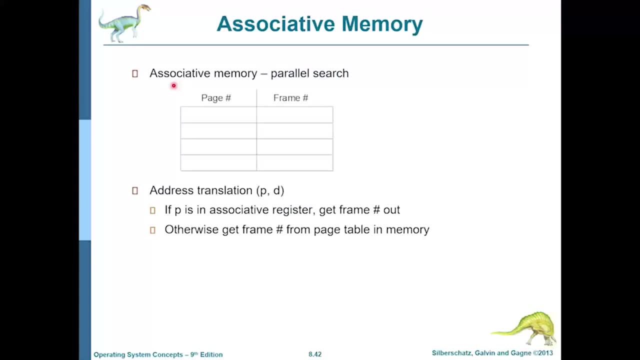 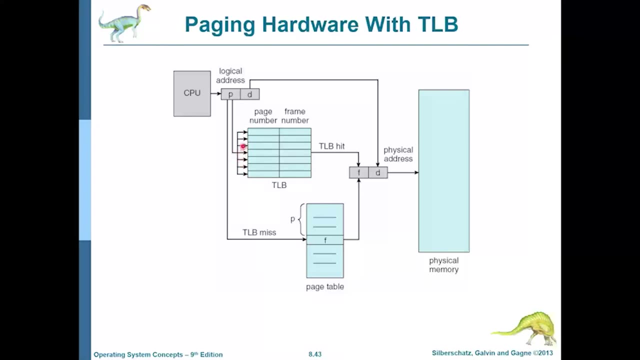 sometimes tlb's also store address space identifiers, called assets, in each tlb entry. so just imagine something like this: so over here we can store some assets also. so why is that necessary? just imagine one process is running and that process has its own mapping from pages to frames. now 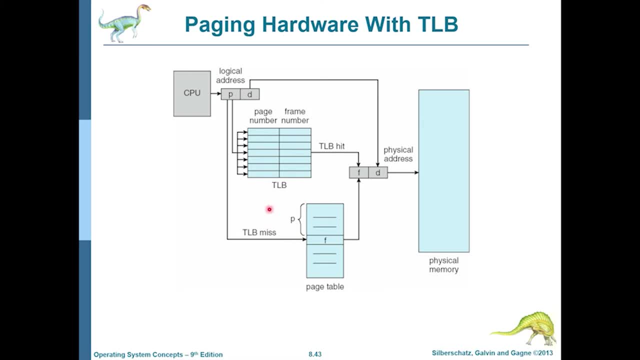 if that process stops running and another process starts running, whatever stale entries, the old entries in tlb that are there, those will not work correctly for the new process. so for example, both processes can have their page number zeros mapped to different frames right in physical memory. now over here, if we have page number zero, 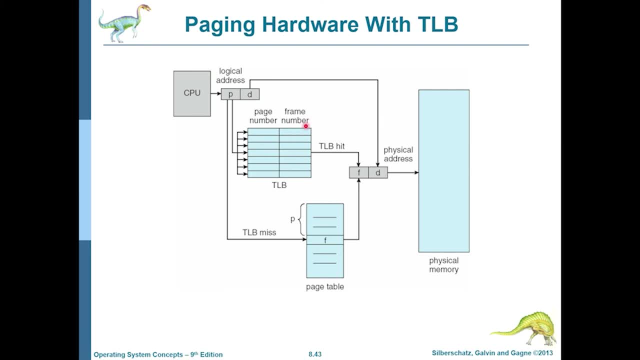 is mapped to frame number 15 for process one. now if a context switch happens and process two comes in, so that process's page number zero might be mapped to frame number 20 in physical memory. but the tlb entry over here has the entry for the first process, process one, which says: 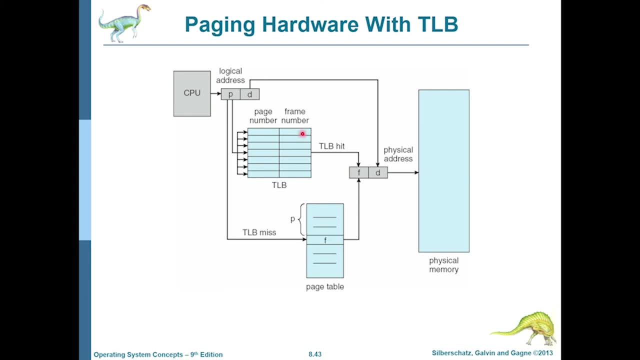 page number zero is mapped to frame number 15. so if you look at the tlb for the second process using the entries of the first process, you will go to the incorrect physical address frames. that is why if you do not store address space identifier over here, which are basically described here, then what will happen is that for every context switch, 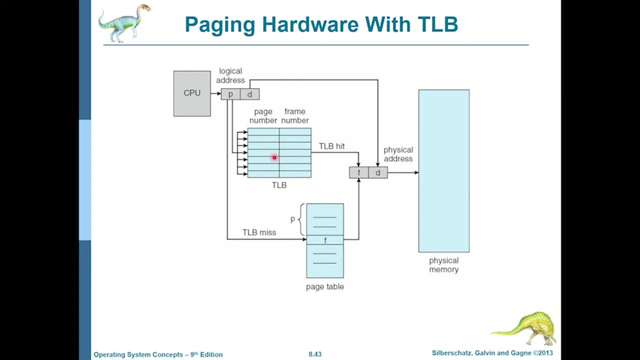 you'd have to flush the tlb. if a new process comes in, this entire tlb has to be flushed and as and when tlb misses happen, the tlb will start getting populated. but if you also store some process specific information in the tlb which says okay, process number one, page number zero, 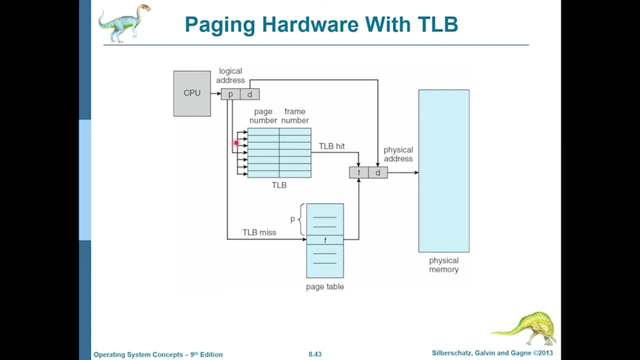 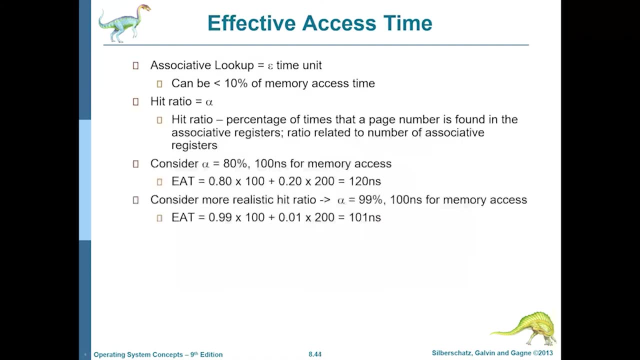 now goes to frame number 15, but process number two, page number zero, goes to frame number 20. then you don't have to flush the tlb for every context switch. now let's look at the concept of effective access time. we know that tlb misses can happen. it is not always that when you try to look for 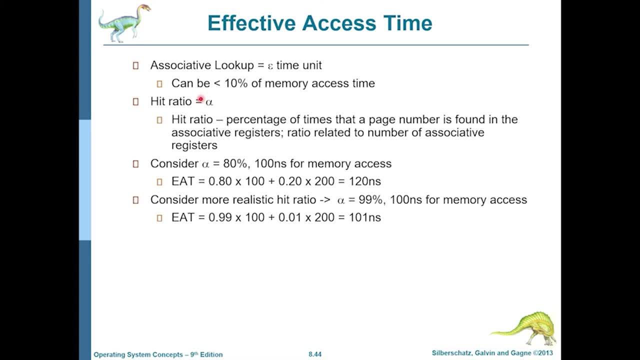 a page table entry inside a tlb that you always find it. so misses do happen. and if a miss happens then you have to go to main memory, you have to go into the real page table and figure out the entry and then go on from there. so we define something called 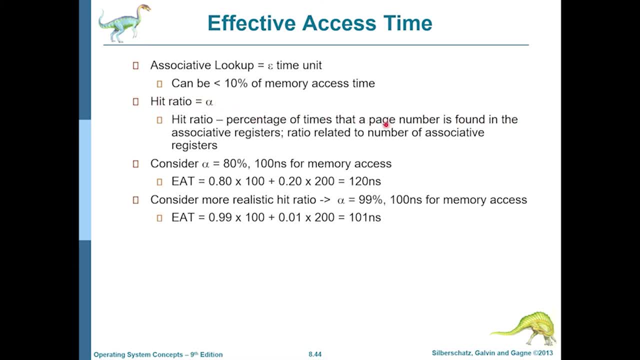 a hit ratio, which is the percentage of times that a page number is found in the tlb, and we take a couple of examples to figure out the effective access time. so if the hit ratio is 0.8, which is 80, and memory access time is 100 nanoseconds, so 80 of the time you can figure. 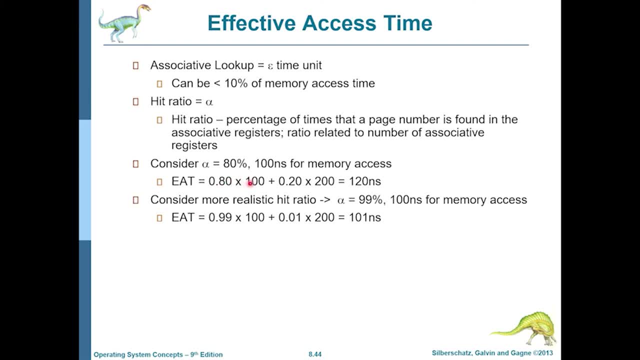 out the page table mapping from a tlb. so you just have to do the real memory access, which is after you get the logical address converted to a physical address, you go to the main memory and get it, and 20 of the time you have to do two memory accesses. that. 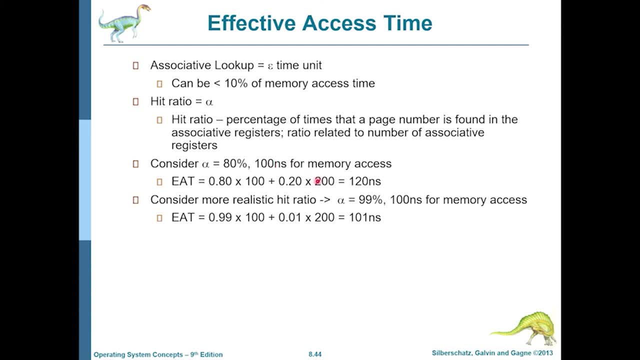 is two into 100 nanoseconds: one time to look at the page table and the second one is the real access. so the effective access time is then 120 nanoseconds. a more realistic hit ratio would be 99, because after the process starts running for a while, all the important page entries actually get. 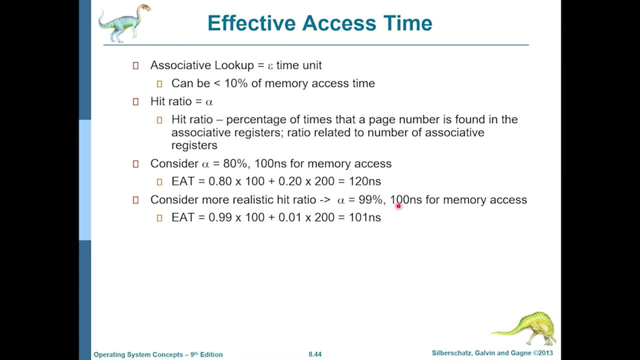 populated into the tlb and the misses become really rare. and for 99 the effective access time is 101 nanosecond, which is very close to that of a single access to memory. so the disadvantage or the extra time that gets introduced because of paging functionality is very, very low, which is 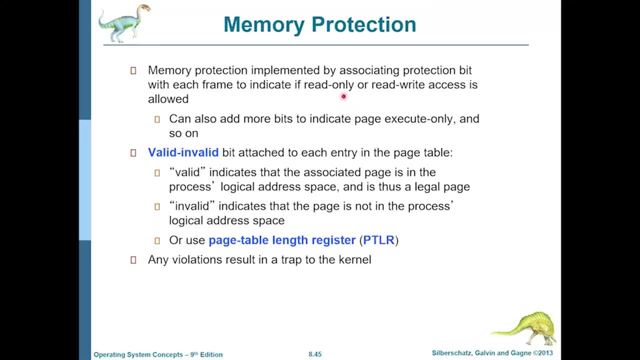 just about one percent. now let's look at how memory protection can be done in paging, just like in segmentation, you can add, read, write, execute bits, valid invalid bits. the same bits can be used in page table entries also, so the page table entries would not only contain the frame number they can. 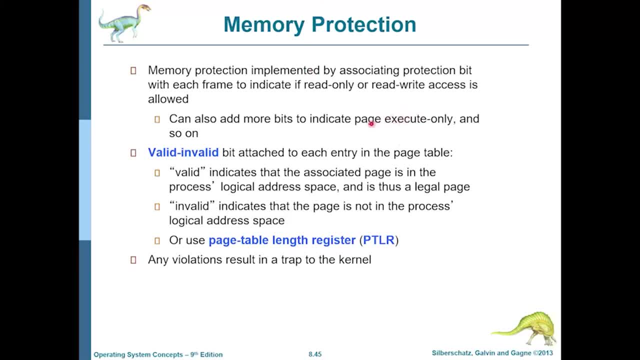 also contain things like the execute- only bit read, only bit read, write whether the page is valid or invalid. so all these bits can provide extra protection. so if there is a page table mapping to a process and the process is not supposed to write to that area, then you can just not have the 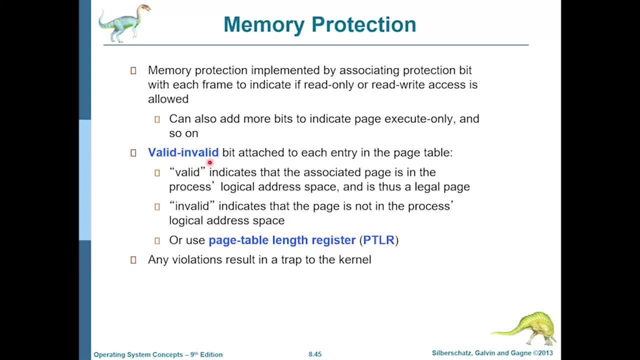 right bit set and then the process will not be able to write to that area. if you have doubts that the contents of a certain area of memory can contain malicious code and you don't want the process to be able to execute anything in that area, then you can set the execute bit of that memory area to false. 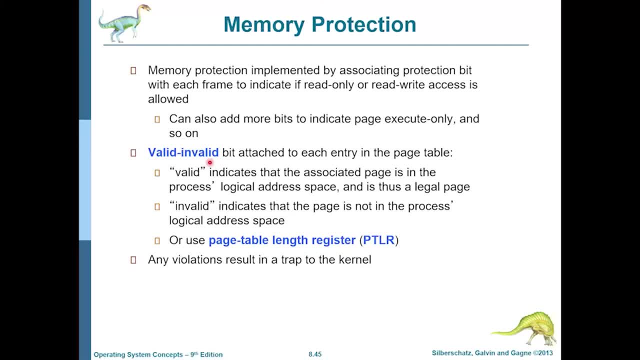 and the process will never be able to execute anything that is located in that memory region. if the valid bit of a page- double entry- is set to invalid, that is, it is not set- then a process will never be able to access, read, write, execute anything from that page. you can use that. 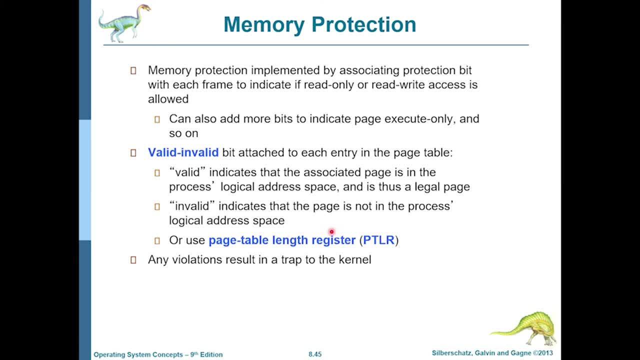 or you can use page table length registers, just like we had segment table length registers. you can also use ptlrs and any violations that occur by lessons, like there is a read only bit set but you're trying to write, or if the execute bit is not set, you're trying to execute. 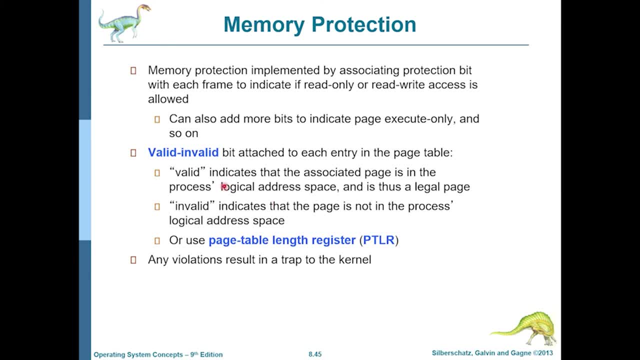 something in that page. any of these violations. you try to access an invalid page or you have gone beyond what is mentioned in the page table length register. you're trying to use a page number which is bigger than what is available in ptlr, then a violation can occur and these are: 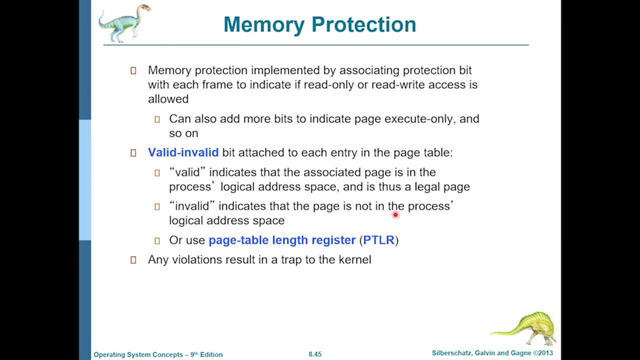 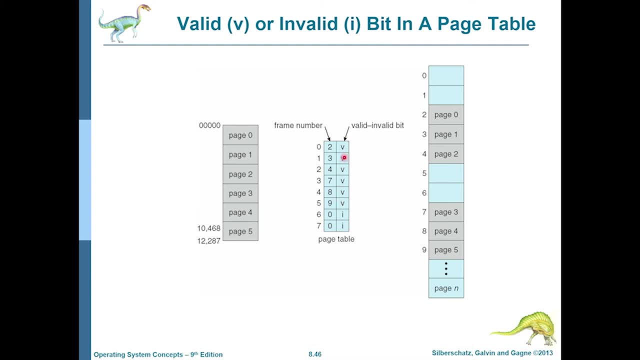 all traps into the kernel and the kernel would know how to handle these. so here is an example of a page table which has each table entries that have the valid and the invalid bits set in these page table entries. here you can see that page table entries zero. 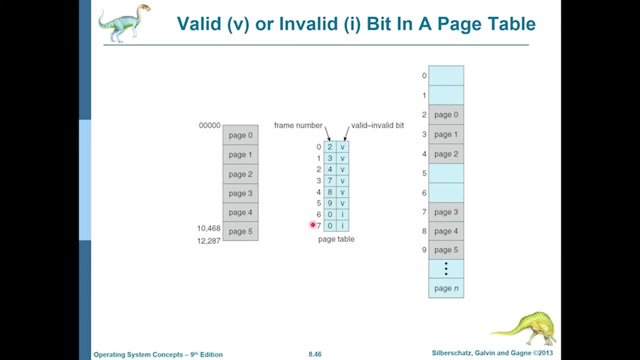 until five are valid, but page table entries six and seven are invalid. so a process can only access memory areas from page number zero to page number five. it cannot go beyond that because those page table entries are marked as invalid. processes can share pages if there is read-only. 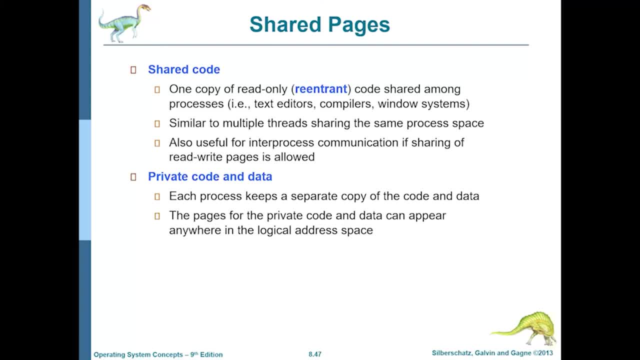 code, then it does not make sense to have that code in more than one physical frame. so there's a lot of. there can be one frame which has that read-only code, and multiple processors that want to run that code can have their pages mapped to the same frame, and so we can call these pages as shared. 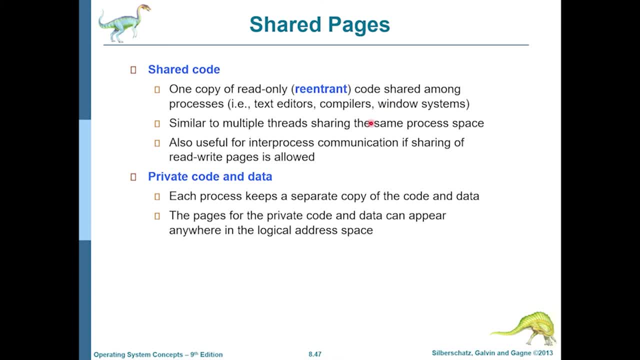 pages. now the shared page does not need to be read, only it could be read and write. and two processors can have two different pages mapped with that same physical frame and they can read and write to that. they can adopt mutual exclusion and use that as their inter-process communication strategy. 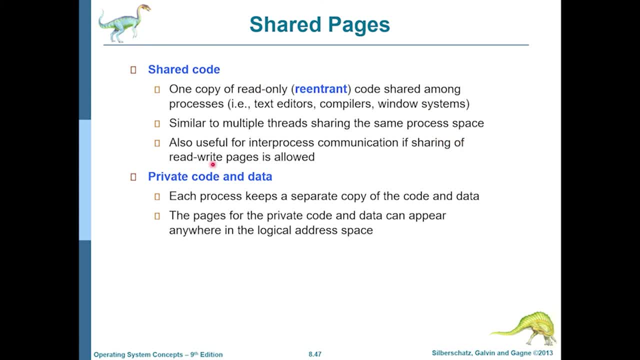 so one process can write to it, another process can then read it. they can probably use something like readers, writers, logs or other things to effectively communicate between each other. processes can also have private code and data, as they always do, and let's look at the next slide to. 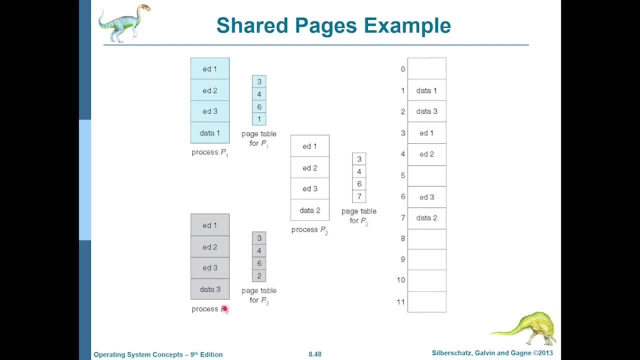 see how that happens. you can see three processes over here and the first three pages of each of these processes are shared. as you can see, the first three pages are mapped to frames three, four, six, three four, six and three four, six over here, so they are all shared between the three processes. 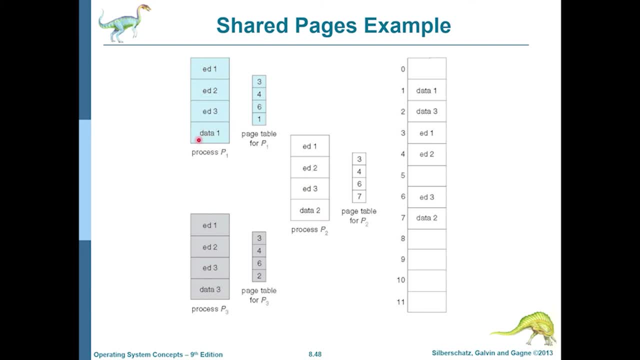 the last pages of each of these processes, that is, data one, data two and data three. they are mapped to distinct pages. so the last page here is mapped to frame number one, here it is frame number seven and here it is frame number two. so these are private pages of these processes, but ed1, ed2 and ed3 the first. 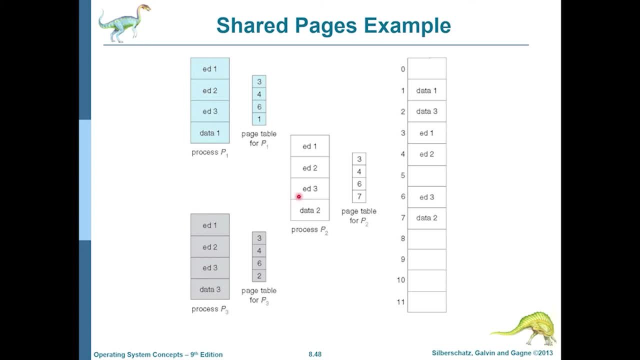 three pages of each of these processes are shared because they are all mapped to the same frames, that is, ed1, for all of them, is mapped to frame number three. ed2, for all of them, is mapped to frame number four, and ed3, for all of those processes, is mapped to frame number six. 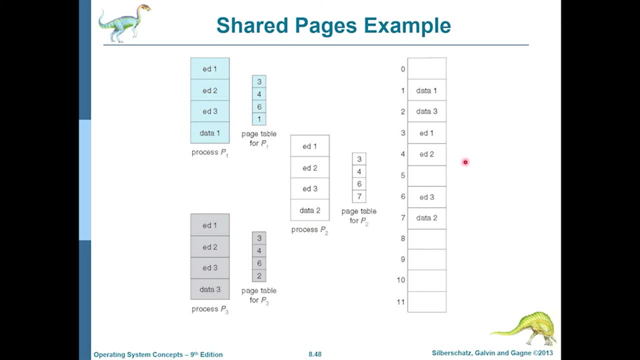 and here are the physical frames over here. as you can see, there is only one copy of ed1, one copy of ed2 and one copy of ed3, while there are three distinct copies of the private pages of these processes, that is, data one, data three and data two over here. 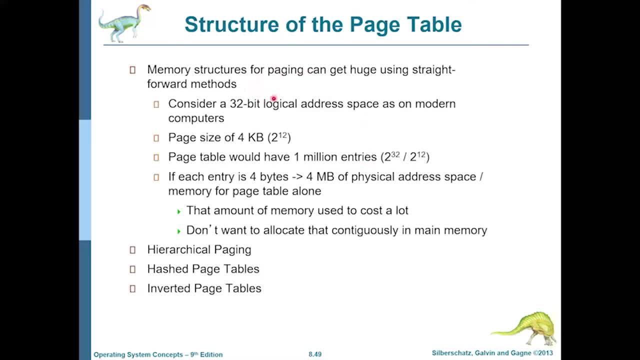 now let's consider this situation. suppose our logical address space is 32 bits in size and the page size is 4 kb, that is, the offset has 12 bits and 2 to the power. 12 is 4 kb. then how many page table entries should be there so we can divide the total size of our logical 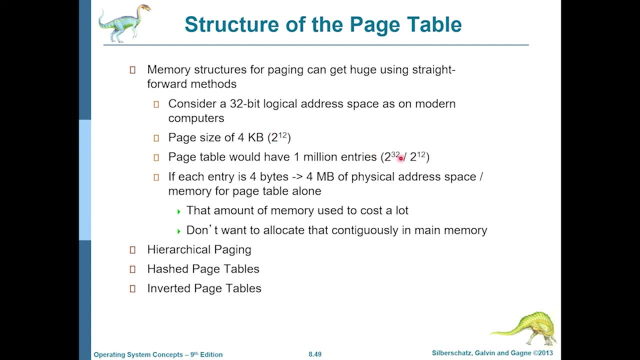 address space with the page size and we will get this number. now, if each of those entries takes 4 bytes, as in each entry would store the frame number, the different valid, read, write, execute bits and a bunch of other things, and in in real hardware and operating systems the page table entries can. 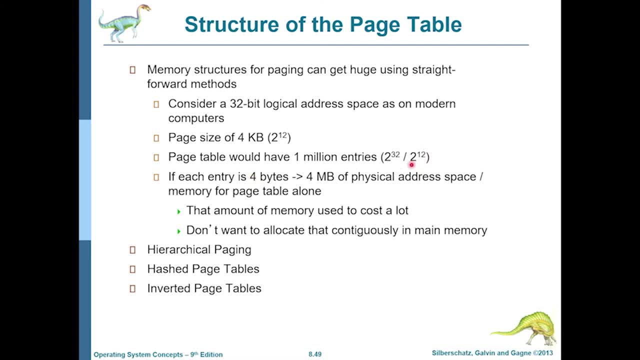 actually be 4 bytes each, then if you take this number and you multiply that by 4, you get 4 megabytes. so if we would have to have page table entries for the entire logical address space, then 4 megabytes of space would only be needed to store the page table. that is a lot of memory and it is usually. 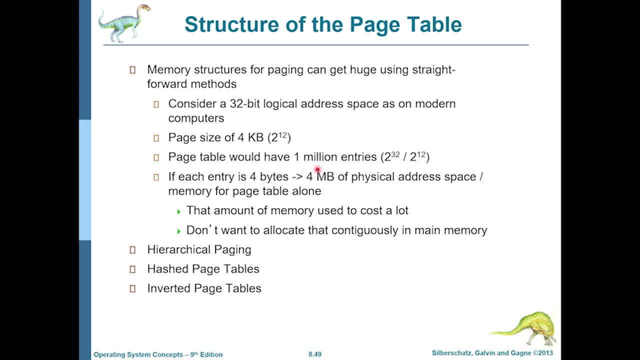 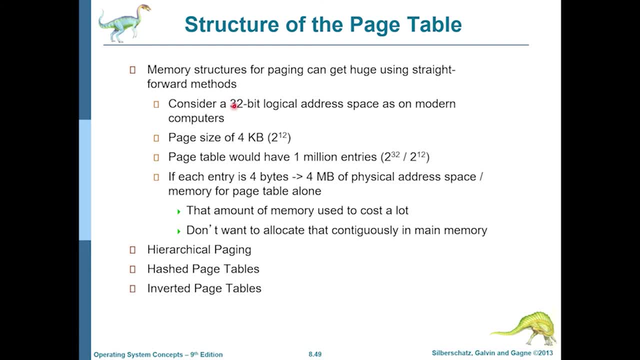 seen that process don't even need to store the page table. that is a lot of memory and it is usually seen that process don't even need to store the page table. that is a lot of memory and it is usually all the pages to them and only map some of them and have invalid bits set for the rest of the page. 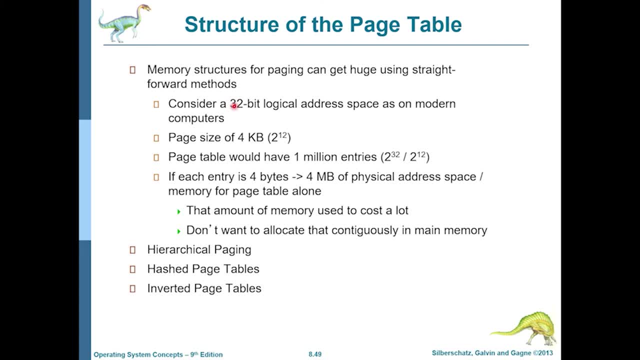 all the pages to them and only map some of them and have invalid bits set for the rest of the page. all the pages to them and only map some of them and have invalid bits set for the rest of the page. table entries. so we don't need four. 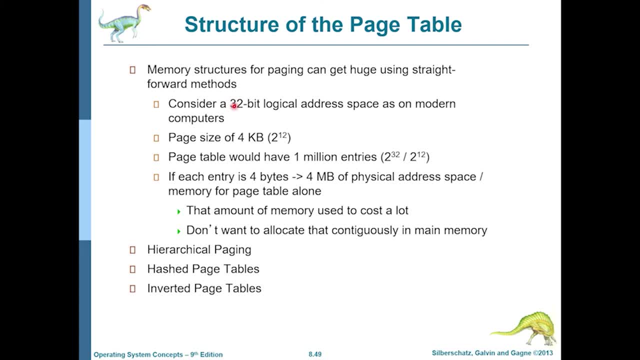 table entries. so we don't need four table entries. so we don't need four megabytes of page table entries for most megabytes of page table entries for most megabytes of page table entries for most processes. so we can start with smaller processes. so we can start with smaller. 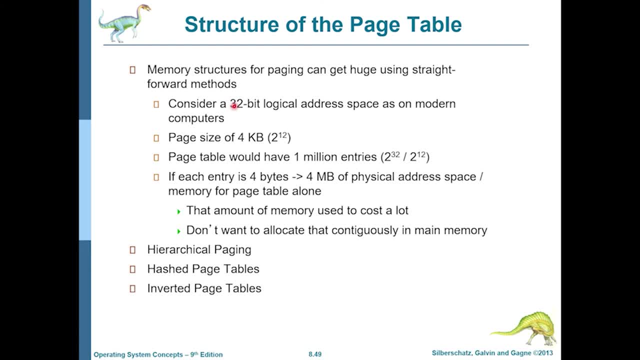 processes so we can start with smaller number of page table entries and keep on number of page table entries and keep on number of page table entries and keep on growing when we need more. so the simple growing when we need more. so the simple growing when we need more. so the simple kind of paging that we saw will always. 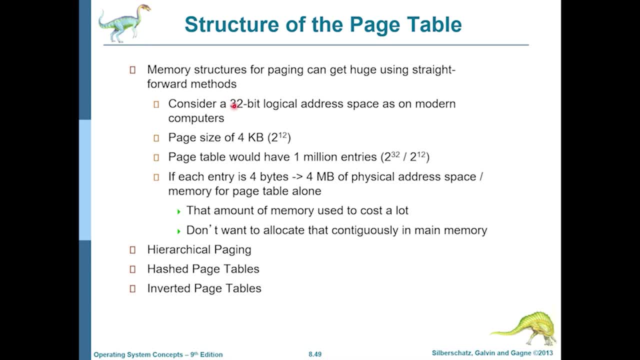 kind of paging that we saw will always kind of paging that we saw will always need all the pages mapped at any one. need all the pages mapped at any one. need all the pages mapped at any one point of time. but we can look at three point of time. but we can look at three. 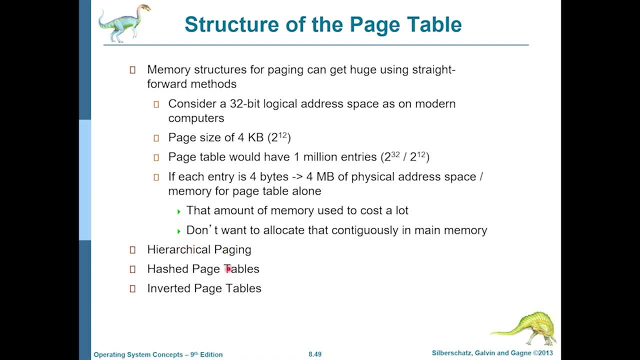 point of time. but we can look at three strategies. that is hierarchical paging strategies. that is hierarchical paging strategies. that is hierarchical paging, hashed page tables and inverted page. hashed page tables and inverted page. hashed page tables and inverted page tables in which we can get away with. tables in which we can get away with. 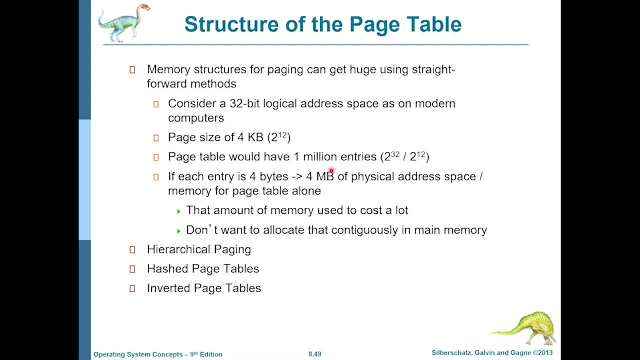 tables in which we can get away with smaller number of page table entries and smaller number of page table entries and smaller number of page table entries, and we will see how that happens in three. we will see how that happens in three. we will see how that happens in three different mechanisms. 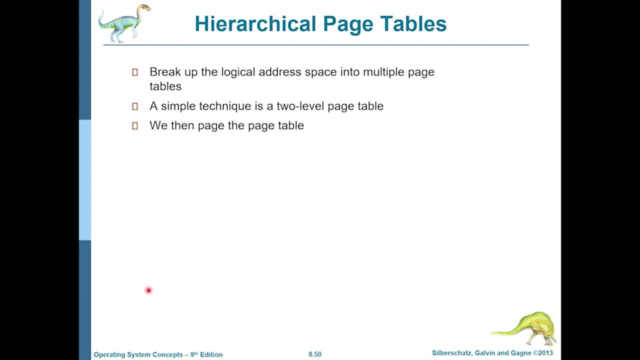 different mechanisms, different mechanisms. so the idea with hierarchical page, so the idea with hierarchical page, so the idea with hierarchical page tables, is that tables is that tables is that we just don't have one layer of page. we just don't have one layer of page. we just don't have one layer of page, tables. 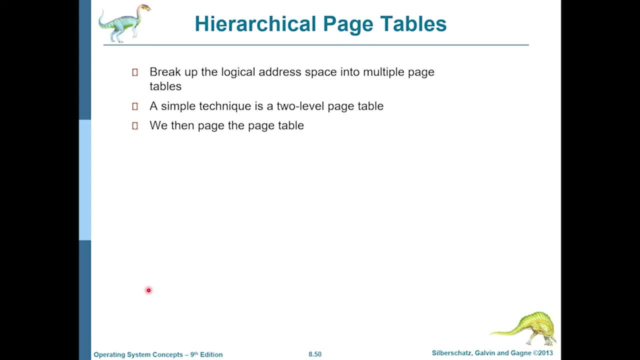 tables, tables at the beginning, so we can have multiple at the beginning. so we can have multiple at the beginning, so we can have multiple levels of page tables and we can walk levels of page tables and we can walk levels of page tables and we can walk through them so we can have the outer. 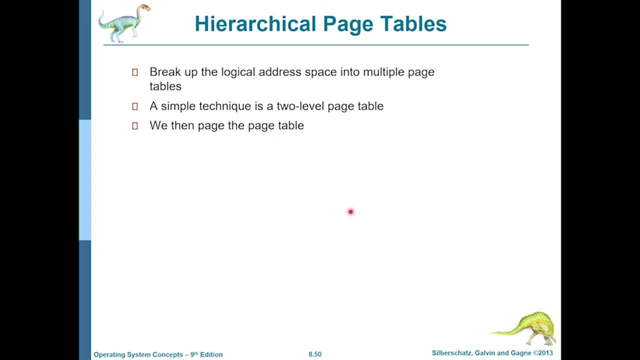 through them so we can have the outer through them, so we can have the outer page table over here. then we can have page table over here, then we can have page table over here, then we can have some inner page tables and we can have some inner page tables and we can have. 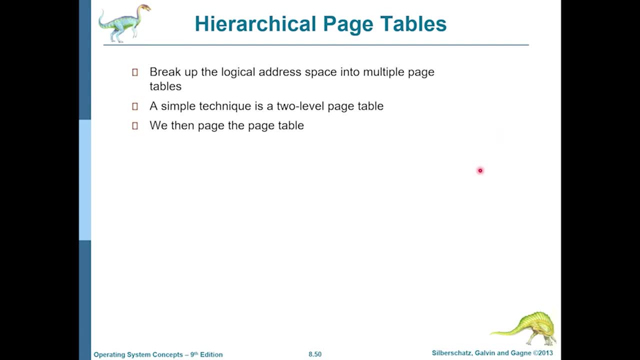 some inner page tables and we can have maybe another level of inner page tables, maybe another level of inner page tables, maybe another level of inner page tables, and then we can go to the frames and then we can go to the frames, and then we can go to the frames. so it is not necessary that the outer 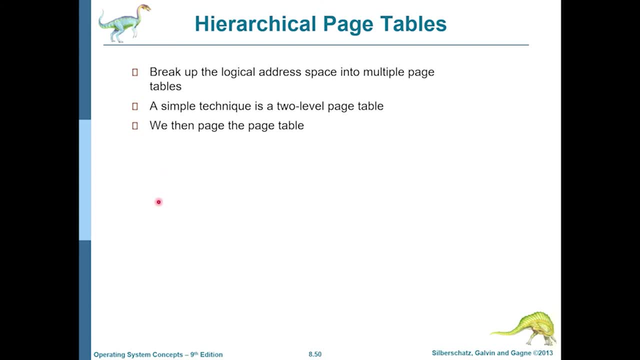 so it is not necessary that the outer. so it is not necessary that the outer page table maps the entire address space page table. maps the entire address space page table. maps the entire address space. it can choose to map only a subset of. it can choose to map only a subset of. 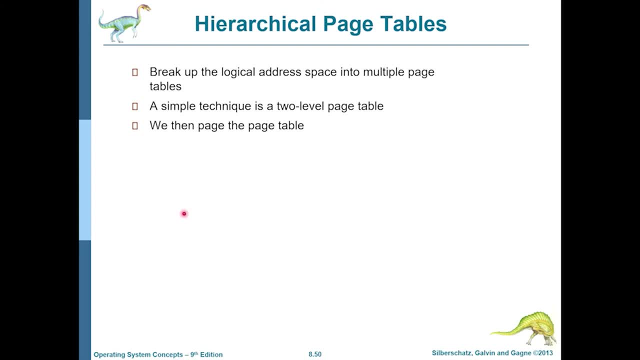 it can choose to map only a subset of the entire logical space, and then the entire logical space, and then the entire logical space, and then whatever it chooses to whatever it chooses to whatever it chooses to map, only those inner page tables will be map only those inner page tables will be. 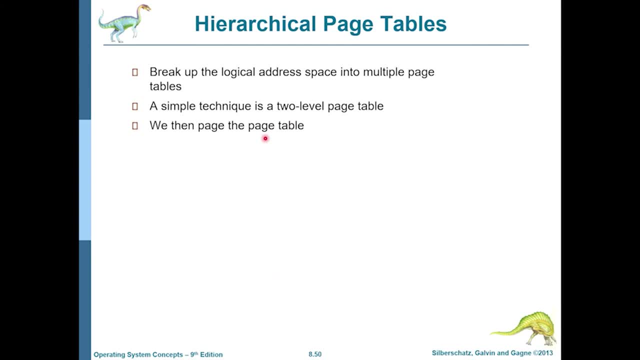 map, only those inner page tables will be present, and so we don't have to have present, and so we don't have to have present, and so we don't have to have the entirety of the page table entries, the entirety of the page table entries, the entirety of the page table entries, for the entire logical space. 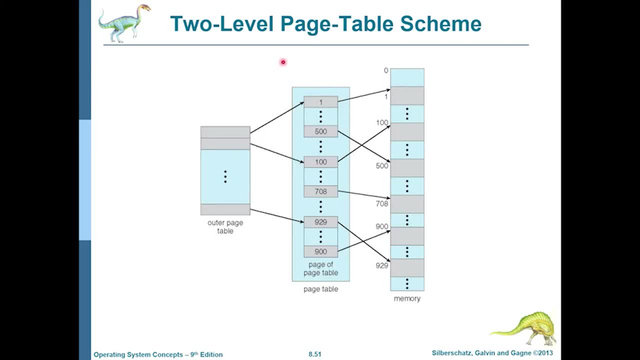 for the entire logical space, for the entire logical space. so this is one example of a two level. so this is one example of a two level. so this is one example of a two level. page table scheme. so here you can look. page table scheme. so here you can look. 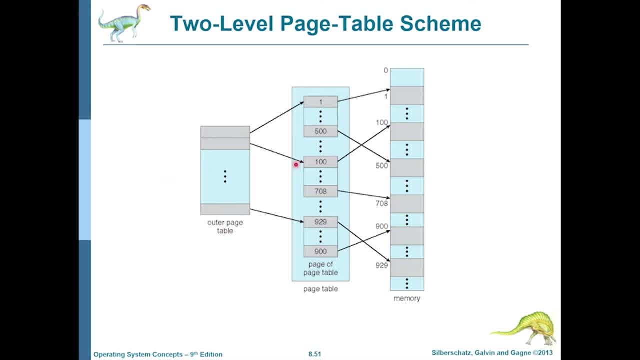 page table scheme. so here you can look at an outer page table and that points at an outer page table, and that points at an outer page table, and that points to, to, to inner page tables, and then they in turn, inner page tables, and then they in turn. 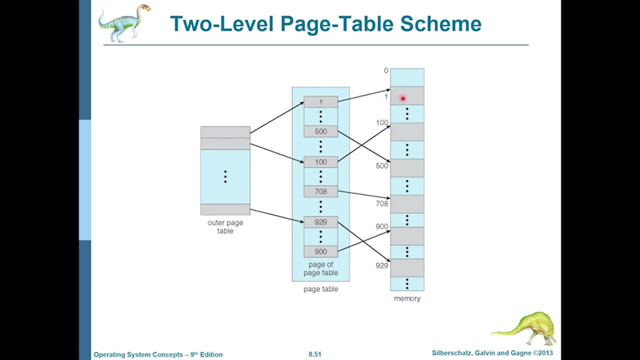 inner page tables and then they, in turn, have the real page table entries. that have the real page table entries, that have the real page table entries. that would give you the, would give you the would give you the frame numbers. now, let's explore a more frame numbers. now, let's explore a more. 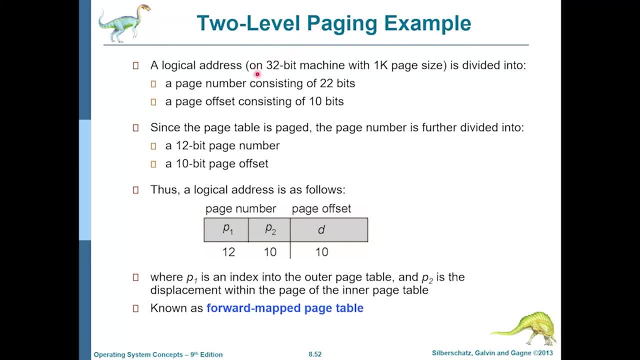 frame numbers. now let's explore a more concrete example of a two level paging. concrete example of a two level paging. concrete example of a two level paging scheme. so our machine is a 32-bit scheme. so our machine is a 32-bit scheme. so our machine is a 32-bit machine. that is the logical address space. 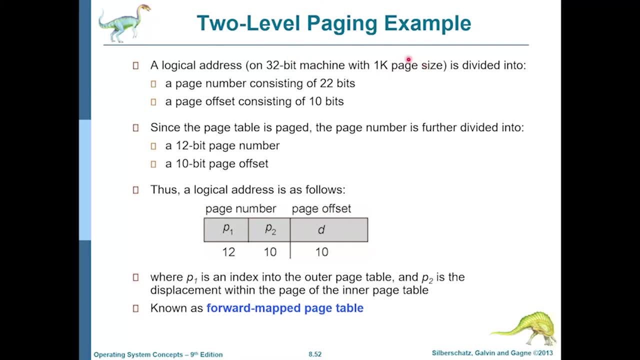 machine. that is the logical address space machine. that is the logical address space. is 32 bits wide, is 32 bits wide, is 32 bits wide, and the page size is 1k, that is 1024. and the page size is 1k, that is 1024. 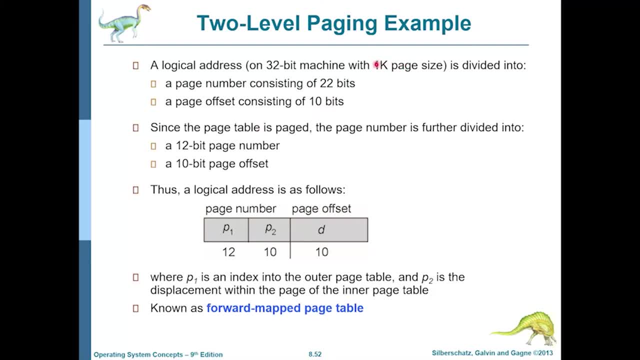 and the page size is 1k, that is 1024 bytes, bytes bytes. so if the page size is 1k, so if the page size is 1k, so if the page size is 1k, you obviously need 10 bits for the. 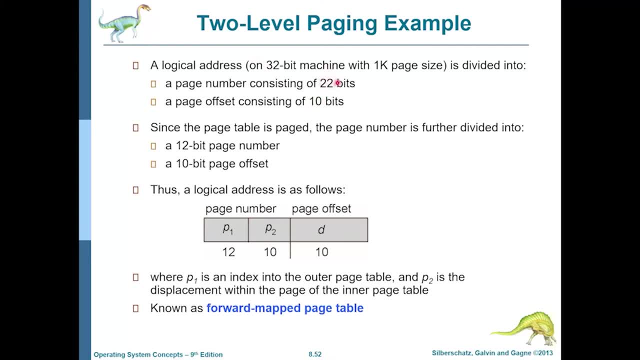 you obviously need 10 bits for the. you obviously need 10 bits for the offset- offset. so 32 minus 10 is 22 and that is what you so 32 minus 10 is 22 and that is what you so 32 minus 10 is 22, and that is what you need to signify the page number. 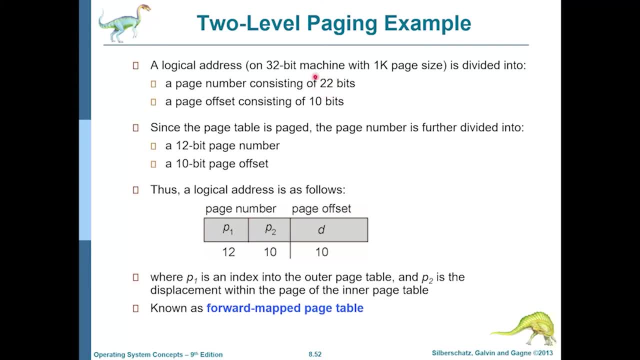 need to signify the page number, need to signify the page number. so in the initial scheme that we saw, we so in the initial scheme that we saw, we so in the initial scheme that we saw, we would have all the 22 bits, would have all the 22 bits. 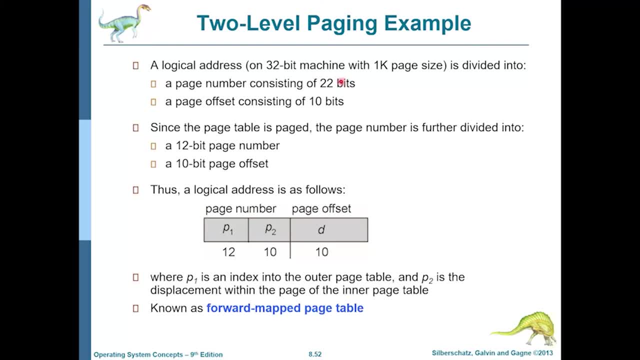 would have all the 22 bits indexed into one page table, indexed into one page table. indexed into one page table. but now with two level paging we can. but now with two level paging we can. but now with two level paging we can take those 22 bits. 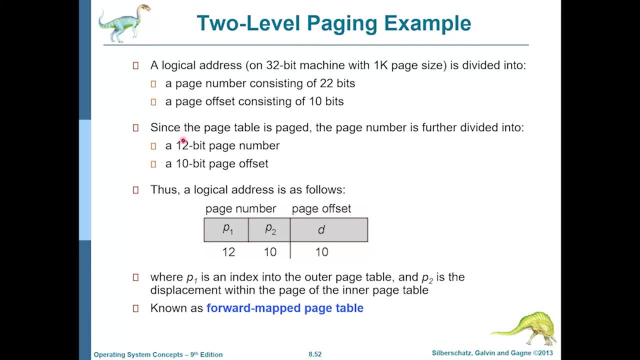 take those 22 bits. take those 22 bits and we can divide them into an outer page and we can divide them into an outer page and we can divide them into an outer page. table that would take up 12 bits. table that would take up 12 bits. 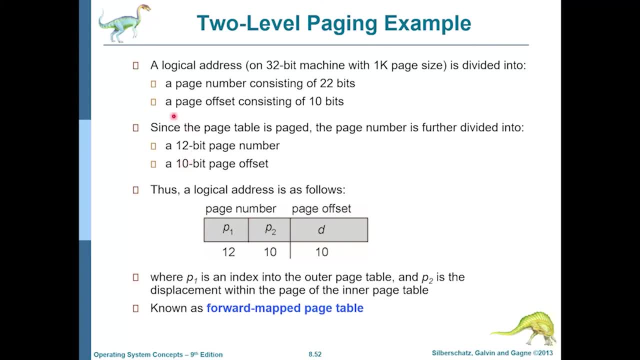 table that would take up 12 bits, and then an inner page table that would, and then an inner page table that would, and then an inner page table that would take the 10 bits. take the 10 bits, take the 10 bits. so once we go into the outer page table, 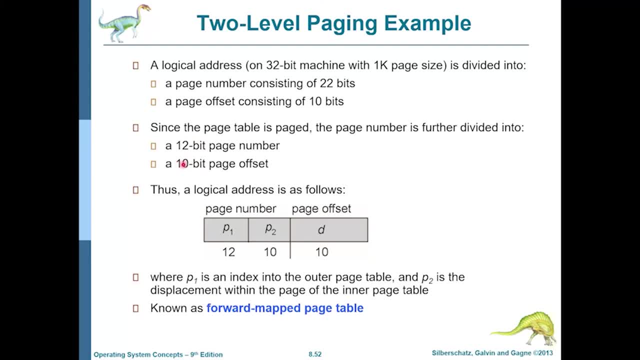 so once we go into the outer page table, so once we go into the outer page table, we figure out some location into, we figure out some location into, we figure out some location into this page table. and then, once we get this page table, and then once we get, 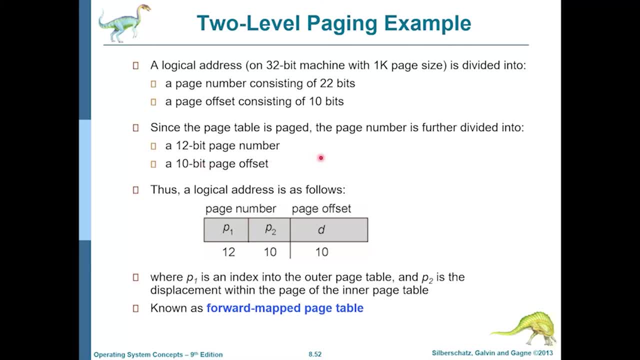 this page table and then, once we get into the inner page table, we get the into the inner page table, we get the into the inner page table, we get the real frame number, real frame number, real frame number, and then we use the page offset to get. and then we use the page offset to get. 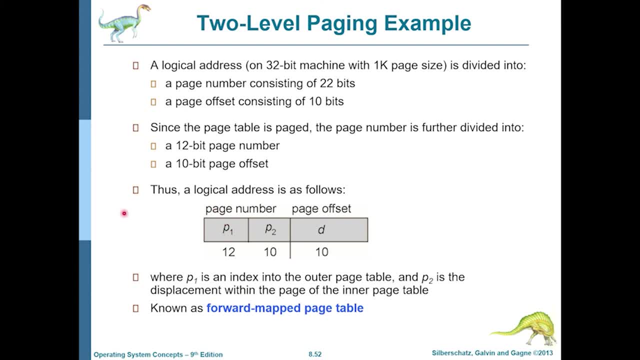 and then we use the page offset to get the inner layer. so you use p1 to index the inner layer. so you use p1 to index the inner layer. so you use p1 to index into the outer page table. you use p2 to into the outer page table. you use p2 to. 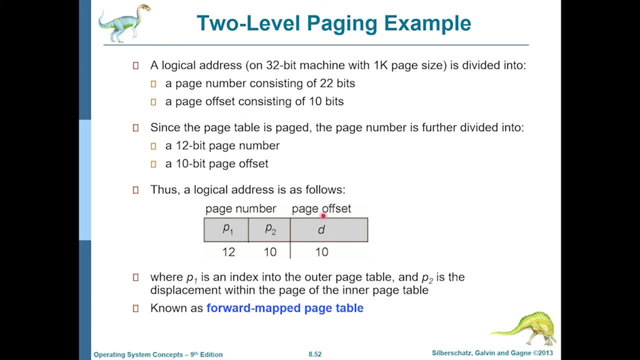 into the outer page table. you use p2 to index into the inner page table and then index into the inner page table and then index into the inner page table. and then you use the offset to index into the, you use the offset to index into the, you use the offset to index into the page. so that way, as we will see, we can. 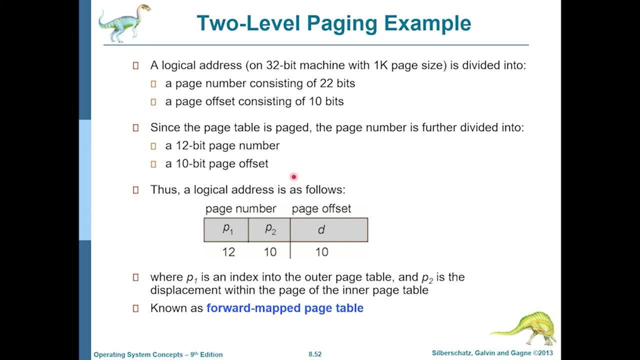 page. so that way, as we will see, we can page. so that way, as we will see, we can have far lesser page table entries. have far lesser page table entries. have far lesser page table entries. because now the number of bits for the, because now the number of bits for the 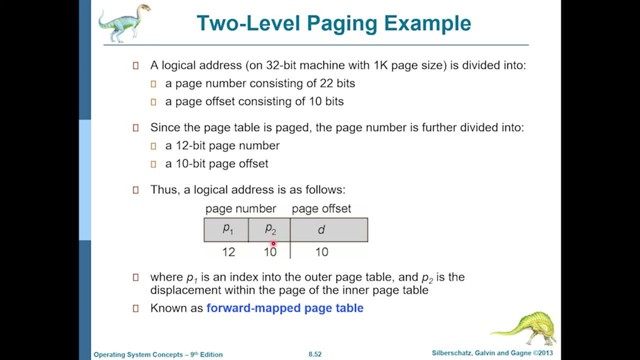 because now the number of bits for the inner page table is only 10, so we would. inner page table is only 10, so we would. inner page table is only 10, so we would not have so many inner page tables. it is not have so many inner page tables, it is. 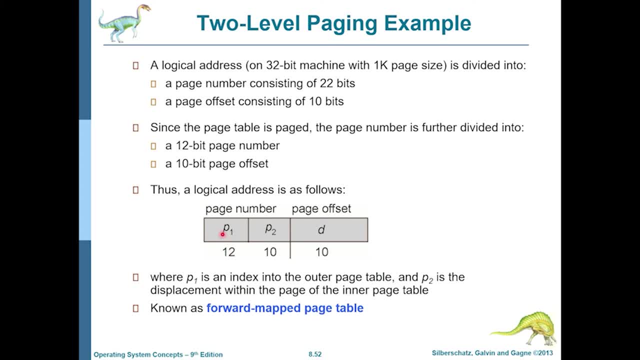 not have so many inner page tables. it is only the ones that the outer page table, only the ones that the outer page table, only the ones that the outer page table chooses to map, chooses to map, chooses to map, only those are the ones that would have, only those are the ones that would have. 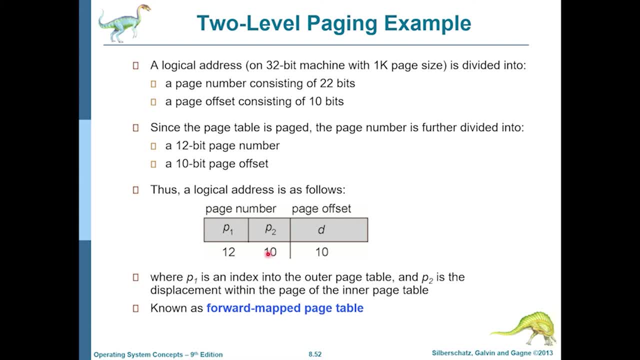 only those are the ones that would have the inner page table entries. the inner page table entries. the inner page table entries. this is usually called a forward mapped. this is usually called a forward mapped. this is usually called a forward mapped page table because we first go to the 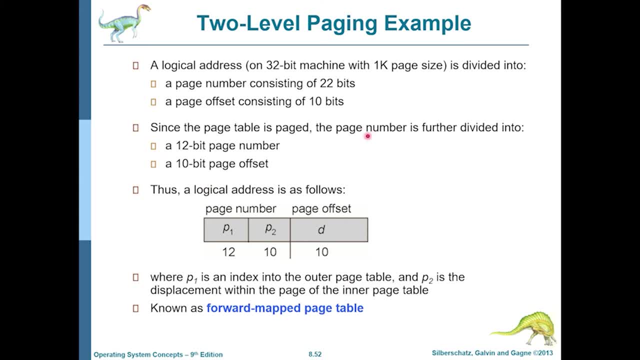 page table. because we first go to the page table, because we first go to the outer page table, then we go to the outer page table, then we go to the outer page table, then we go to the inner page table and then we go to the inner page table and then we go to the. 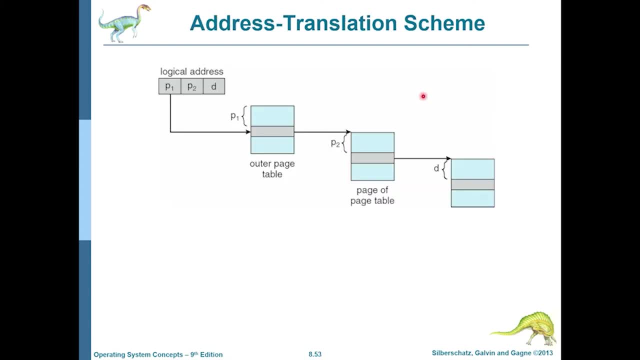 inner page table and then we go to the page and this is a more diagrammatic and this is a more diagrammatic and this is a more diagrammatic explanation of what i talked in the last explanation of what i talked in the last explanation of what i talked in the last slide. 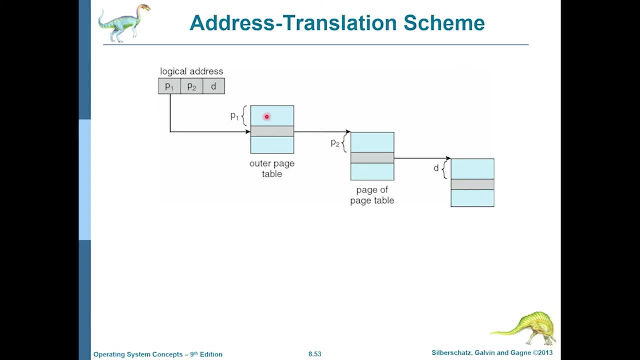 slide, slide. so we use p1 to index into an outer. so we use p1 to index into an outer. so we use p1 to index into an outer page table. so this is an outer page page table. so this is an outer page page table. so this is an outer page table. and you see the gap here from the. 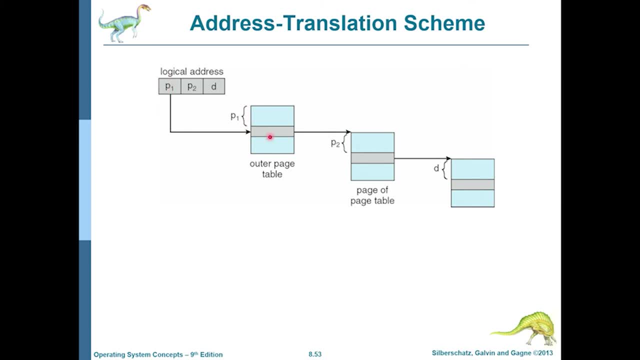 table and you see the gap here from the table and you see the gap here from the base is p1, which is basically this number. base is p1, which is basically this number. base is p1, which is basically this number over here, over here, over here, and then whatever address we get, then 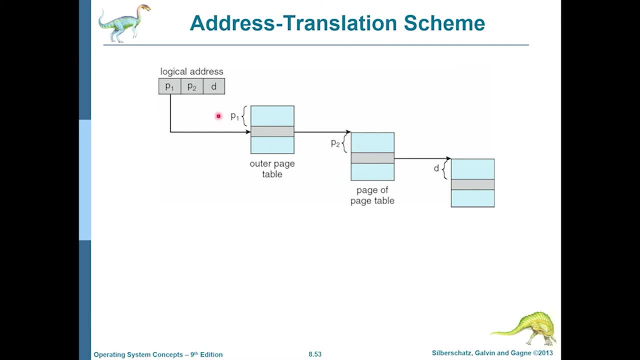 and then whatever address we get then, and then whatever address we get, then that is the base address of the inner, that is the base address of the inner, that is the base address of the inner page, table page, table, page, table, and then we use p2 to index into that. 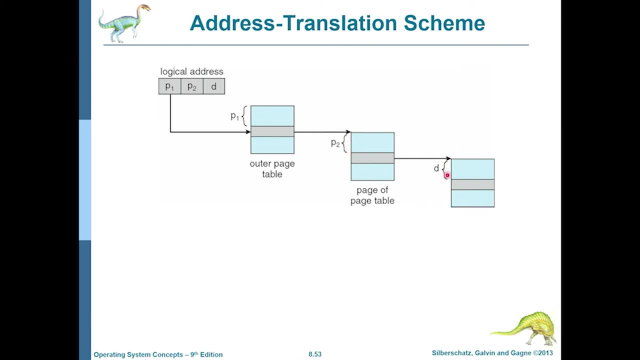 and then we use p2 to index into that, and then we use p2 to index into that. inner page table. inner page table, inner page table. and then we get the base address of the and then we get the base address of the and then we get the base address of the frame. 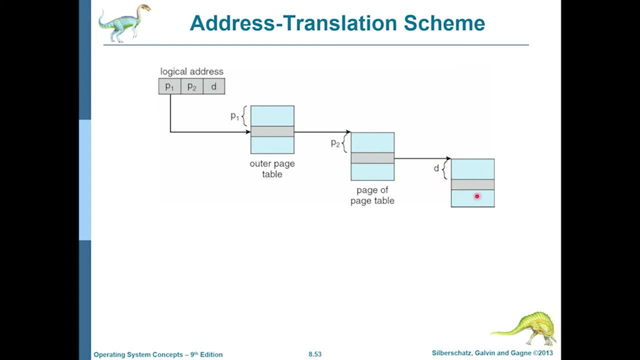 frame frame and then we use d to index into that, and then we use d to index into that, and then we use d to index into that frame and we get our, and then we use d to index into that frame and we get our physical memory location. 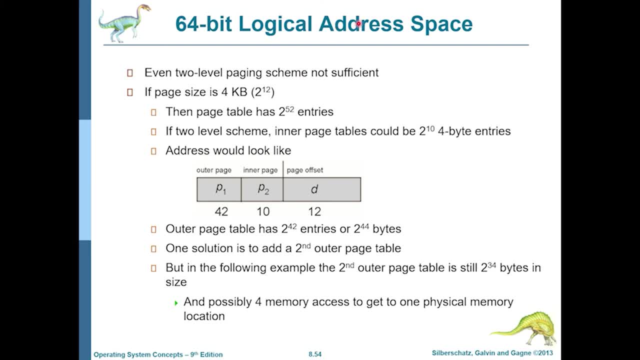 physical memory location. physical memory location. so what happens if we have a 64-bit? so what happens if we have a 64-bit? so what happens if we have a 64-bit logical address space, logical address space, logical address space? then you would see that if our page 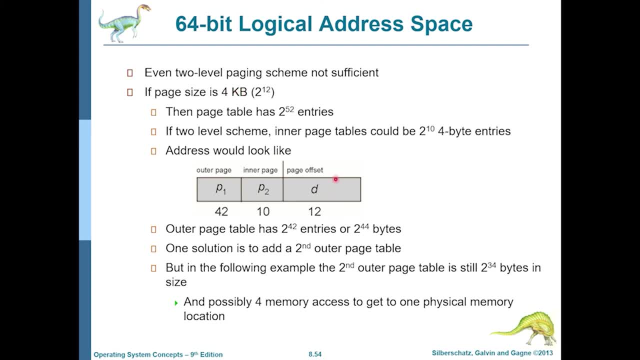 then you would see that, if our page, then you would see that if our page sizes are still, sizes are still sizes are still 4kb, so that would be 12 bits for the 4kb. so that would be 12 bits for the 4kb. so that would be 12 bits for the page offset. 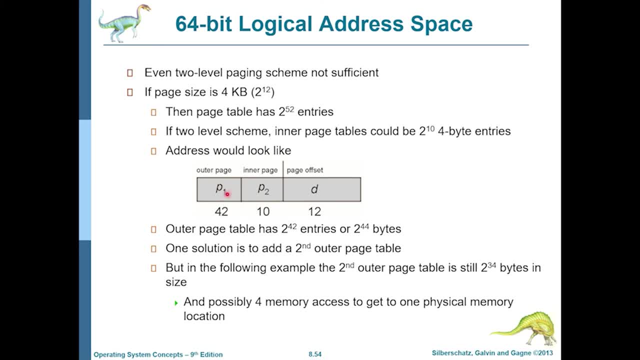 page offset. page offset. we are still left with 52 bits. we are still left with 52 bits. we are still left with 52 bits for the page numbers. and then if we do for the page numbers, and then if we do for the page numbers, and then if we do a split like this of the outer page table: 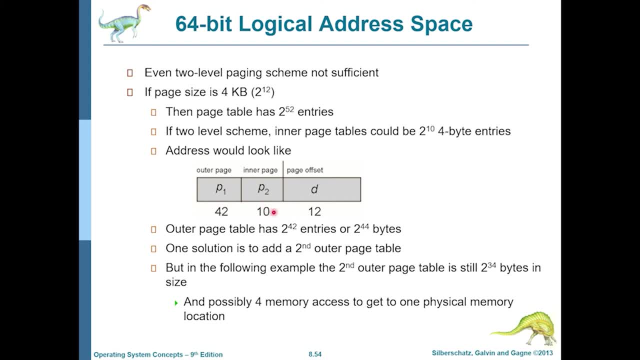 a split like this of the outer page table. a split like this of the outer page table getting 42 bits and the inner page getting 42 bits, and the inner page getting 42 bits and the inner page table getting 10 bits, then 42 bits is again. 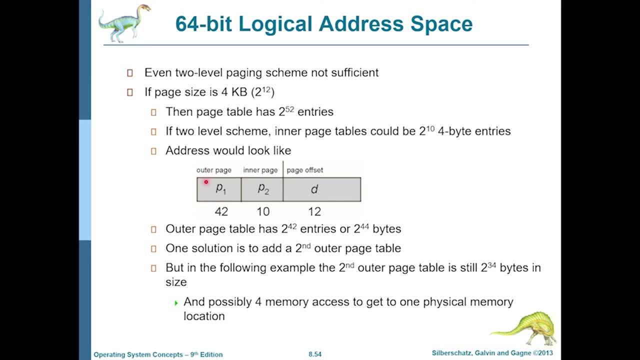 table getting 10 bits then 42 bits is again table. getting 10 bits then 42 bits is again too high of a number, for too high of a number, for too high of a number for outer pages. that would be 2 to the outer pages. that would be 2 to the. 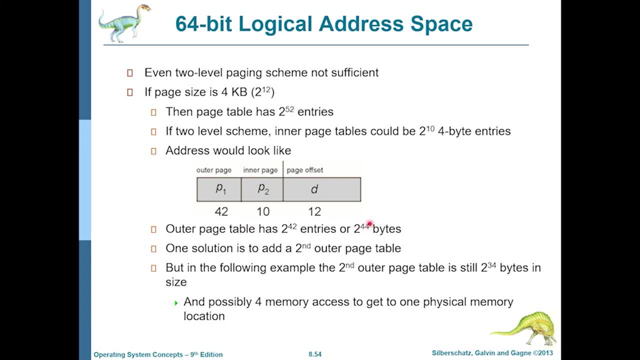 outer pages. that would be 2 to the power 44 bytes. power 44 bytes. power 44 bytes. that is a lot of bytes just for the outer. that is a lot of bytes just for the outer. that is a lot of bytes just for the outer page tables. so 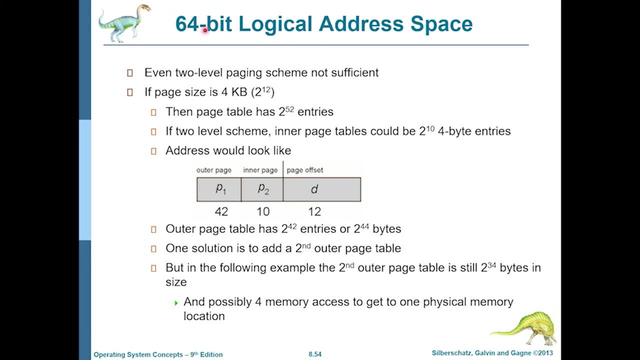 page tables, so page tables. so two levels of paging is not sufficient. two levels of paging is not sufficient. two levels of paging is not sufficient for 64-bit logical address spaces. we will for 64-bit logical address spaces. we will for 64-bit logical address spaces. we will need more levels for 64-bit logical. 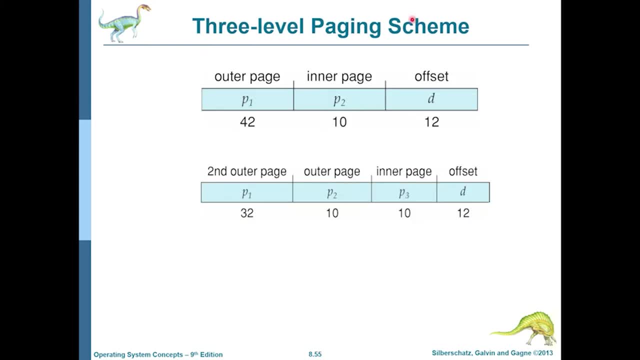 need more levels for 64-bit logical need more levels for 64-bit logical addresses, addresses, addresses. so we go for a three level paging scheme. so we go for a three level paging scheme. so we go for a three level paging scheme. so if we had to do a two level paging, 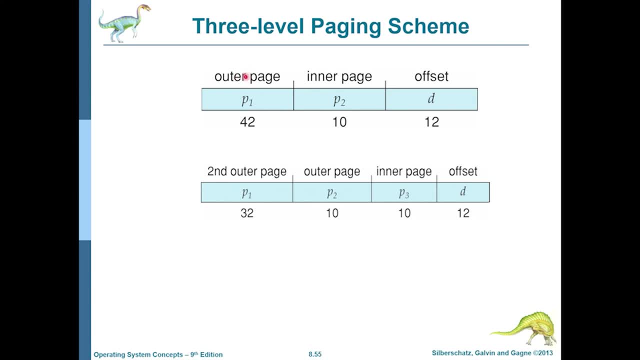 so if we had to do a two level paging? so if we had to do a two level paging scheme, we'd have to have 42 bits for the scheme. we'd have to have 42 bits for the scheme. we'd have to have 42 bits for the outer page. but what we usually do is: 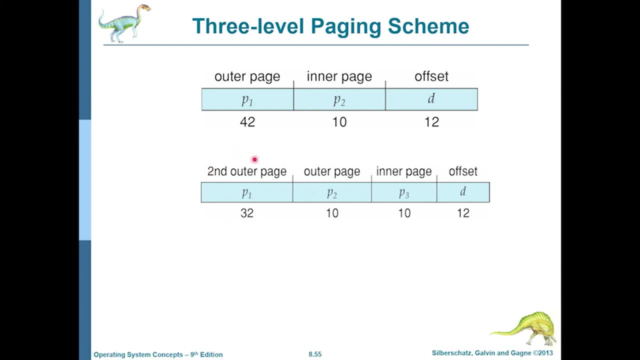 outer page, but what we usually do is outer page, but what we usually do is that we split it into one more level. so that we split it into one more level, so that we split it into one more level, so we have a second outer page of 32 bits. 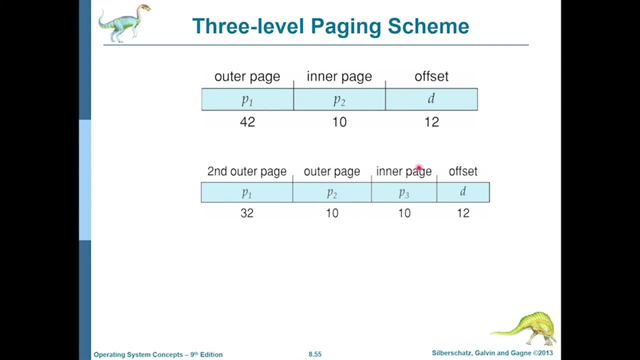 we have a second outer page of 32 bits. we have a second outer page of 32 bits, we have an outer page of 10 bits and we we have an outer page of 10 bits and we we have an outer page of 10 bits and we have an inner page of. 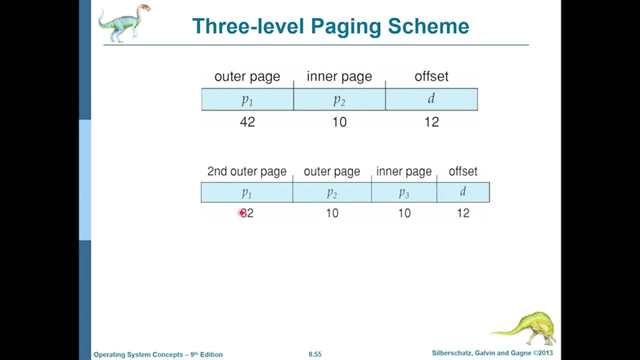 have an inner page of, have an inner page of 10 bits, and then the offset is of 12 bits, 10 bits, and then the offset is of 12 bits, 10 bits, and then the offset is of 12 bits. so if i take the 32 bits of the 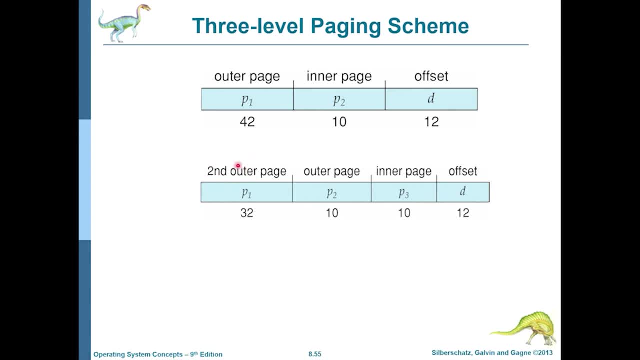 so if i take the 32 bits of the, so if i take the 32 bits of the logical address here, logical address here, logical address here, and i index into the second outer page i and i index into the second outer page i and i index into the second outer page, i will find the base address of the outer. 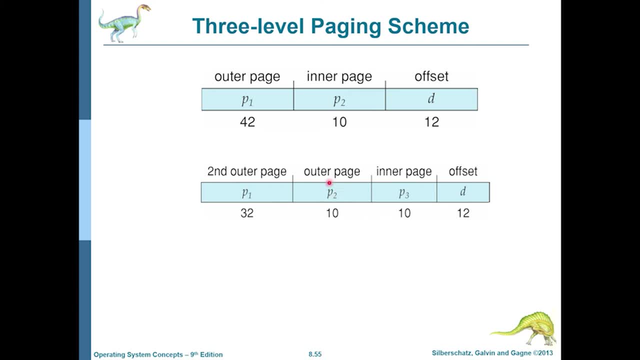 will find the base address of the outer will find the base address of the outer page, page page. once i find the base address of the outer, once i find the base address of the outer, once i find the base address of the outer page, i will use these 10 bits to index. 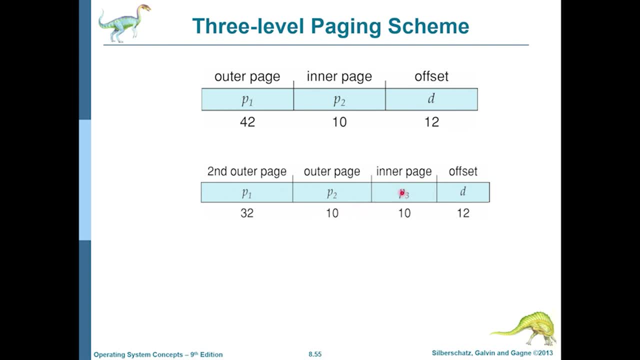 page. i will use these 10 bits to index page. i will use these 10 bits to index into that page to find out the base into that page to find out the base into that page to find out the base. address of the inner page. address of the inner page. 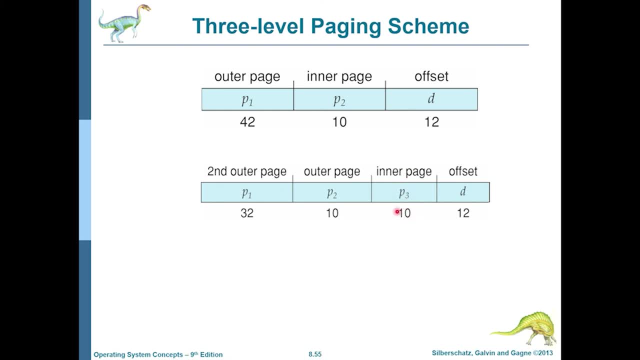 address of the inner page. once i find the base address of the, once i find the base address of the, once i find the base address of the inner page, i will use these 10 bits to inner page. i will use these 10 bits to inner page. i will use these 10 bits to index into that to find the. 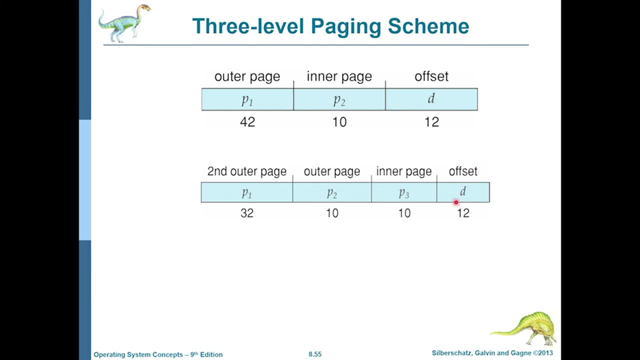 index into that to find the index into that to find the base address of the frame. then once i base address of the frame, then once i base address of the frame, then once i know the base address of the physical, know the base address of the physical, know the base address of the physical frame, then i will use the 12 bits over. 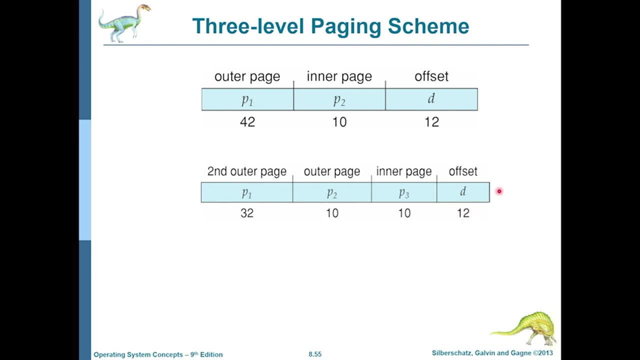 frame. then i will use the 12 bits over frame, then i will use the 12 bits over here to index into that frame and find here to index into that frame and find here to index into that frame and find my physical memory location. let's quickly look at another variation. 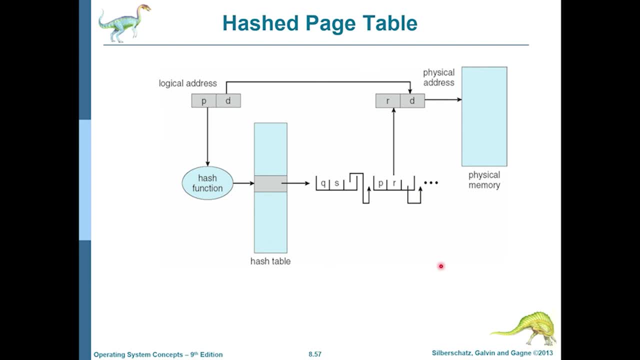 let's quickly look at another variation. let's quickly look at another variation of the mechanisms that can be used to, of the mechanisms that can be used to, of the mechanisms that can be used to not have so many page table entries, not have so many page table entries. 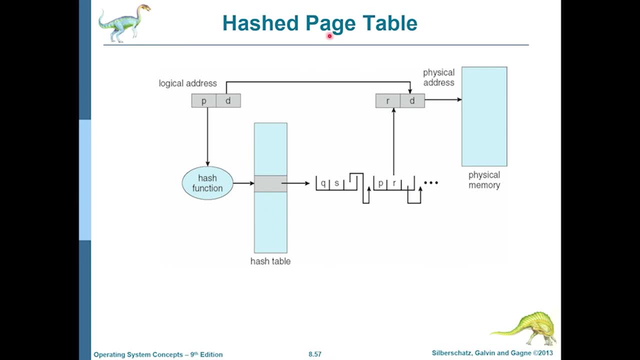 not have so many page table entries. so apart from multi-level paging schemes, so apart from multi-level paging schemes, so apart from multi-level paging schemes, we can also use hashed page tables and we can also use hashed page tables and we can also use hashed page tables. and in the diagram it is pretty clear what. 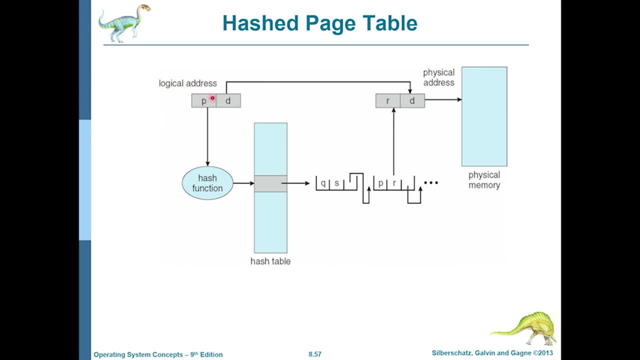 in the diagram it is pretty clear what. in the diagram it is pretty clear what it is doing. it is doing. it is doing so. our logical address space is again. so our logical address space is again. so our logical address space is again divided into a page number and 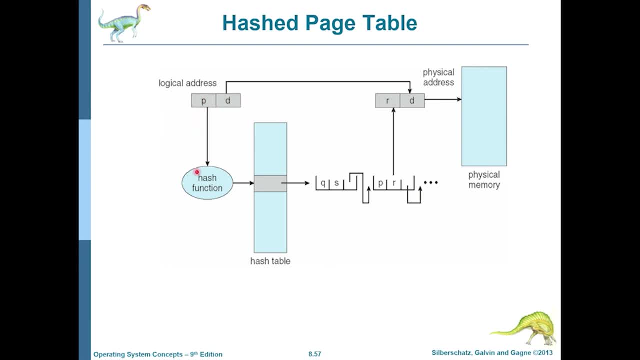 divided into a page number and divided into a page number and an offset. we can take the page number and an offset. we can take the page number and an offset. we can take the page number and, instead of directly indexing into a, instead of directly indexing into a. 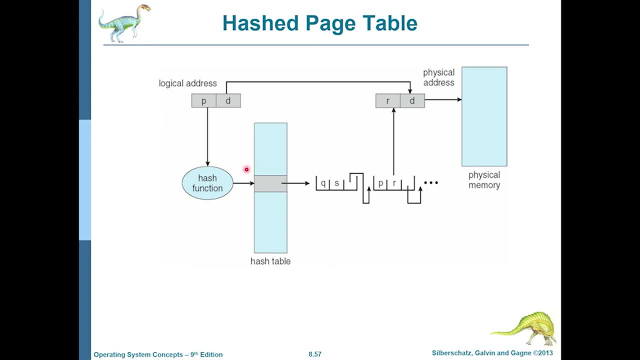 instead of directly indexing into a page table. and if we page table and if we page table, and if we do that we would really need lots of page. do that, we would really need lots of page. do that, we would really need lots of page table entries. and that is why we are. 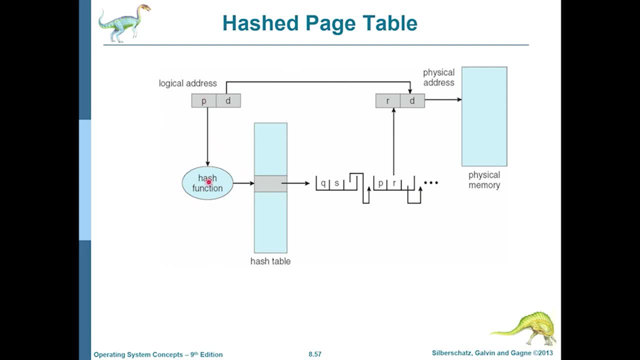 table entries, and that is why we are table entries and that is why we are not doing it. not doing it. not doing it, we would actually take the page number, we would actually take the page number, we would actually take the page number and use a hash function. 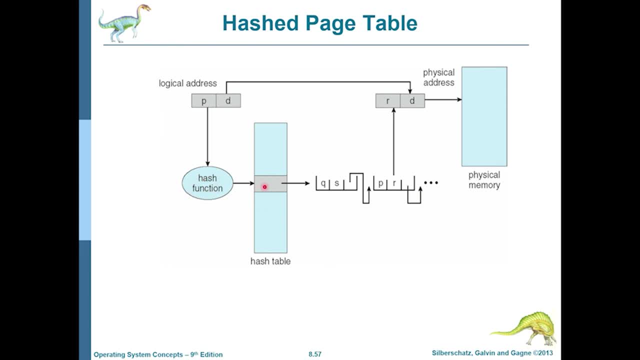 and use a hash function and use a hash function and the hash function will give us a. and the hash function will give us a. and the hash function will give us a location in a hash table. location in a hash table. location in a hash table that has page table entries inside them. 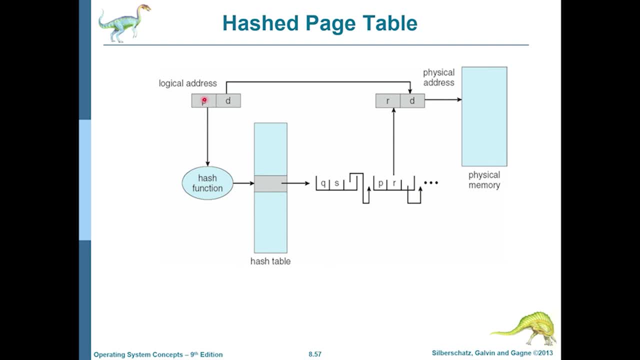 that has page table entries inside them. that has page table entries inside them. so so, so, look at this, so we take p, and we look at this, so we take p and we look at this, so we take p and we put it into a hash function. we get some. 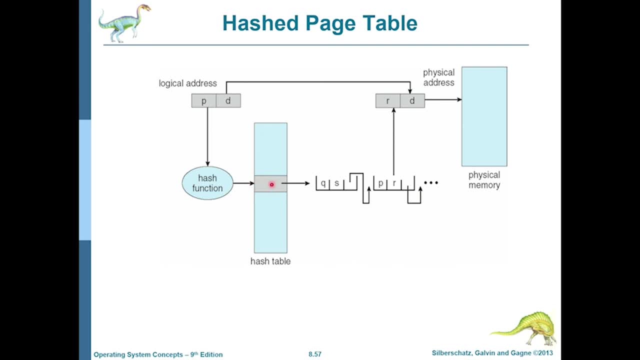 put it into a hash function, we get some. put it into a hash function, we get some value and then that helps us value, and then that helps us value and then that helps us do a lookup inside a hash table, that. do a lookup inside a hash table that. 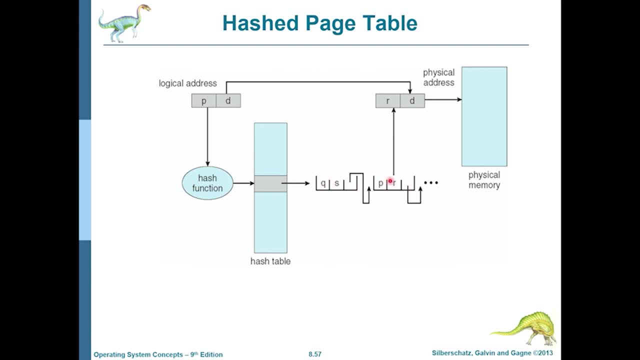 do a lookup inside a hash table that has a few page table entries chained. has a few page table entries chained. has a few page table entries chained like this. now you might ask why is this like this? now you might ask, why is this like this? now you might ask why is this chaining there? because whenever you use 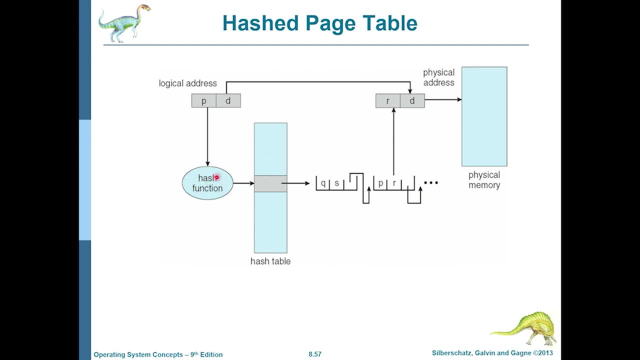 chaining there. because whenever you use chaining there, because whenever you use a hash function, there is a possibility, a hash function, there is a possibility, a hash function, there is a possibility of collisions, of collisions, of collisions. so more than one entries can map to the. so more than one entries can map to the. 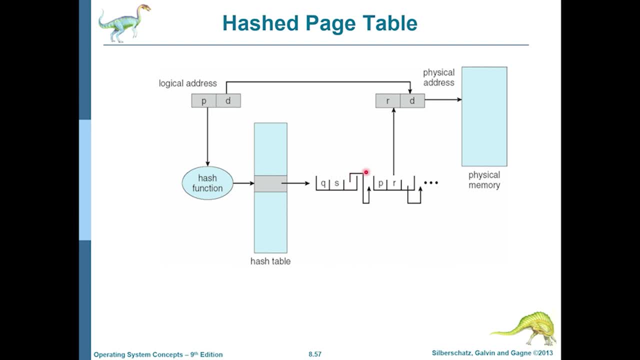 so more than one entries can map to the same hash function value. same hash function value, same hash function value. so there is a possibility that multiple. so there is a possibility that multiple. so there is a possibility that multiple page table entries could exist here. page table entries could exist here. 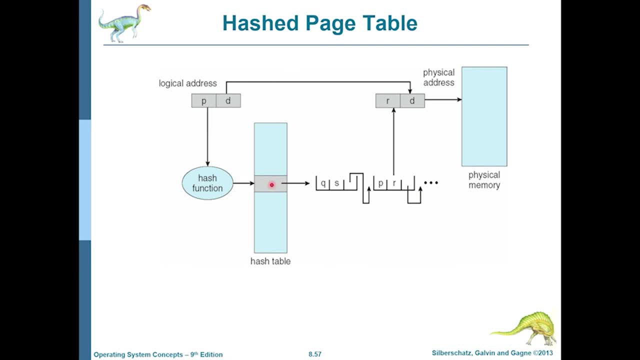 page table entries could exist here. so what we can do is after we look into. so what we can do is after we look into. so what we can do is after we look into this hash table and we find these values, this hash table- and we find these values. 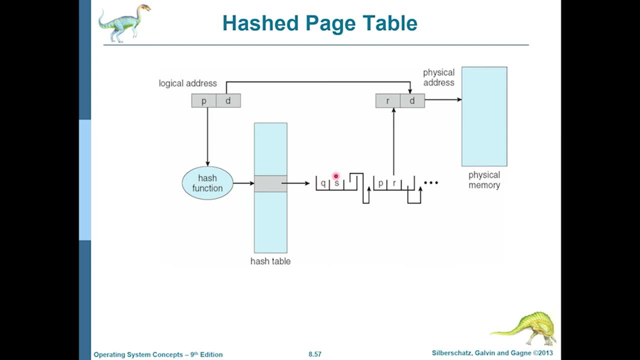 this hash table and we find these values over here, over here, over here. we go one by one to see which one of them. we go one by one to see which one of them. we go one by one to see which one of them has p, has p. 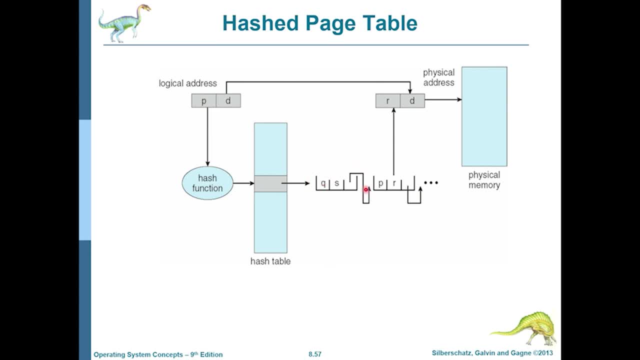 has p, because that is our page number. so this is because that is our page number. so this is because that is our page number. so this is q, so we go to the next one in the link. q. so we go to the next one in the link. 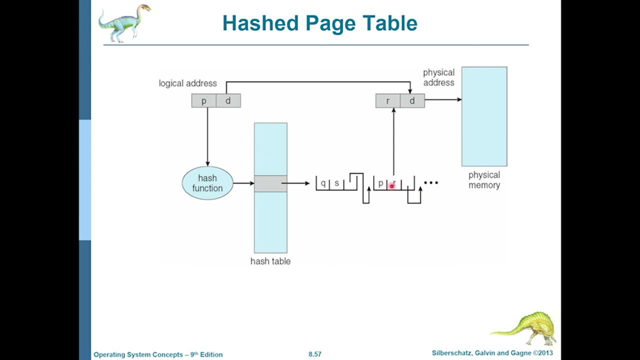 q. so we go to the next one in the link list and we get p, and we know that the list, and we get p. and we know that the list and we get p, and we know that the frame number here is r, so we patch p by. 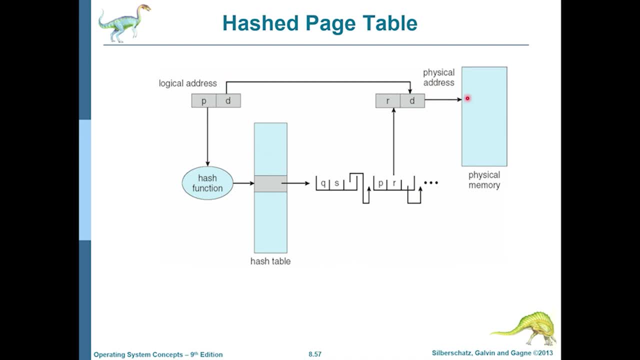 frame number: here is r, so we patch p by frame number: here is r, so we patch p by r and the offset remains the same. and we r and the offset remains the same and we r and the offset remains the same. and we go to the physical address. 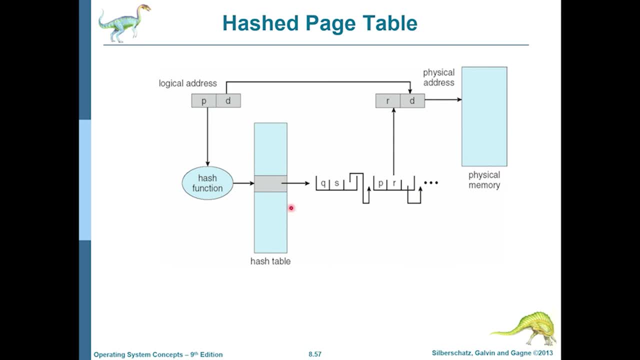 go to the physical address. go to the physical address. so in this hash table, we don't have to. so in this hash table, we don't have to. so in this hash table, we don't have to store information about all the page. store information about all the page. 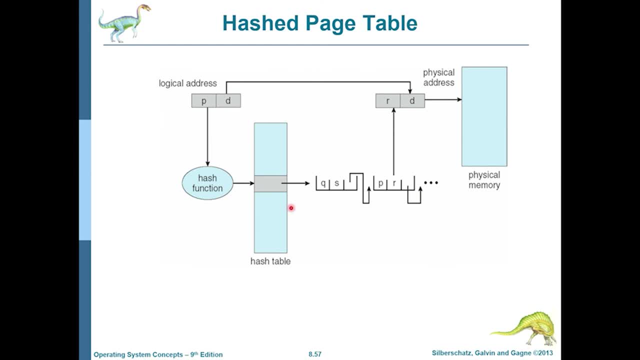 store information about all the page table entries. that is, we don't need table entries. that is, we don't need table entries. that is, we don't need information about all the possible page information about all the possible page information about all the possible page table entries that occupy 4mb of space. 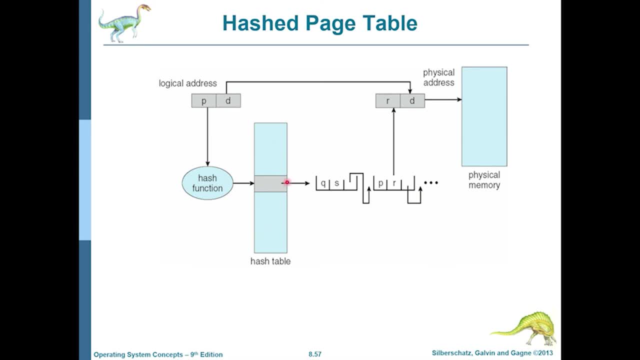 table entries that occupy 4mb of space. table entries that occupy 4mb of space. as we saw before, we can get away with as we saw before. we can get away with as we saw before. we can get away with only a small number of page double. 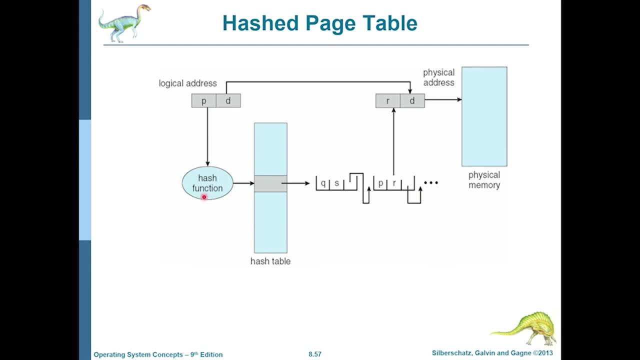 only a small number of page double, only a small number of page double. entries over here and, as you know, has entries over here and, as you know, has entries over here and, as you know, has. functions are really quick, but they can. functions are really quick, but they can. 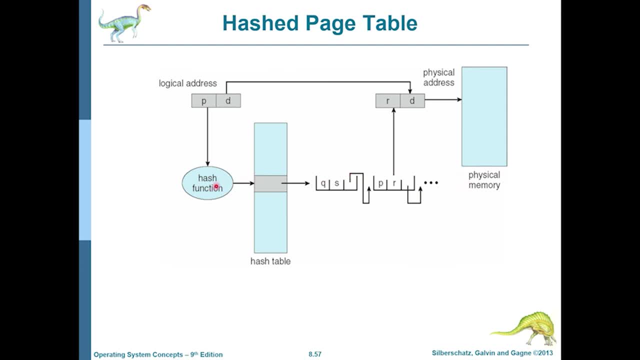 functions are really quick, but they can not be off one if there are a lot of not be off one if there are a lot of not be off one if there are a lot of collisions, by the way, so we have to. collisions by the way, so we have to. 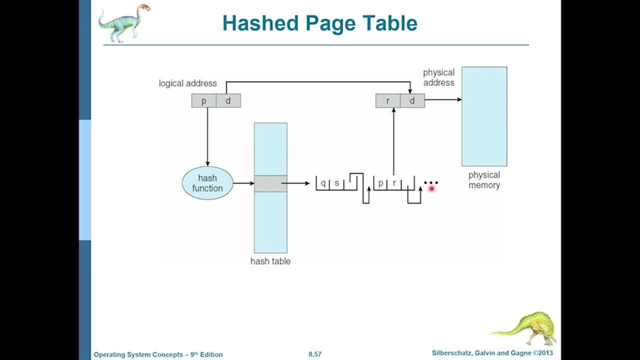 collisions, by the way. so we have to choose our hash function in a way that choose our hash function in a way that choose our hash function in a way that avoids lots of collisions, because for avoids lots of collisions, because for avoids lots of collisions, because, for example, here we got lucky because only 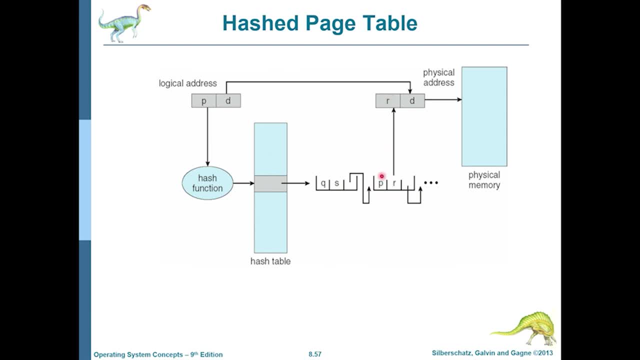 example: here we got lucky, because only example: here we got lucky, because only the second entry was the correct one. but the second entry was the correct one. but the second entry was the correct one. but what if this chain was really really? what if this chain was really really? 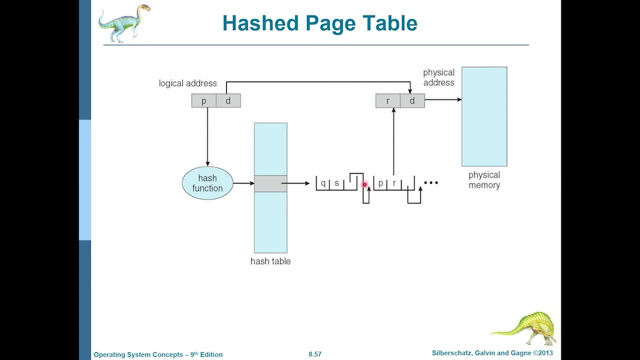 what if this chain was really really long, then this operation will not be off. long then this operation will not be off. long then this operation will not be off one. and we need to traverse this link one, and we need to traverse this link one, and we need to traverse this link list until we find the correct page. 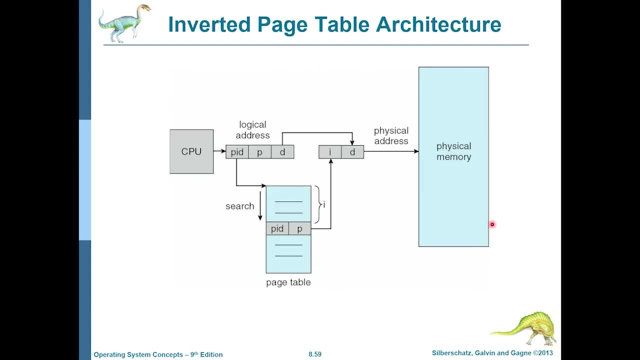 list until we find the correct page list, until we find the correct page number that we are looking for. let's look at the third mechanism using. let's look at the third mechanism using. let's look at the third mechanism using which we can avoid having too many page. 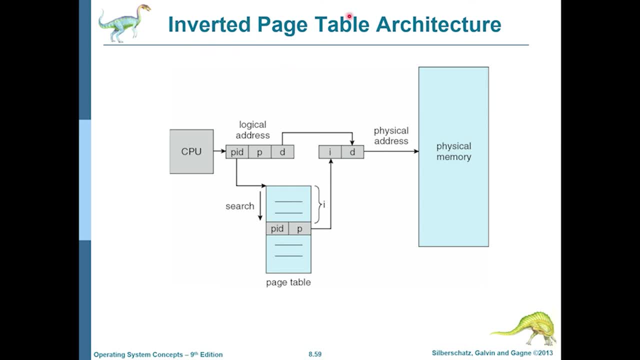 which we can avoid having too many page, which we can avoid having too many page table entries, and that is called table entries, and that is called table entries, and that is called inverted page table architecture. so inverted page table architecture, so inverted page table architecture. so this diagram again makes it very, very. 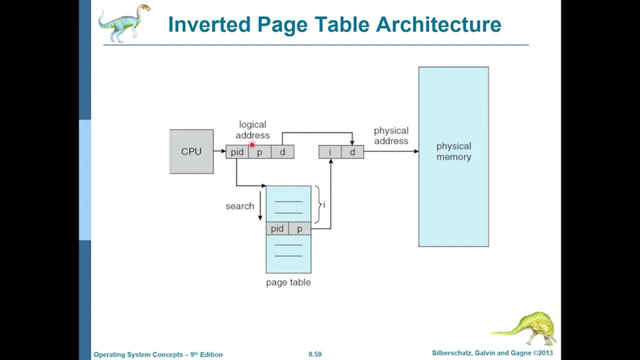 this diagram again makes it very, very. this diagram again makes it very, very clear, clear, clear. when you generate logical addresses, we, when you generate logical addresses, we, when you generate logical addresses, we also take into account the process id, also take into account the process id, also take into account the process id and, as always, we have the page number. 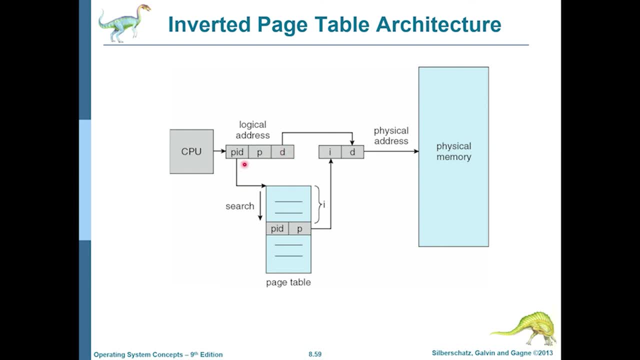 and as always, we have the page number and as always we have the page number and the offset, the page offset right and the offset, the page offset right and the offset, the page offset right. here, here, here. so we take the combination of pid and so we take the combination of pid and 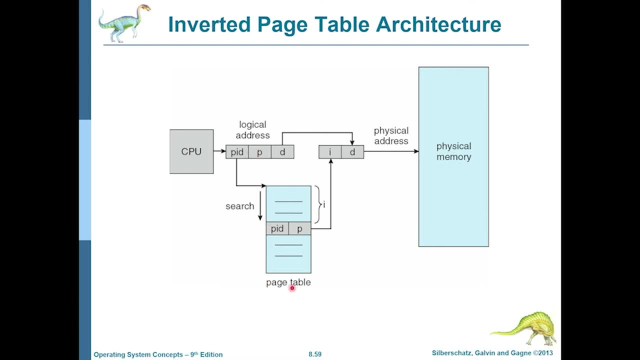 so we take the combination of pid and the page number and then we do a linear the page number and then we do a linear the page number and then we do a linear search inside a page table. search inside a page table. search inside a page table. now, it is not guaranteed that this page. 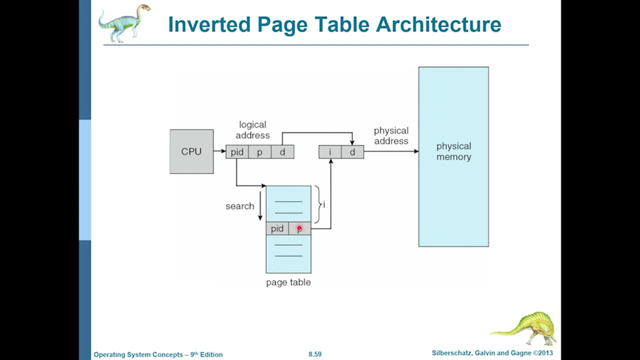 now it is not guaranteed that this page, now it is not guaranteed that this page table is sorted according to table- is sorted according to table. is sorted according to the page number. it is not. it is actually the page number. it is not. it is actually the page number. it is not. it is actually sorted according to the frame number. 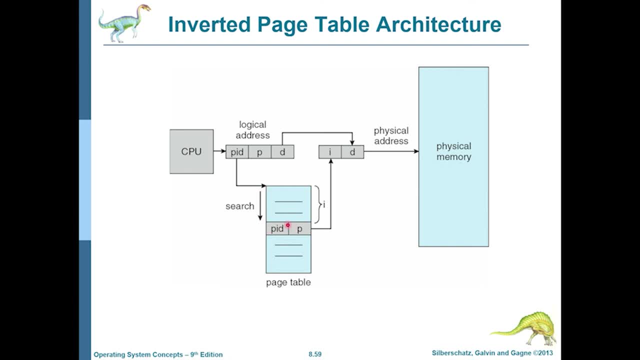 sorted according to the frame number. sorted according to the frame number. so once we do a search and at one point. so once we do a search and at one point. so once we do a search and at one point, we will find the pidp combination over. we will find the pidp combination over. 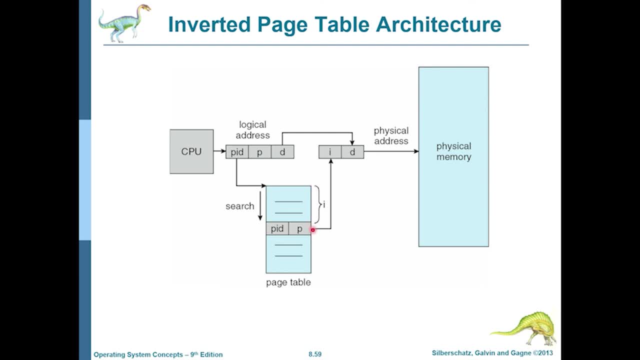 we will find the pidp combination over here and then we will see how far down here and then we will see how far down here and then we will see how far down the page table have we gone? and this the page table: have we gone? and this: 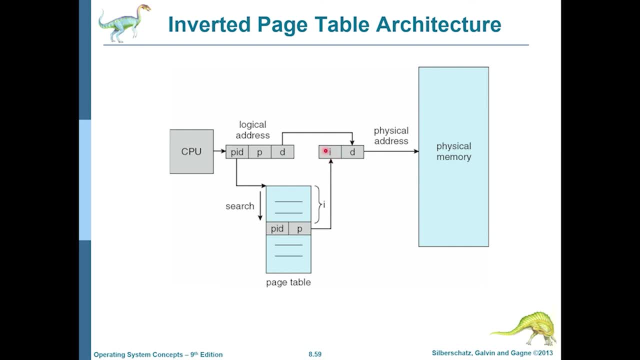 the page table have we gone, and this distance from the base is actually the distance from the base is actually the distance from the base is actually the frame number. and then, once we find the frame number, and then once we find the frame number, and then once we find the frame number, we can use the offset over. 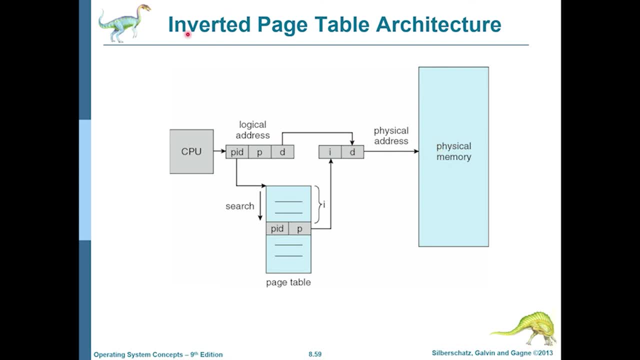 frame number. we can use the offset over frame number. we can use the offset over here and we can go to physical memory here and we can go to physical memory here and we can go to physical memory. the reason why this is called inverted. the reason why this is called inverted. 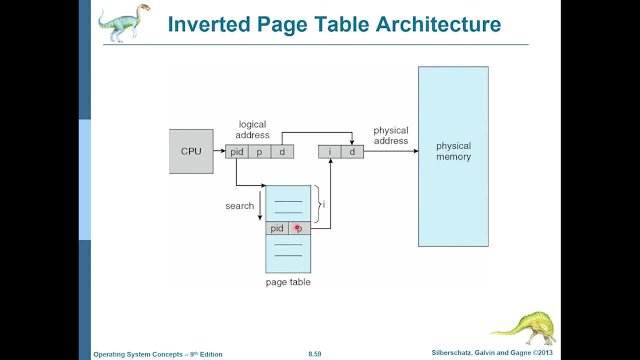 the reason why this is called inverted is because this table is not indexed by. is because this table is not indexed by is because this table is not indexed by the logical page number. it is actually the logical page number. it is actually the logical page number. it is actually indexed by the physical frame number. 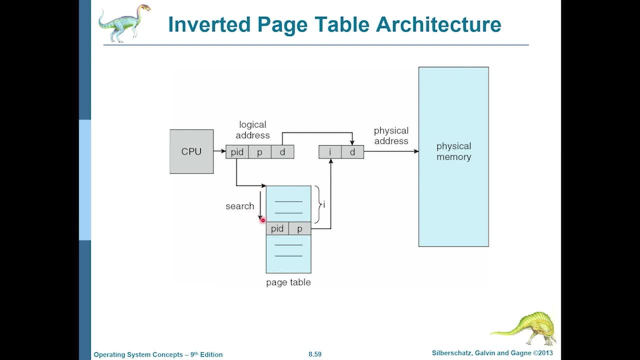 indexed by the physical frame number. indexed by the physical frame number. that is why it is inverted, so you might. that is why it is inverted, so you might. that is why it is inverted, so you might. ask this: linear searching can take a lot. ask this: linear searching can take a lot. 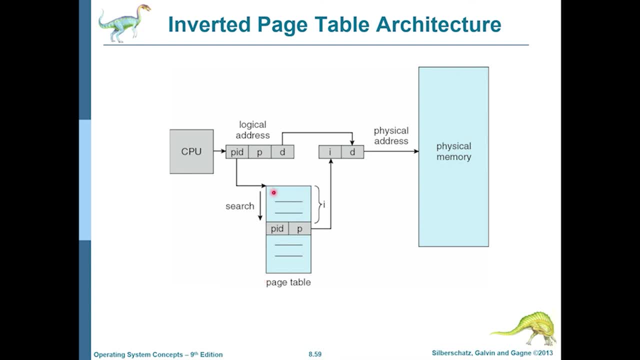 ask this: linear searching can take a lot of time because you have to first look of time. because you have to first look of time, because you have to first look at the first entry and say, okay, does at the first entry. and say, okay, does at the first entry and say, okay, does this entry even belong to this process? 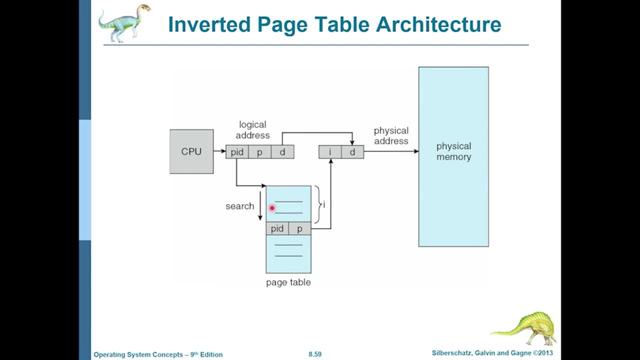 this entry even belong to this process. this entry even belong to this process, no, okay, let's go to the next one, okay, no, okay, let's go to the next one, okay, no, okay, let's go to the next one. okay, this entry belongs to this process, but. 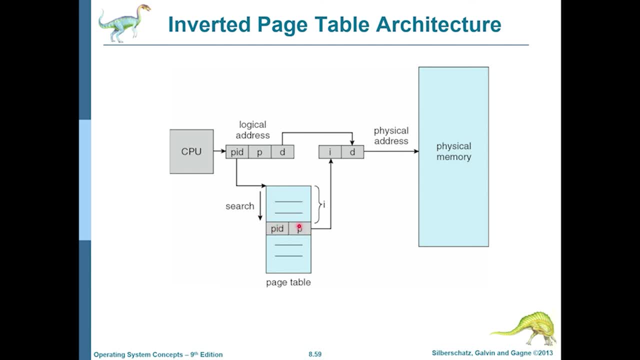 this entry belongs to this process. but this entry belongs to this process. but is this the page number? no, the pid. is this the page number? no, the pid. is this the page number? no, the pid. matched, but the page number did not match. matched, but the page number did not match. 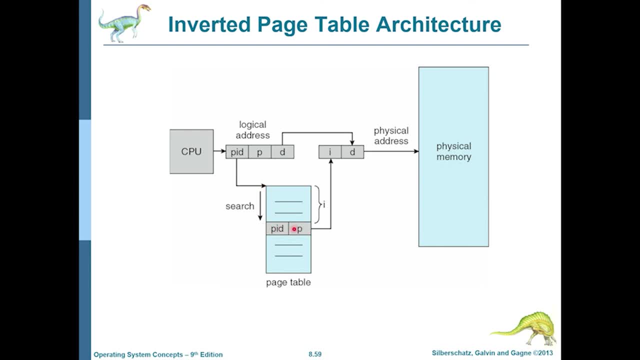 matched, but the page number did not match. so you keep going like that until you. so you keep going like that until you. so you keep going like that until you find your pid p combination somewhere, find your pid p combination somewhere, find your pid p combination somewhere, and then you find: how far have you gone? 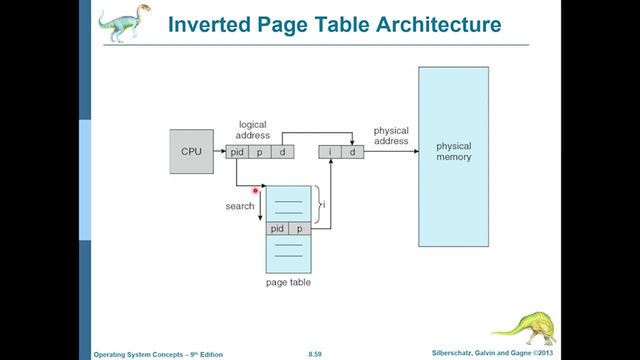 and then you find how far have you gone, and then you find how far have you gone and that is your and that is your and that is your frame number i. so we can use tlbs to frame number i. so we can use tlbs to frame number i. so we can use tlbs to accelerate this process, because 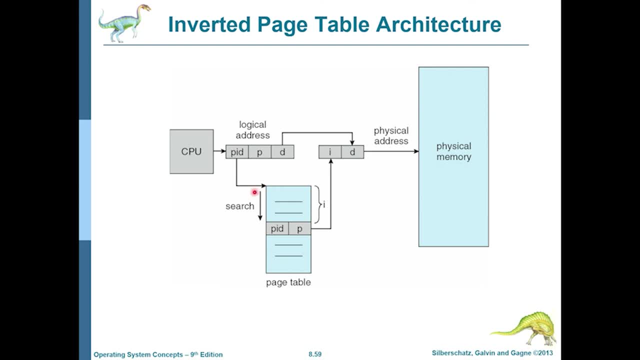 accelerate this process because accelerate this process? because translation: look aside buffers. use translation. look aside buffers. use translation. look aside buffers, use associative memory and in associative associative memory and in associative associative memory and in associative memory. you can do a parallel memory, you can do a parallel memory, you can do a parallel search. you can look at all the entries. 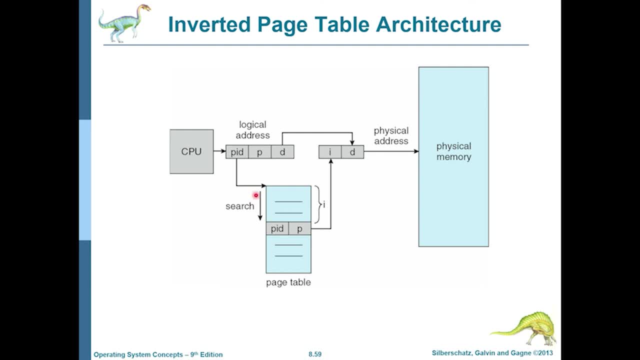 search you can look at all the entries. search. you can look at all the entries at the same time, parallelly, at the same time, parallelly, at the same time, parallelly, simultaneously, and you don't have to do simultaneously, and you don't have to do simultaneously, and you don't have to do a linear search, such kinds of searches. 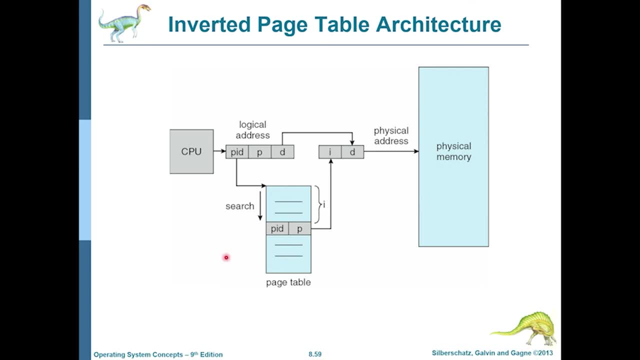 a linear search, such kinds of searches, a linear search, such kinds of searches are very, very cheap. time wise, now let's quickly look at the intel 32. now let's quickly look at the intel 32. now let's quickly look at the intel 32 and 64-bit architectures. we will also 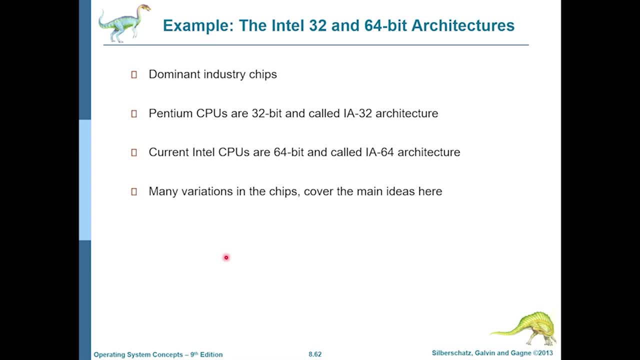 and 64-bit architectures. we will also and 64-bit architectures. we will also. give a brief glimpse at the arm. give a brief glimpse at the arm. give a brief glimpse at the arm. architecture- before concluding this architecture, before concluding this architecture, before concluding this chapter, as you all know, intel chips have. 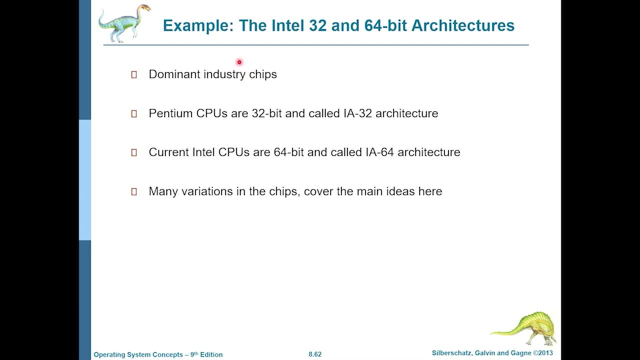 chapter. as you all know, intel chips have chapter. as you all know, intel chips have been the dominant industry chips for been the dominant industry chips for been the dominant industry chips for many decades now, many decades now, many decades now. pentium cpus are 32-bit and are called. 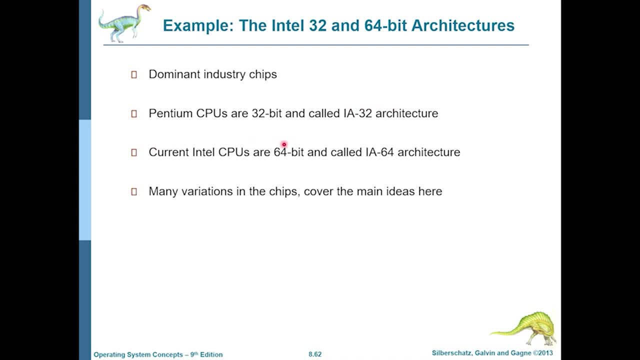 pentium cpus are 32-bit and are called pentium cpus are 32-bit and are called ia32 architecture. the current intel cpus: ia32 architecture. the current intel cpus: ia32 architecture. the current intel cpus are 64-bit and they are called the ia64. 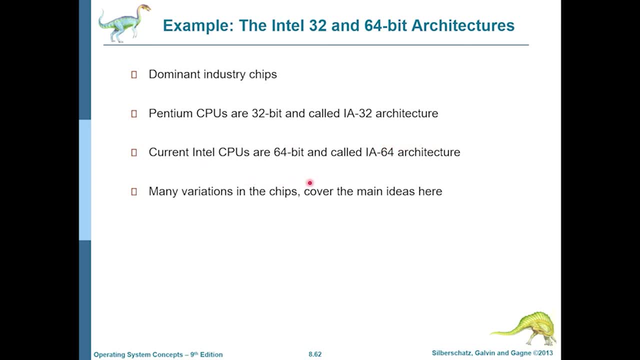 are 64-bit and they are called the ia64 are 64-bit and they are called the ia64. architecture, architecture, architecture. many variations in the chips. are there? many variations in the chips. are there? many variations in the chips are there. we will just cover the main ideas over. 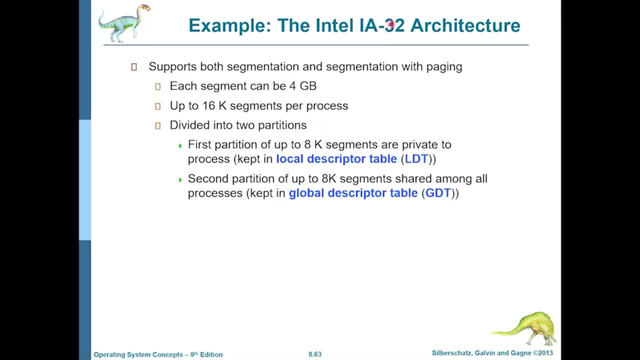 we will just cover the main ideas over. we will just cover the main ideas over paging. so you can either use only paging. so you can either use only paging. so you can either use only segmentation, or you can choose to use segmentation, or you can choose to use 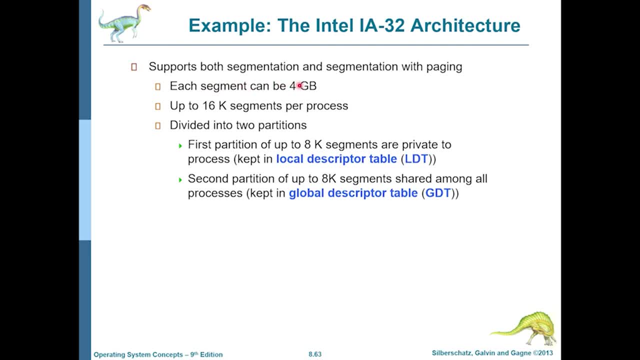 segmentation, or you can choose to use segmentation with paging, segmentation with paging, segmentation with paging. each segment can be 4 gb big. each segment can be 4 gb big. each segment can be 4 gb big. you can have up to 16 k segments per. you can have up to 16 k segments per. 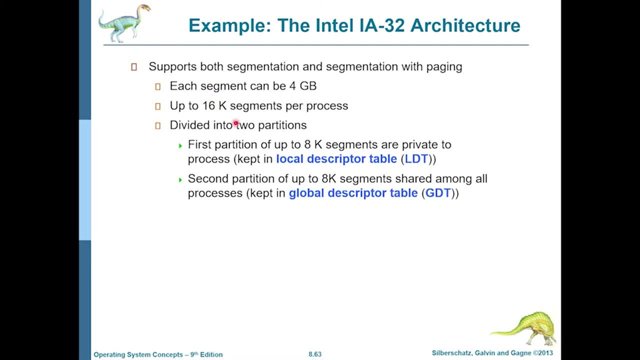 you can have up to 16 k segments per process, and these 16k segments are process. and these 16k segments are process, and these 16k segments are divided into two parts. divided into two parts. divided into two parts. one partition is described by the local 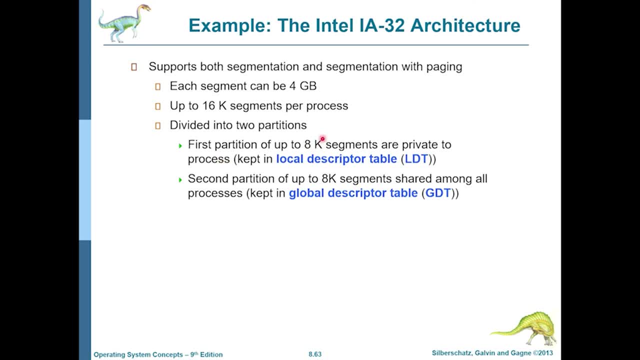 one partition is described by the local. one partition is described by the local descriptor table and these are private descriptor table and these are private descriptor table and these are private to the process and you can have 8k to the process and you can have 8k. 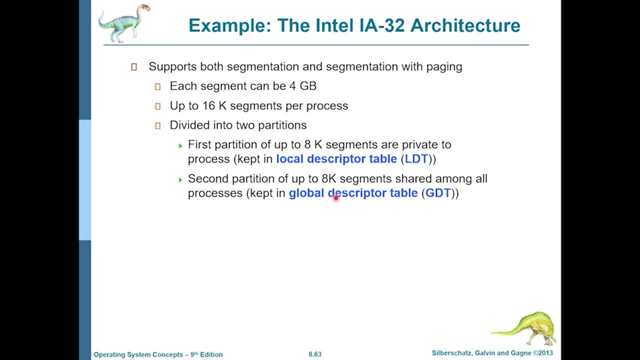 to the process and you can have 8k segments like that, segments like that, segments like that, and then the second partition is, and then the second partition is, and then the second partition is described by the global descriptor, described by the global descriptor, described by the global descriptor table, that is gdt, and you can have 8k. 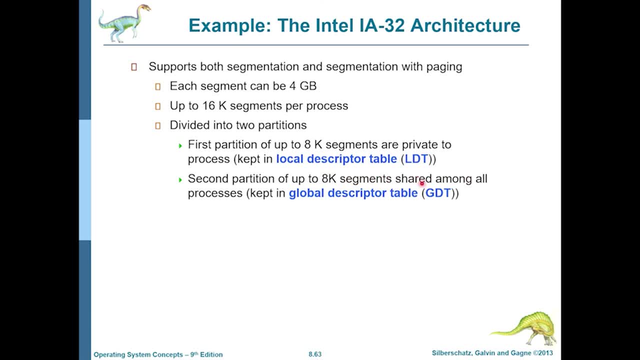 table that is gdt and you can have 8k table that is gdt and you can have 8k segments that way and these 8k segments segments that way and these 8k segments segments that way, and these 8k segments are shared among all the processes. 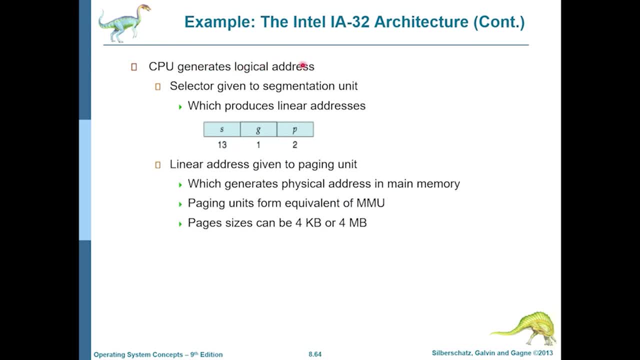 the cpu generates logical addresses. as the cpu generates logical addresses. as the cpu generates logical addresses as always, always, always, and, and, and. they are fed to the segmentation unit. they are fed to the segmentation unit. they are fed to the segmentation unit because the segmentation unit gets an. 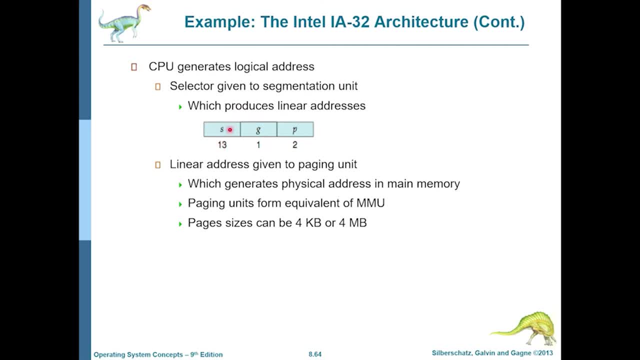 because the segmentation unit gets an, because the segmentation unit gets an address like this, so there is a segment address like this, so there is a segment address like this, so there is a segment selector, which is basically the segment selector, which is basically the segment selector, which is basically the segment number that takes. 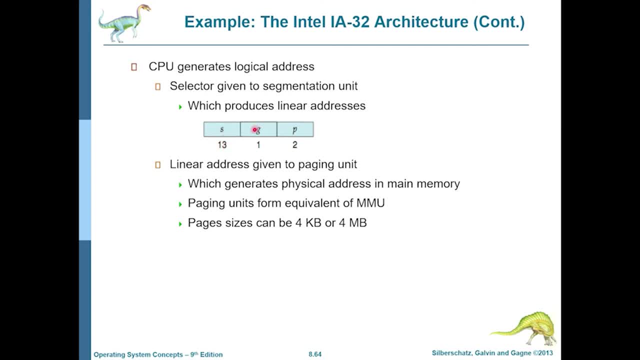 number that takes number that takes 13 bits. and then there is a g bit which 13 bits. and then there is a g bit which 13 bits, and then there is a g bit which basically tells you whether it should go. basically tells you whether it should go. 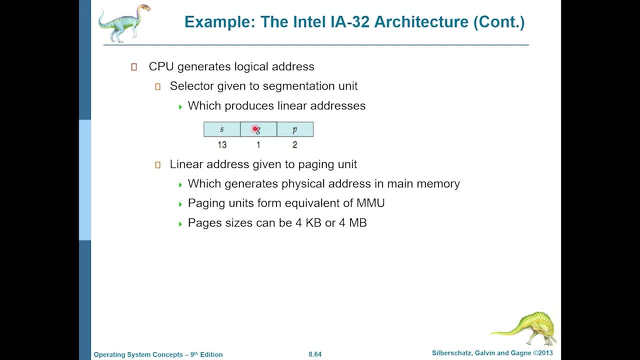 basically tells you whether it should go to the gdt- the global descriptor table, to the gdt- the global descriptor table, to the gdt- the global descriptor table, or the ldt- the local descriptor table, or the ldt- the local descriptor table. as we saw, there are 8k. 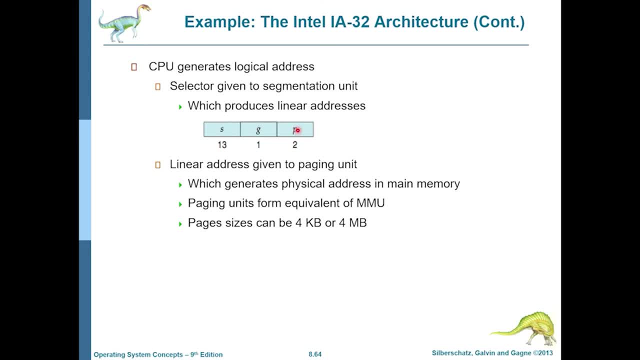 as we saw, there are 8k. as we saw, there are 8k, each in each of those tables, and then each in each of those tables, and then each in each of those tables, and then this p is used for protection. this p is used for protection. 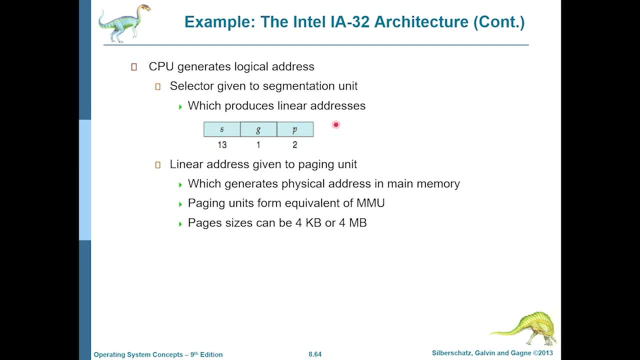 this p is used for protection- then whatever comes out of the, then whatever comes out of the, then whatever comes out of the segmentation unit- whatever address, we segmentation unit. whatever address, we segmentation unit. whatever address we get, we call that the linear address and get, we call that the linear address. and 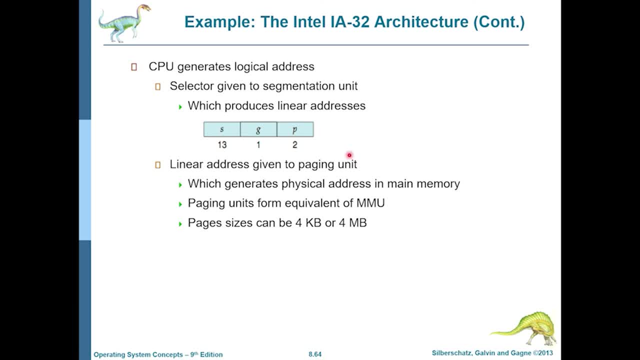 get. we call that the linear address, and then that address can go into the paging, then that address can go into the paging, then that address can go into the paging unit, unit, unit, and the linear address is converted to and the linear address is converted to and the linear address is converted to a physical address inside the paging. 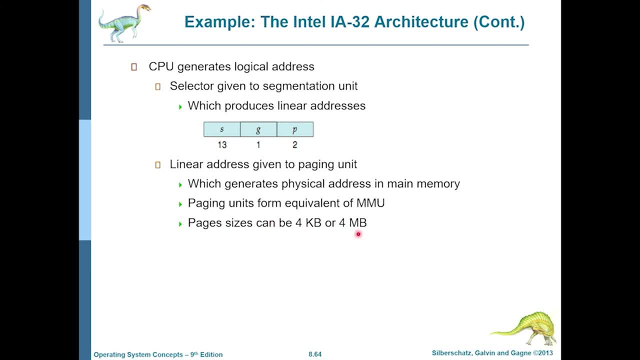 a physical address inside the paging. a physical address inside the paging unit and the page sizes can be 4 kb or 4 unit and the page sizes can be 4 kb or 4 unit and the page sizes can be 4 kb or 4 mb in the intel ia32 architecture. 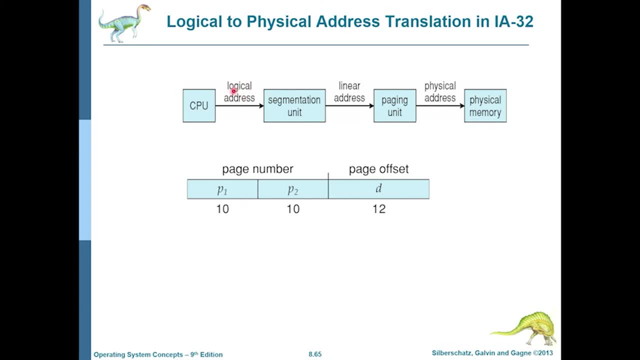 mb in the intel ia32 architecture. mb in the intel ia32 architecture. so this is how it goes. the cpu generates. so this is how it goes. the cpu generates. so this is how it goes. the cpu generates logical addresses. they go into the logical addresses. they go into the. 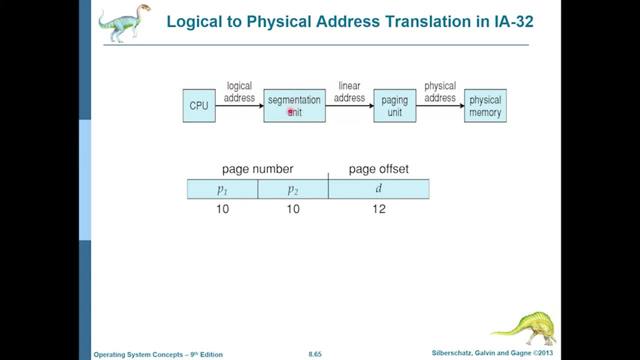 logical addresses. they go into the segmentation unit. so the segmentation segmentation unit, so the segmentation segmentation unit. so the segmentation unit will look at the base address of the unit, will look at the base address of the unit, will look at the base address of the segment number that you have chosen. 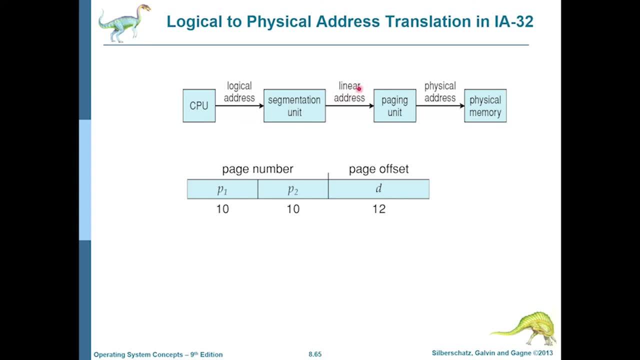 segment number that you have chosen, segment number that you have chosen, then it will add the offset to it to give. then it will add the offset to it to give. then it will add the offset to it to give you a linear address. and we have seen you a linear address and we have seen 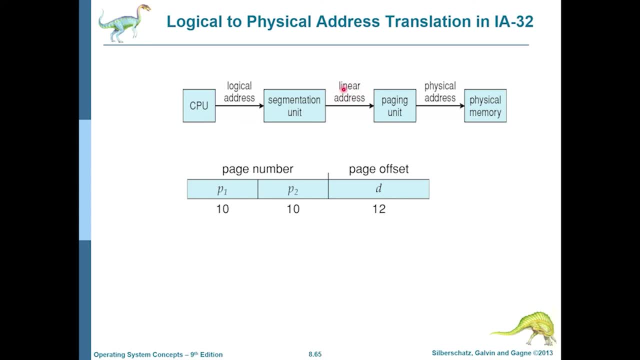 you a linear address and we have seen how this works in the segmentation, how this works in the segmentation, how this works in the segmentation. slides before slides, before slides, before the linear address is then given to the. the linear address is then given to the. the linear address is then given to the paging unit. it will look at. 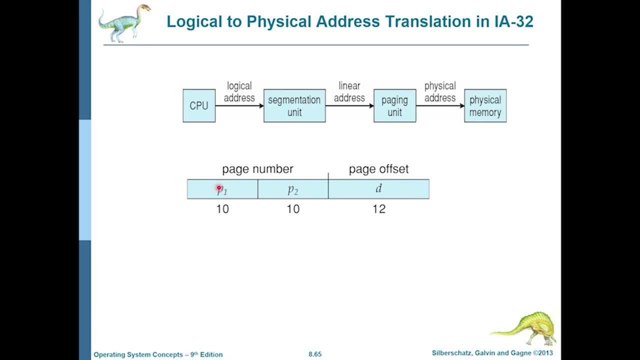 paging unit. it will look at paging unit. it will look at the linear address in this format. so it the linear address in this format. so it the linear address in this format. so it will think of these 10 bits as the outer, will think of these 10 bits as the outer. 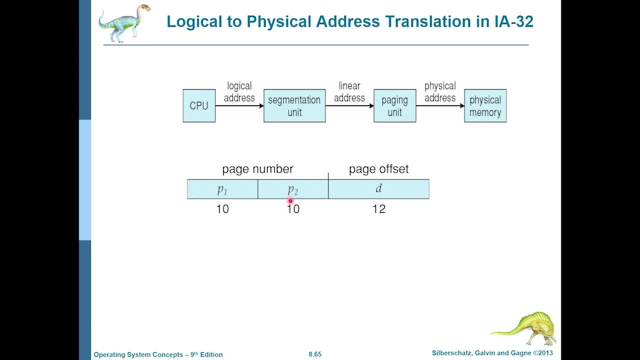 will think of these 10 bits as the outer page table, these 10 bits as belonging page table, these 10 bits as belonging page table, these 10 bits as belonging to the inner page table and 12 bits for to the inner page table and 12 bits for. 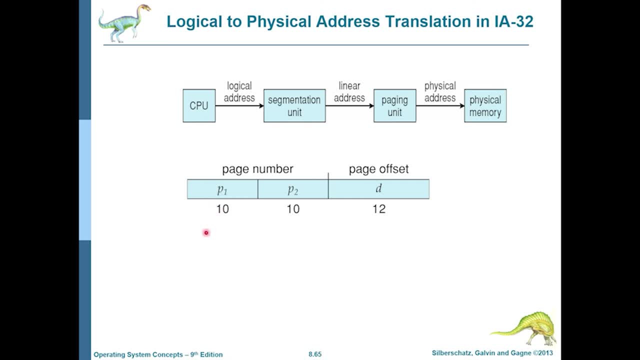 to the inner page table and 12 bits for the offset. so it will use these 10 bits the offset. so it will use these 10 bits the offset. so it will use these 10 bits to index into the outer page table. then to index into the outer page table then. 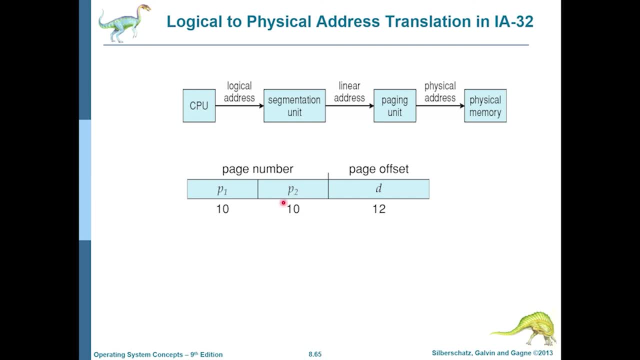 to index into the outer page table. then, whenever it finds the base address of, whenever it finds the base address of, whenever it finds the base address of the inner page table, it will use these. the inner page table. it will use these. the inner page table. it will use these 10 bits to index into that page table. 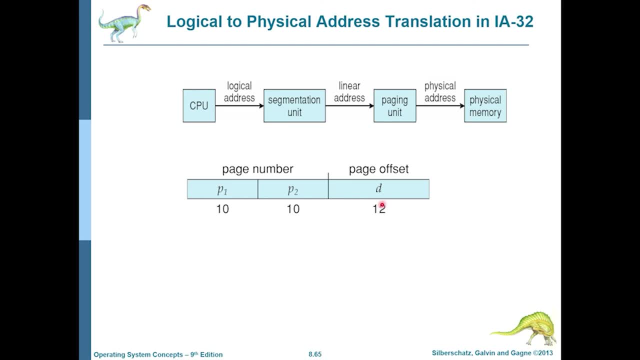 10 bits to index into that page table. 10 bits to index into that page table the inner page table. then once it has the inner page table, then once it has the inner page table, then once it has found the real page table, entry for the. found the real page table. entry for the. 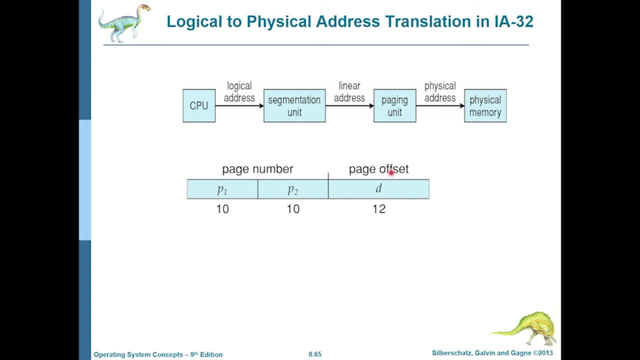 found the real page table entry for the page. it will figure out the base address page. it will figure out the base address page. it will figure out the base address of the frame. then it will use the 12 of the frame. then it will use the 12. 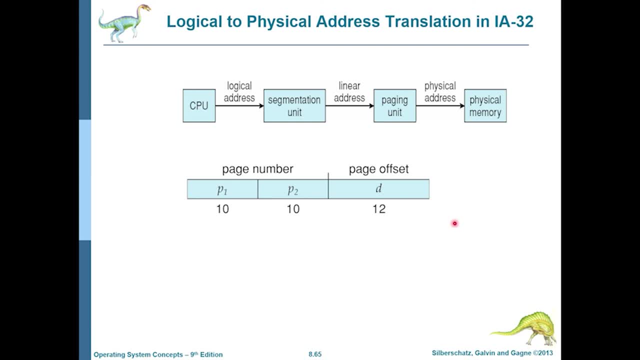 of the frame. then it will use the 12 bits over here to figure out how far bits over here, to figure out how far bits over here to figure out how far into the frame the physical memory, into the frame, the physical memory, into the frame, the physical memory location is, and then it will generate. 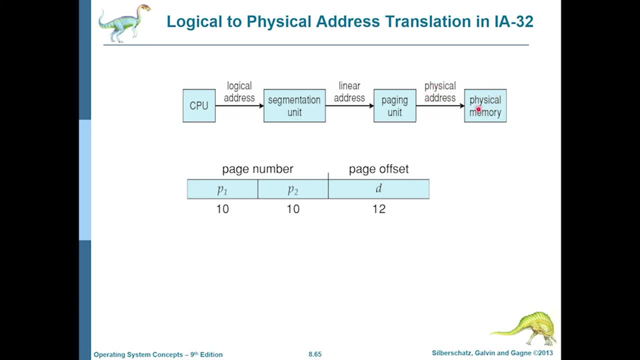 location is and then it will generate location is and then it will generate the physical address. that will go into the physical address. that will go into the physical address, that will go into the physical memory and we can read: or the physical memory and we can read, or 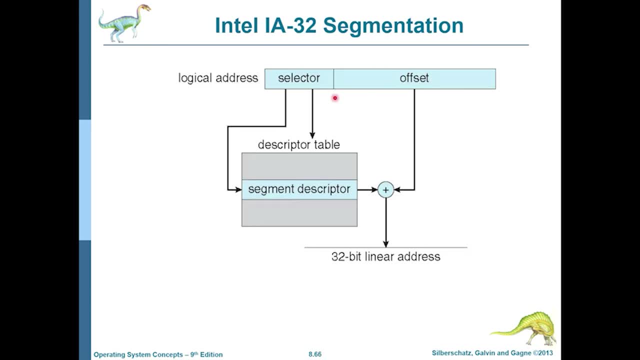 the physical memory and we can read or write to that physical memory. write to that physical memory, write to that physical memory. here is a bigger picture of the. here is a bigger picture of the. here is a bigger picture of the segmentation unit and, as i said before, 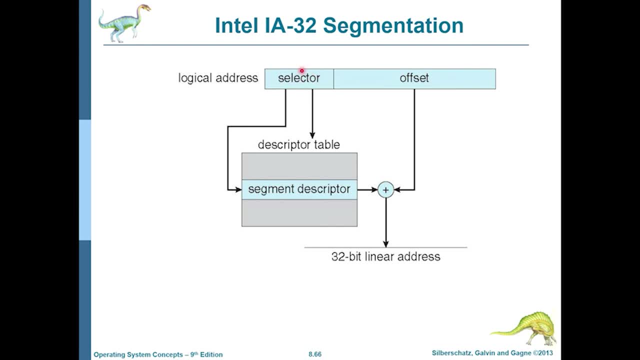 segmentation unit and, as i said before, segmentation unit and, as i said before, the selector has the segment number. the selector has the segment number. the selector has the segment number. either it is gdt or ldt and there is a. either it is gdt or ldt and there is a. 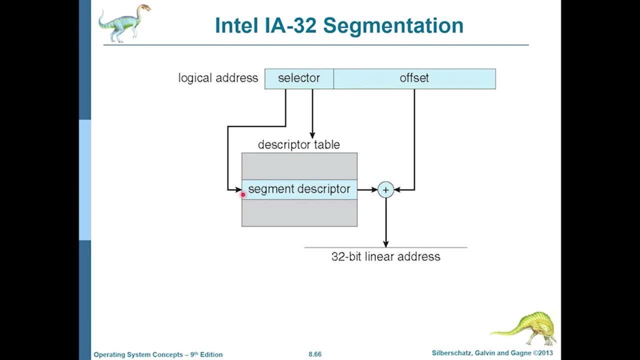 either it is gdt or ldt and there is a couple of bits for protection. so we look couple of bits for protection. so we look couple of bits for protection. so we look at a descriptor table and we use the. at a descriptor table and we use the. 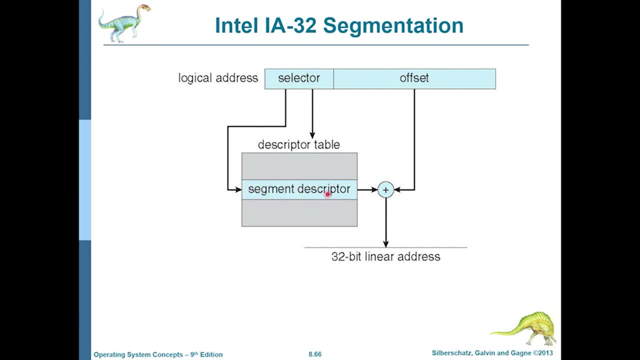 at a descriptor table and we use the segment number to kind of index into segment number, to kind of index into segment number, to kind of index into that and figure out that, and figure out that, and figure out which segment it is and find its segment, which segment it is and find its segment. 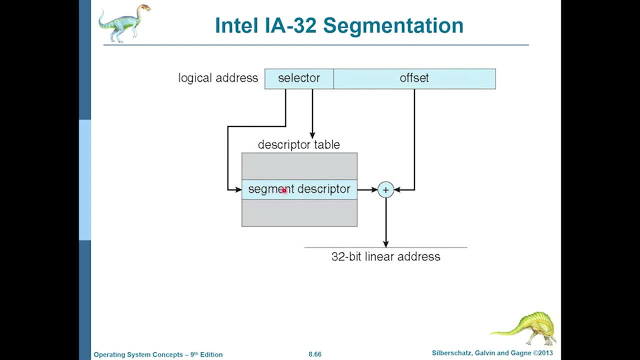 which segment it is and find its segment descriptor. the segment descriptor will descriptor. the segment descriptor will descriptor. the segment descriptor will give us the base address of the segment. give us the base address of the segment. give us the base address of the segment. we take the offset, we add them and we 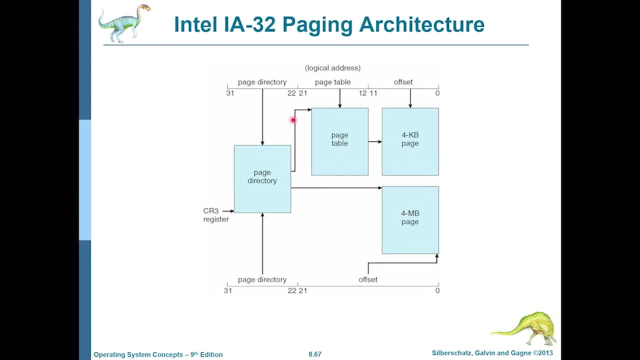 we take the offset, we add them and we we take the offset, we add them and we get a 32-bit linear address over here. get a 32-bit linear address over here. get a 32-bit linear address over here. and this is the paging structure. so here. 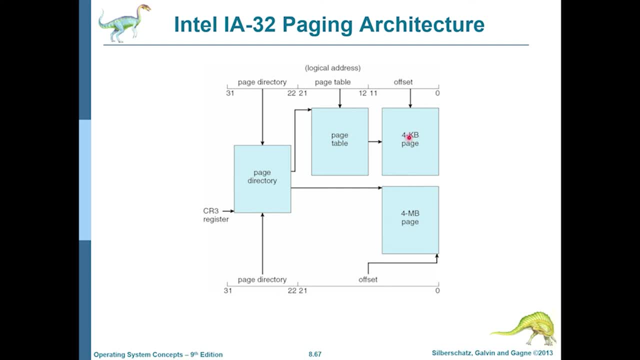 and this is the paging structure. so here, and this is the paging structure, so here we use two levels of paging for smaller. we use two levels of paging for smaller. we use two levels of paging for smaller pages because smaller pages can have pages, because smaller pages can have. 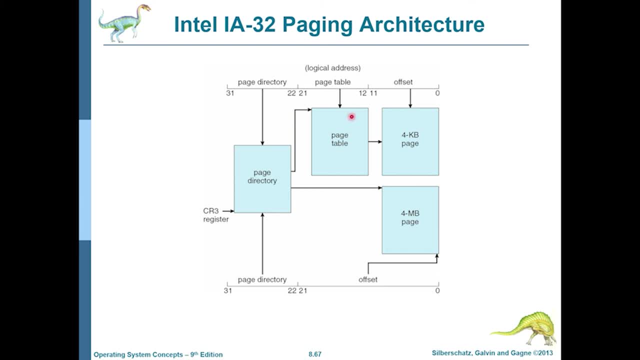 pages, because smaller pages can have lots of page table entries. so we need lots of page table entries. so we need lots of page table entries. so we need two levels over here and we will look at two levels over here. and we will look at two levels over here and we will look at later what happens for 4mb pages. just a. 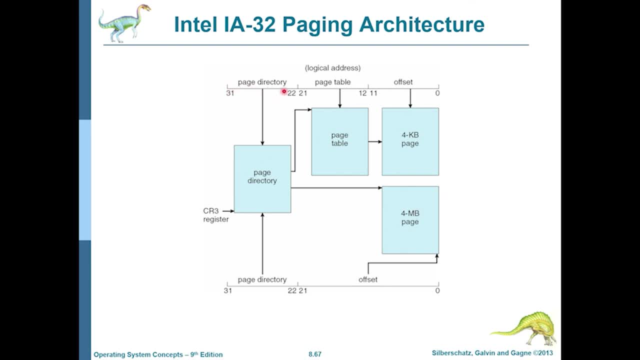 later what happens for 4mb pages. just a later: what happens for 4mb pages just a little bit after this little bit, after this little bit after this. so we use the 10 bits over here. so we use the 10 bits over here. so we use the 10 bits over here to index into the page directory. right, 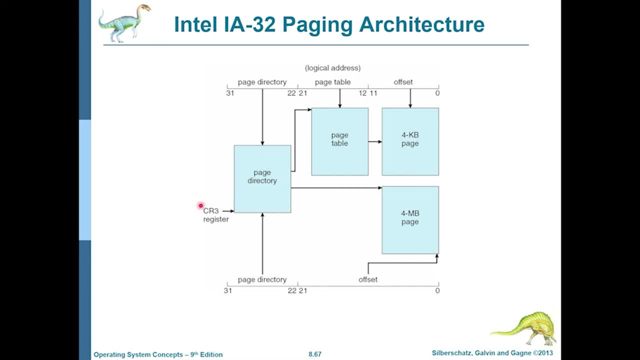 to index into the page directory: right. to index into the page directory: right. so the page directory is stored. so the page directory is stored. so the page directory is stored somewhere in memory, somewhere in memory, somewhere in memory. and and and the cr3 register in ia32 actually points. 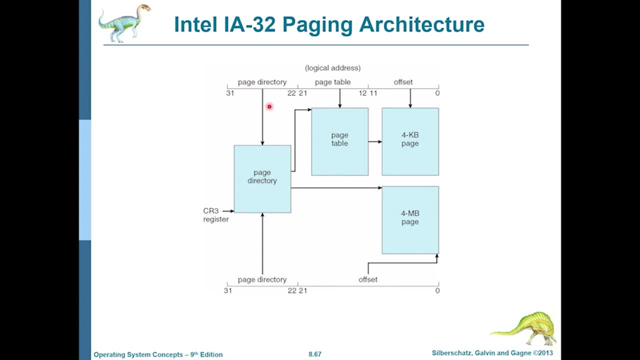 the cr3 register in ia32 actually points. the cr3 register in ia32 actually points to the base of the page directory. so we to the base of the page directory. so we to the base of the page directory. so we use the n bits of the logical address. 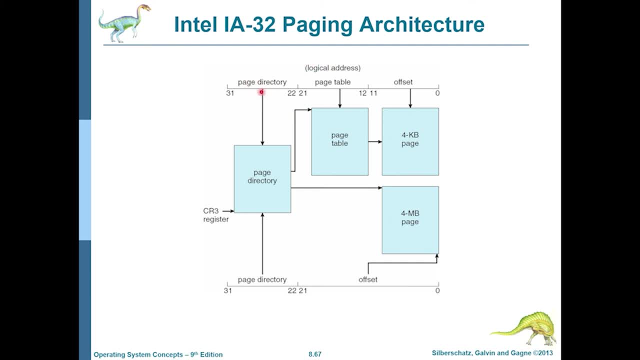 use the n bits of the logical address. use the n bits of the logical address over here, or the linear address which over here, or the linear address which over here, or the linear address which the segmentation unit gives us to index. the segmentation unit gives us to index. 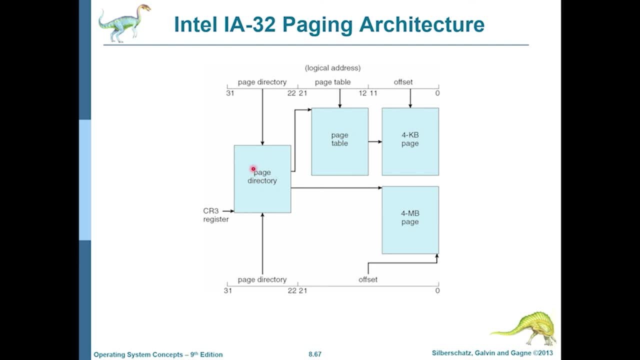 the segmentation unit gives us to index into the page directory, or you can also into the page directory, or you can also into the page directory, or you can also call this the outer page table and then call this the outer page table and then call this the outer page table and then, when we find the base address of the 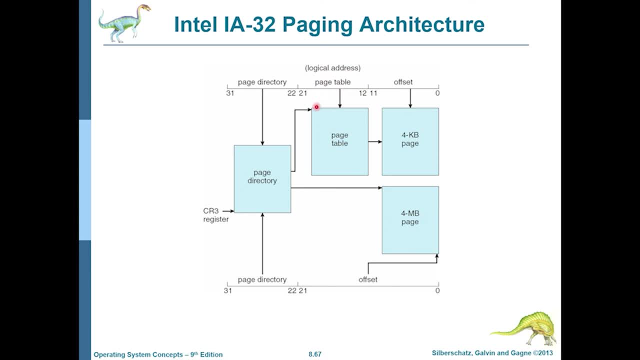 when we find the base address of the, when we find the base address of the page table, we go there, then we use these page table. we go there, then we use these page table. we go there, then we use these 10 bits over here which are allocated: 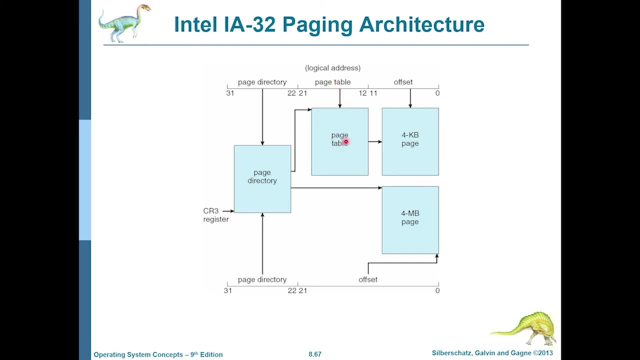 10 bits over here which are allocated, 10 bits over here which are allocated for the inner page table. then we index for the inner page table, then we index for the inner page table, then we index into the inner page table over here, into the inner page table over here. 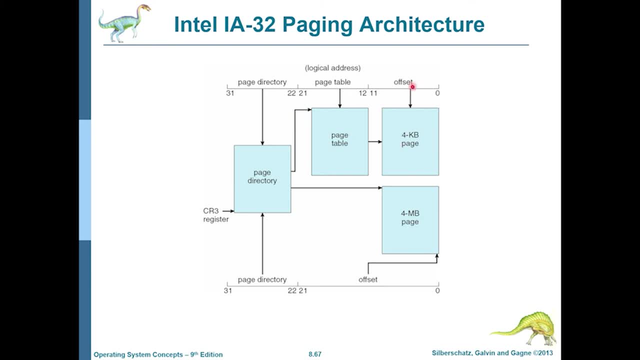 into the inner page table over here. then we get the base address of a page. then we get the base address of a page. then we get the base address of a page. then we use the offset to index into the. then we use the offset to index into the. 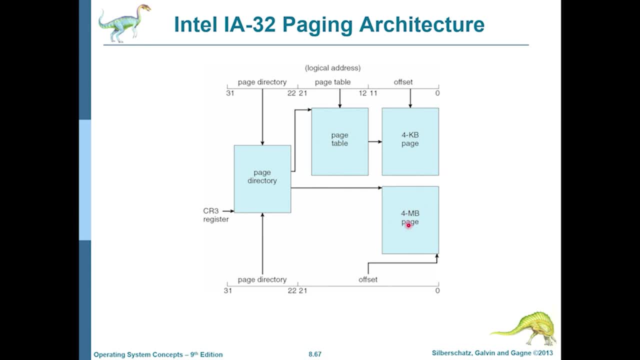 then we use the offset to index into the page and we find our memory location page and we find our memory location page and we find our memory location. but if four megabyte pages are being but if four megabyte pages are being, but if four megabyte pages are being used, then we don't need two levels of 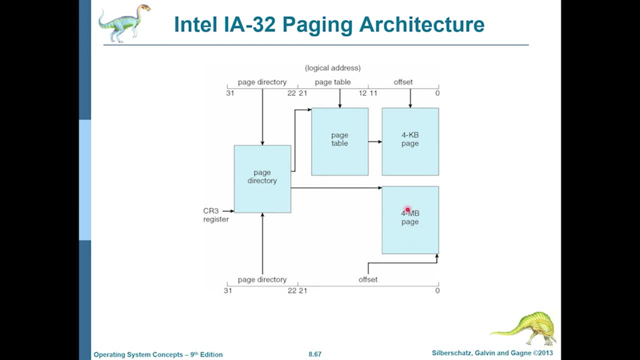 used, then we don't need two levels of used, then we don't need two levels of page tables, because only a very few page tables, because only a very few page tables, because only a very few pages like these would be there, so we. pages like these would be there, so we. 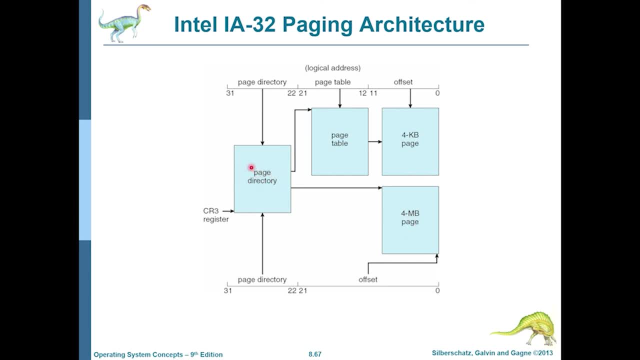 pages like these would be there. so we can just get away with using one level, can just get away with using one level, can just get away with using one level of page tables and we can just use the of page tables and we can just use the of page tables and we can just use the page directory over here, the outer page. 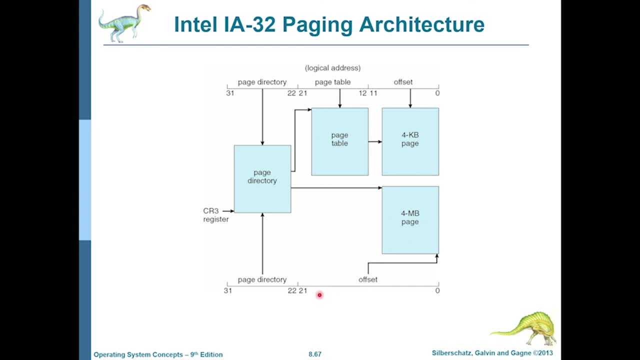 page directory over here. the outer page page directory over here. the outer page table is just enough. so since the offset table is just enough, so since the offset table is just enough, so since the offset is now bigger for four megabyte pages is now bigger for four megabyte pages. 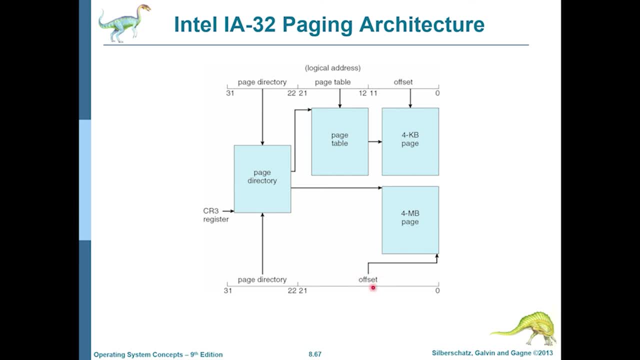 is now bigger for four megabyte pages because the pages are bigger. you need a because the pages are bigger. you need a because the pages are bigger. you need a larger offset. so the number of bits, that larger offset, so the number of bits, that larger offset, so the number of bits that are used for the page number have now. 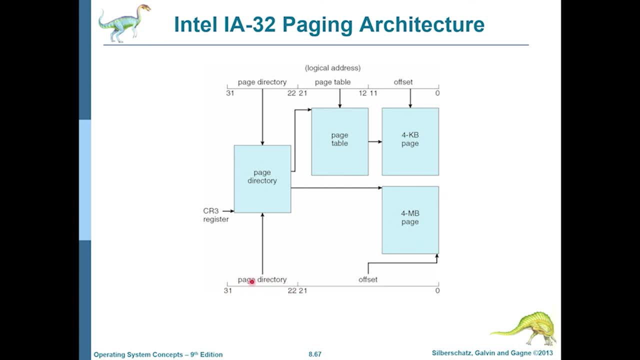 are used for the page number have now are used for the page number have now decreased, so we just need 10 bits for decreased. so we just need 10 bits for decreased. so we just need 10 bits for the page number and the rest of it is. 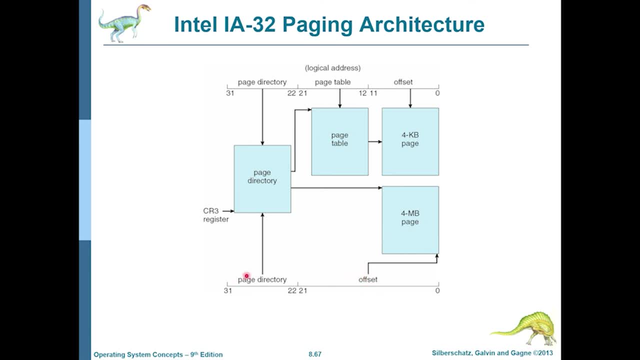 the page number and the rest of it is just the offset into the four megabyte, just the offset into the four megabyte, just the offset into the four megabyte page. so we use these 10 bits to index page. so we use these 10 bits to index. 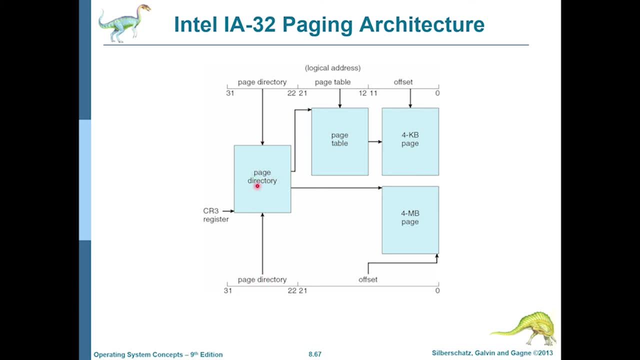 page. so we use these 10 bits to index into the page directory and whatever into the page directory and whatever into the page directory and whatever page table entry we find over here that page table entry we find over here, that page table entry we find over here. that will give us the base address of this. 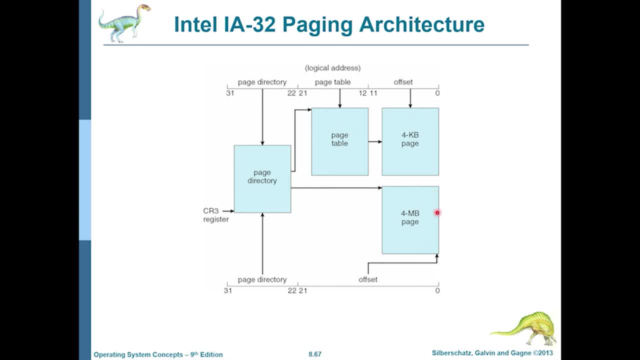 will give us the base address of this, will give us the base address of this four megabyte page and we can use this four megabyte page and we can use this four megabyte page and we can use this offset to offset into that page. offset to offset into that page. 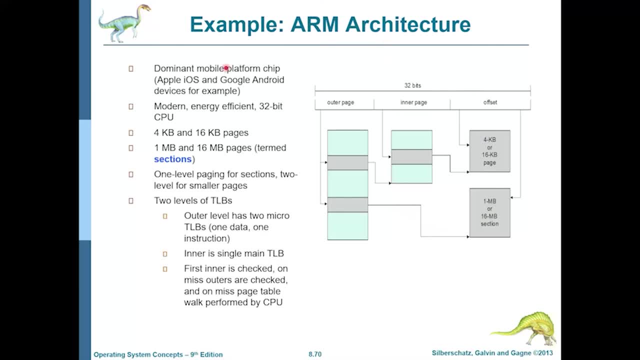 offset to offset into that page. and here we briefly look into the arm. and here we briefly look into the arm. and here we briefly look into the arm architecture. so arm is the dominant architecture, so arm is the dominant architecture. so arm is the dominant mobile platform chip. it is used by 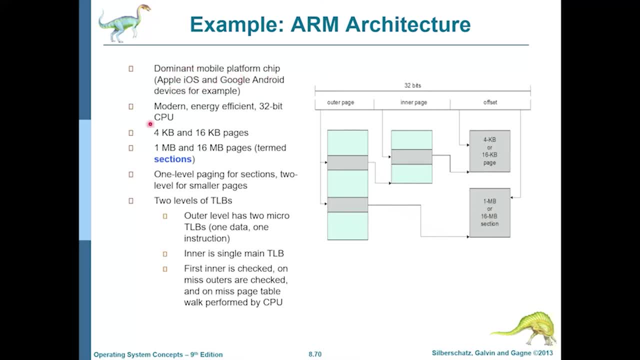 mobile platform chip. it is used by mobile platform chip. it is used by apple ios and google android and other apple ios and google android and other apple ios and google android and other devices, devices, devices. so it is very modern, it is very energy. so it is very modern, it is very energy. 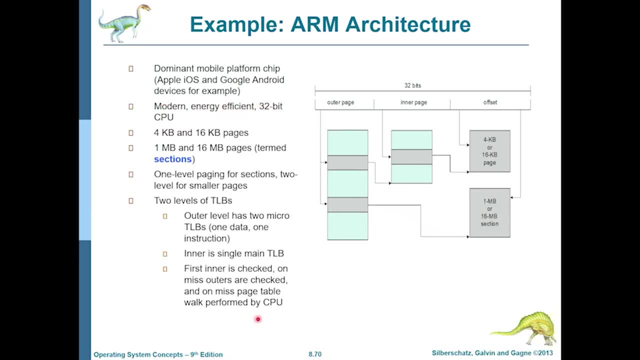 so it is very modern, it is very energy efficient and at the time when these efficient and at the time when these efficient and at the time when these slides were being prepared, that is 2013- slides were being prepared. that is 2013 slides were being prepared. that is 2013, only the 32-bit variant of these. 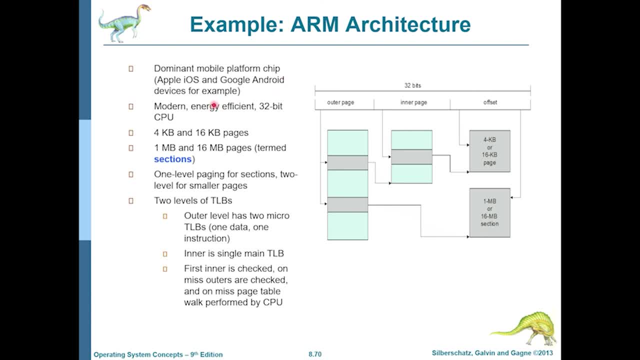 only the 32-bit variant of these. only the 32-bit variant of these chips were present. chips were present. chips were present when i am recording this video today, we, when i am recording this video today, we, when i am recording this video today, we 32-bit version of this chip. 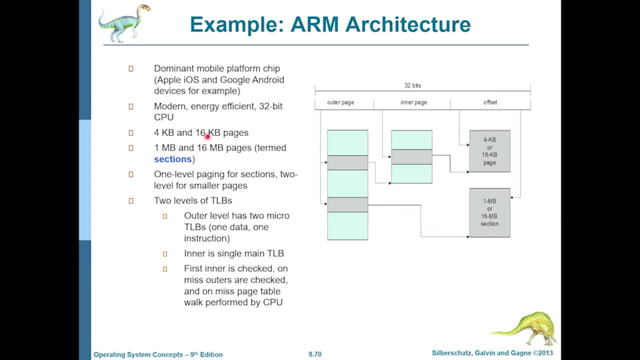 32-bit version of this chip. 32-bit version of this chip worked as far as paging is concerned. worked as far as paging is concerned. worked as far as paging is concerned. so the 32-bit versions of these cpus. so the 32-bit versions of these cpus. 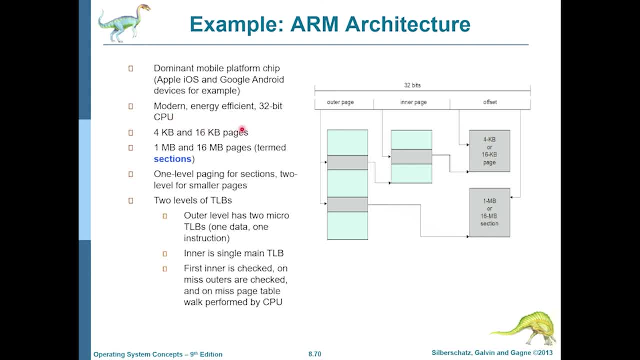 so the 32-bit versions of these cpus have have have both 4kb and 16 kb pages, both 4kb and 16 kb pages, both 4kb and 16 kb pages. they can also have 1 mb and 16 mb pages. they can also have 1 mb and 16 mb pages. they can also have 1 mb and 16 mb pages, and these are large pages and they are, and these are large pages and they are, and these are large pages and they are called as called as: 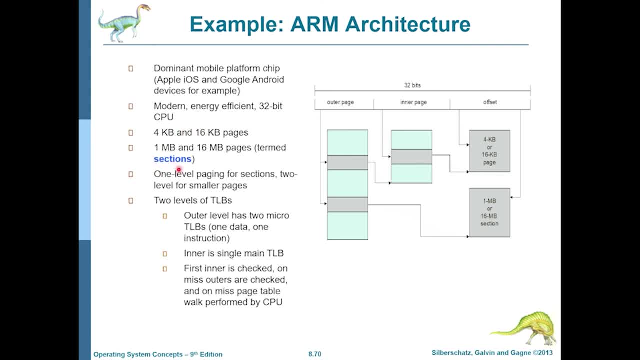 called as sections. so for this, small pages sections. so for this, small pages sections. so for this, small pages, we do two levels of paging, but for this we do two levels of paging. but for this we do two levels of paging. but for this, bigger pages, those are sections, we just 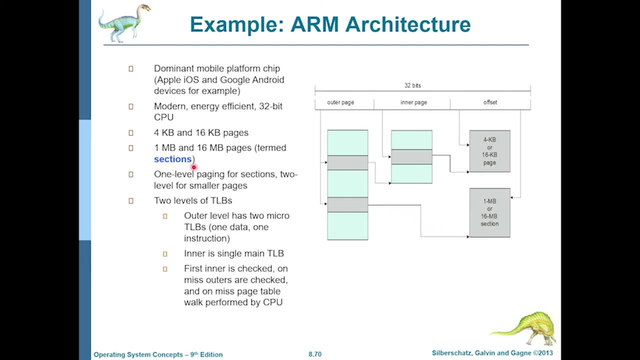 bigger pages. those are sections. we just bigger pages. those are sections. we just need one level of paging. this was also need one level of paging. this was also need one level of paging. this was also the case for intel when we used to use the case for intel, when we used to use.